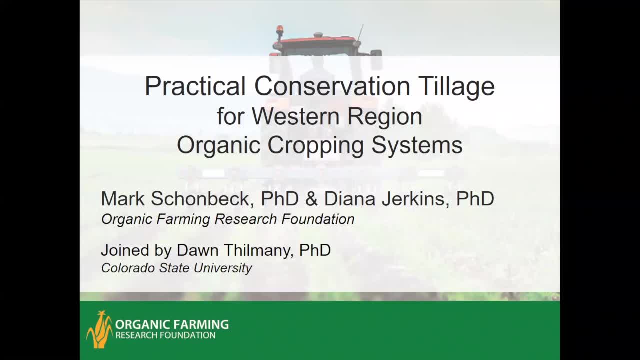 I'm your host, Alice Formiga of eOrganic. eOrganic has many articles, videos and webinars about organic farming and research, and you can find all of them on our website and on the eOrganic YouTube channel. We are recording this webinar and we will have the recording available on YouTube within one. 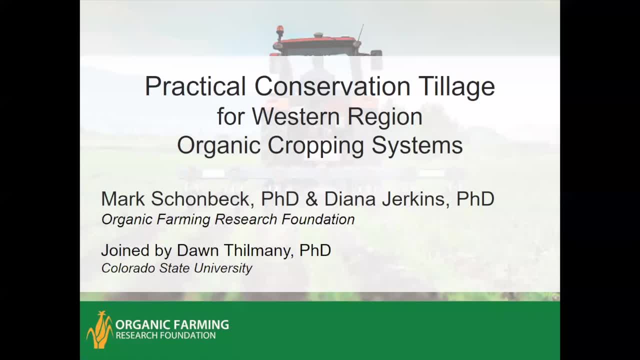 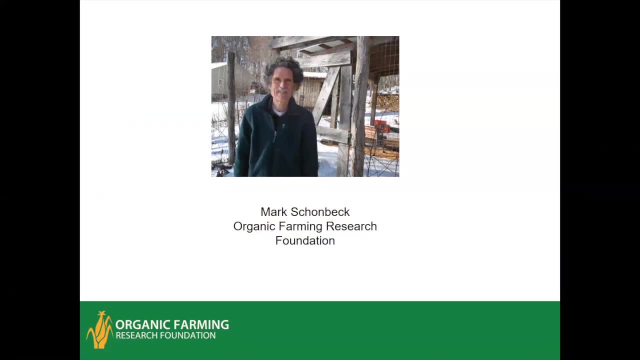 to two weeks. This webinar will be presented by Mark Schoenbeck, who is a research associate at the Organic Farming Research Foundation. Mark has worked for the last 31 years as a researcher, consultant and educator about organic farming and sustainable agriculture. He also 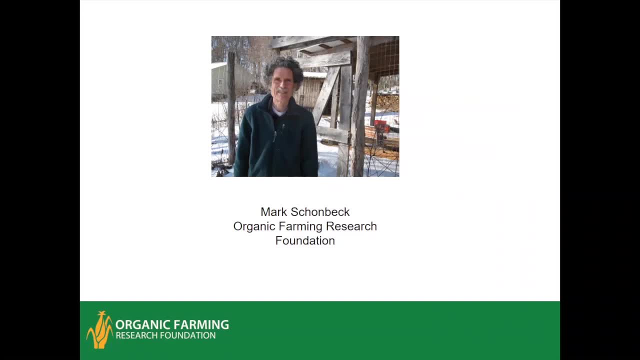 worked as a research consultant and educator about sustainable agriculture. He also worked with the Virginia Association for Biological Farming. We also have Dawn Telmani with us from Colorado State University and she is going to be online for the question and answer session. in case there is anything related to her area of expertise. She's a professor of agro-economics. 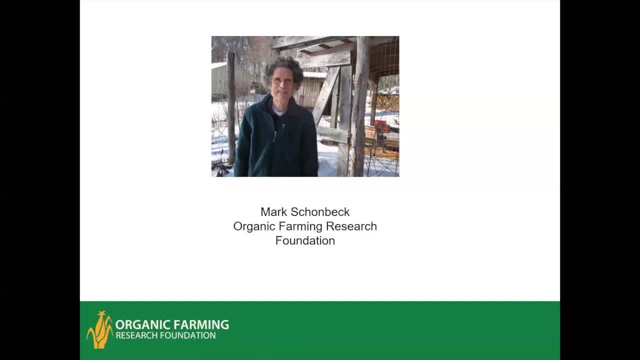 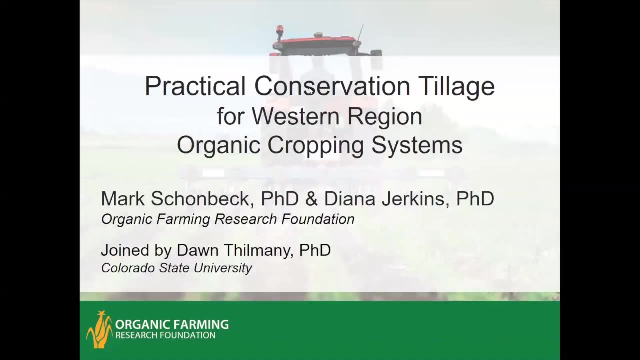 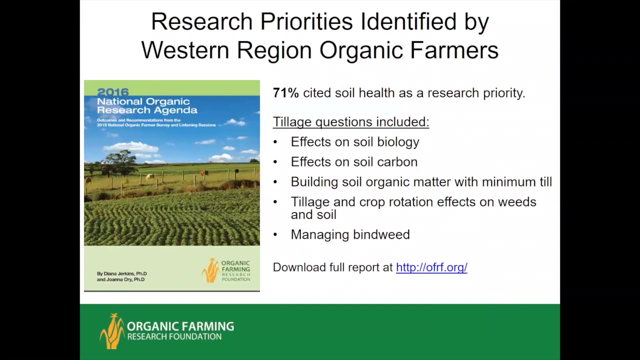 with Colorado State University and specializes in economic development related to local, organic and other value-added food market segments. So now, Mark, I am going to hand over the remote control to you. All right, thank you. So one of the first things I 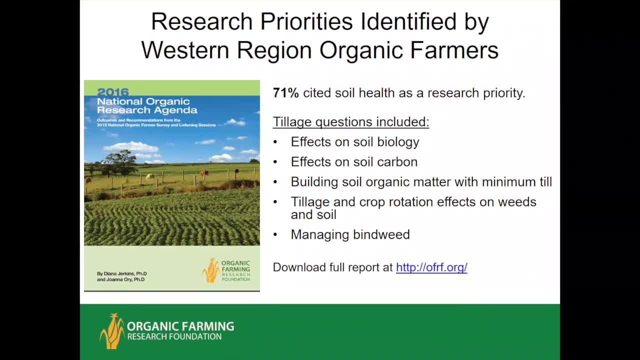 like to cover in these webinars is discuss the research priorities of western region organic farmers. This is based on a survey that the Organic Farming Research Foundation conducted during 2015 and published report in 2016, which became the National Organic Research Agenda. Not surprisingly, the largest percentage of farmers identified soil health. 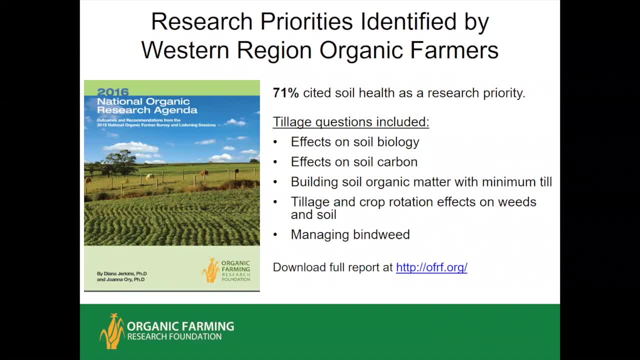 as a high research priority: 71 percent in the western region. This is based on 555 respondents and also a series of six listening sessions And, within the topic of healthy soils, which, of course, are the basis of organic farming, some of the questions related to tillage included. 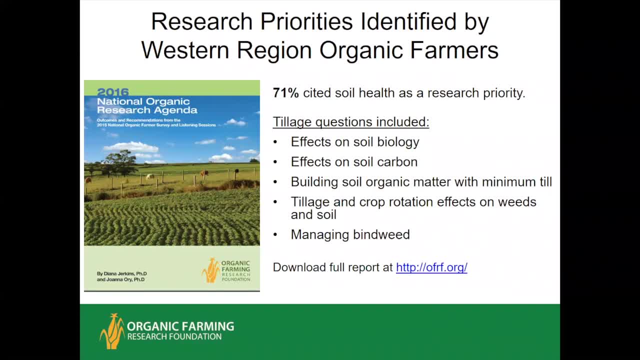 the effects on soil biology, soil life effects on soil carbon. how to build soil organic matter with minimum tillage. tillage and crop rotation. effects on the interaction between weeds and soils and crops. And then one weed continued to rear its ugly head: field bindweed, which I'm sure a lot of. 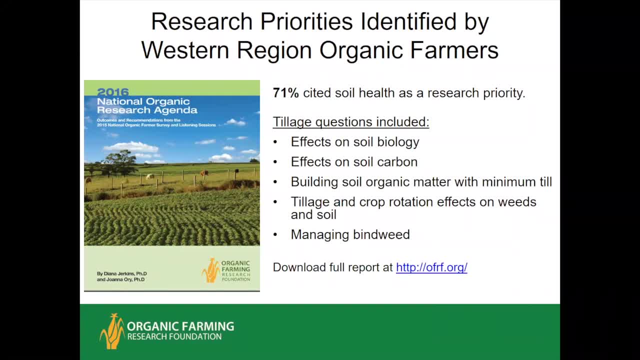 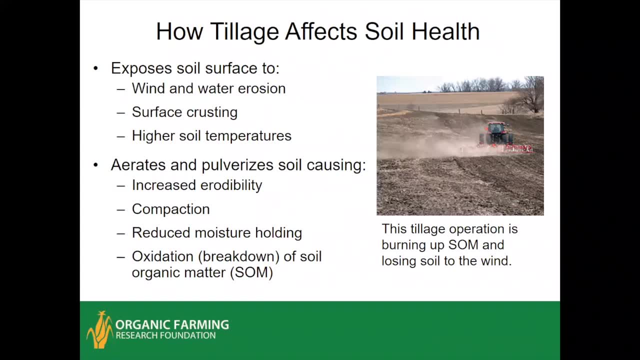 you are quite familiar with, more so than I am. So these are some of the topics that we'll try to cover during this session. Okay, well, how does tillage affect soil health? Well, here's how it affects the physical properties. If the soil is even somewhat dry, when you're out there with your 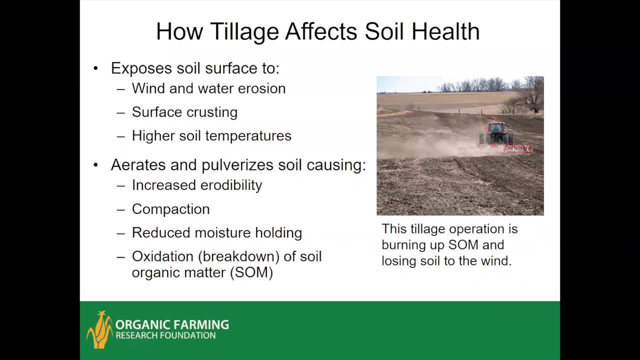 tillage implement and you're doing full width tillage, you're going to be losing some of the soil to the wind And also, stirring the soil surface exposes the organic matter to oxidation And, of course, even if this weren't happening during the tillage, the bare soil period afterwards subject to wind and water erosion. 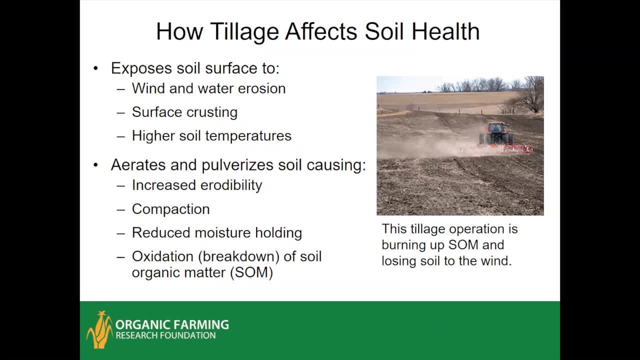 surface crusting. when rain falls on an uncovered surface, it tends to seal to a greater or lesser extent. It also increases soil temperatures, so that that top inch or so may become so hot as to be inhospitable to soil life, so that soil life will go dormant. 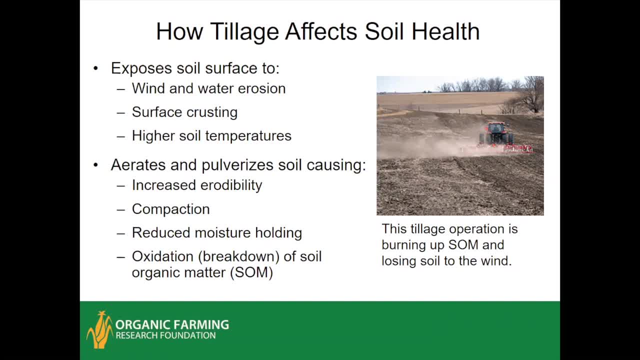 even partially, die out in that very surface area, part of the soil, And the aeration and the oxidation causes some other changes. By loosening the soil it is more subject to erosion and also compaction And you will reduce, have some loss of moisture holding capacity as well. 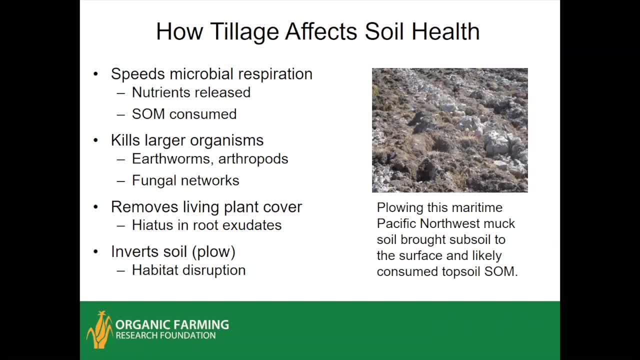 And this is how soil tillage affects biological properties. The tilling action stimulates certain microbes to increase their respiratory activity And, in fact, the ratio between what is called maintenance respiration- how much of the soil organic residues are simply turning into carbon dioxide, versus how much goes into growing new microbes. 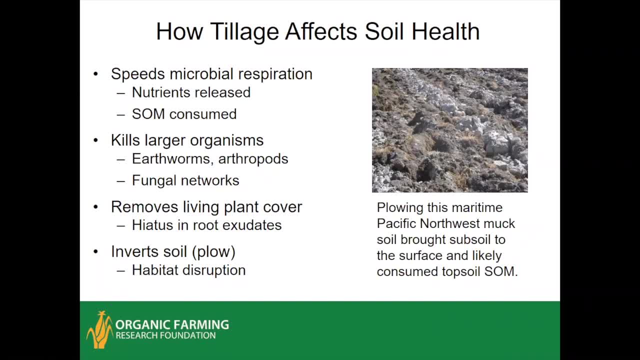 and new microbial residues. that is increased. This increases the release of nutrients- crop nutrients- But it also burns up the organic matter And, of course, the more intense the physical disturbance, the more you lose larger organisms like earthworms and the microarthropods. 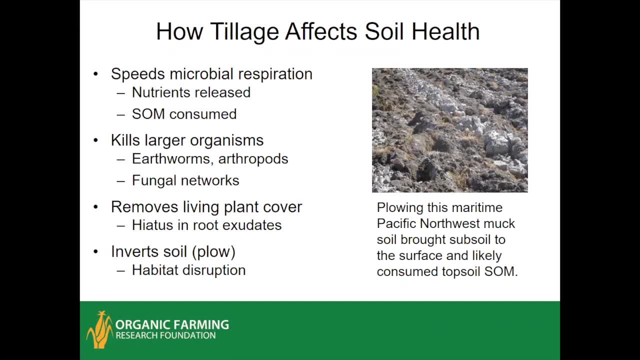 and also the fungal network, the fungal network, the fungal network that is used over time, and also the fungal network that is also the source of the networks. although fungi on an individual basis are microbes and that the filaments are very microscopic, the length and the extent of those networks can actually cover many. 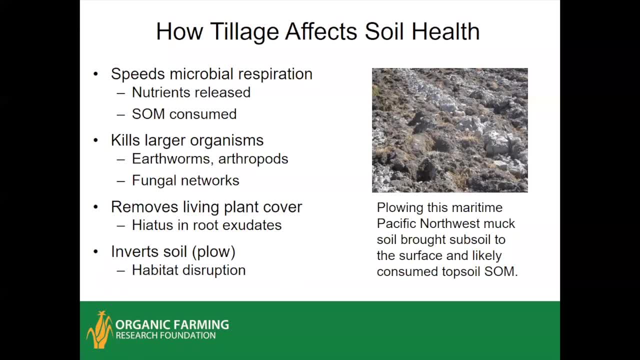 square feet, even an acre. So you're breaking up those networks. And then one other thing that happens is whenever you remove the living cover, the primary source of food for the soil, life is, at least temporarily cut off. As long as there's nothing growing, there's no root exudates and no root deposition going. 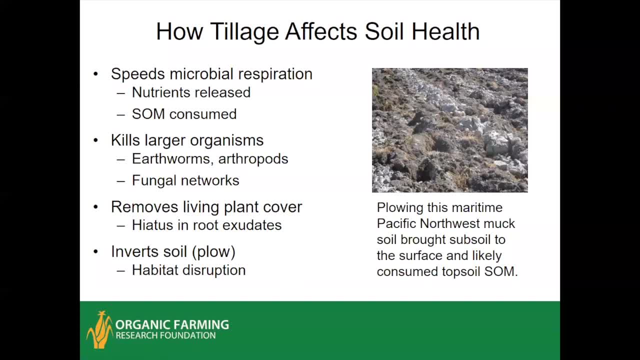 into the soil And that is like the staple in the diet of the soil life. So that creates a hiatus in that flow of nutrients to the soil food web And when you have inversion tillage that you see in this picture, this was on a muck soil. 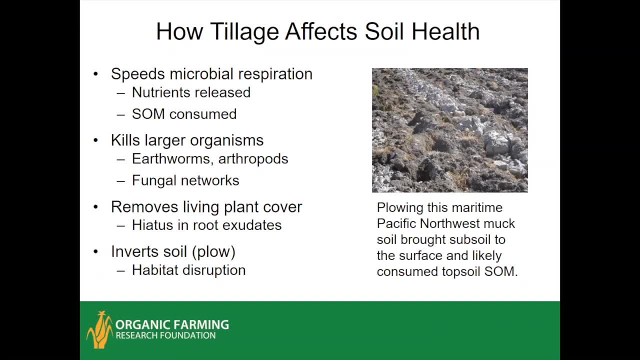 It was a fairly shallow depth down to the sandy subsoil And you can see what happened there when a plow was run through and it brought some of that subsoil to the surface And even if that doesn't occur visibly, you've disrupted habitat, broken up, earthworm burrows. 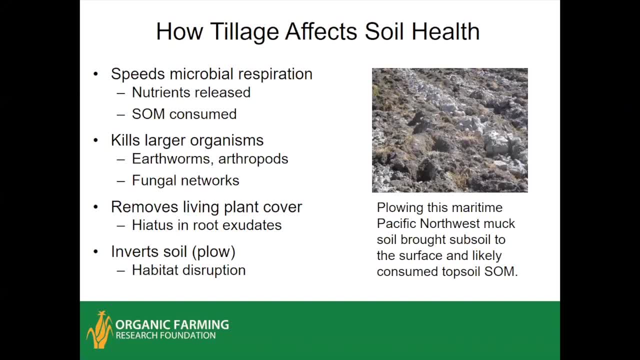 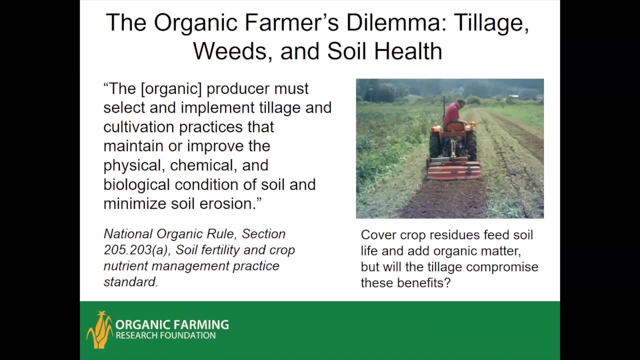 buried the most biologically active surface organisms under several inches of soil, So it's like having your house turned upside down. So organic farmers face a dilemma. They're not using herbicides, So there is bound to be some need for tillage. 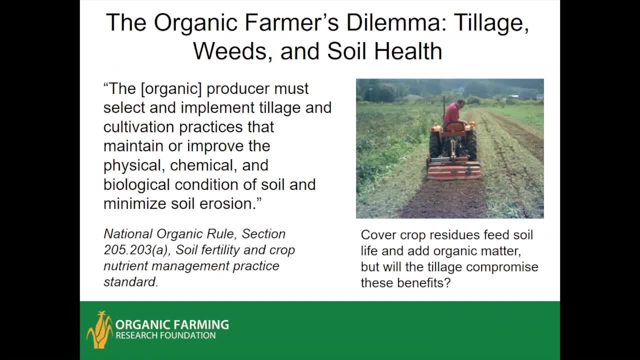 There is a need to manage cover crop residues and, of course, to manage weeds so that they don't out-compete the crops, And so in the picture here you see the farmer tilling in a recently mowed cover crop. that's quite a substantial biomass. 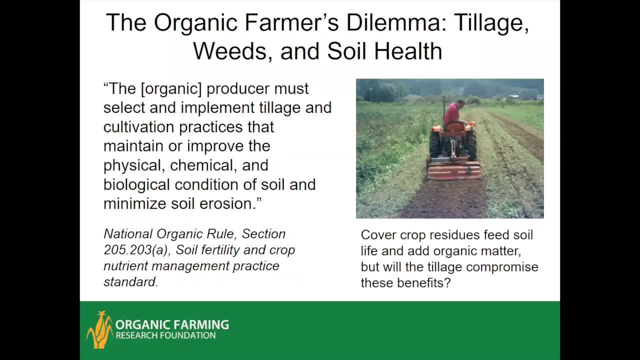 So it's feeding the soil but at the same time it's disturbing the soil to a pretty fair extent. That's a rototiller there. So the National Organic Rule here says that the organic producer must use tillage practices that will maintain the soil. 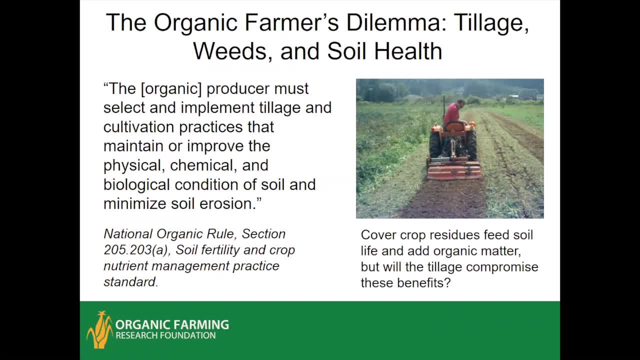 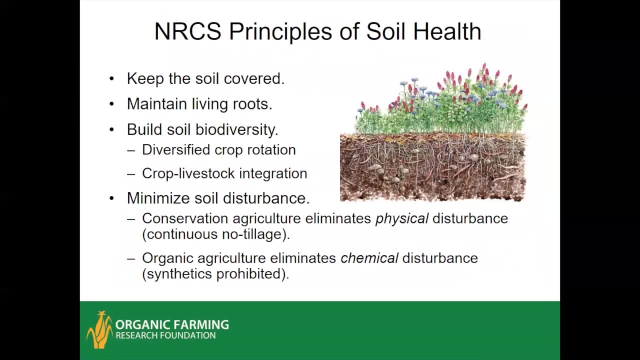 Maintain or improve the physical, biological and chemical condition of the soil and minimize soil erosion, Basically find a way that maintains soil health. And that's almost a paradox, and yet it basically sums up the challenge that we're all facing. So research has shown that, on all these aspects of soil health, the NRCS-4 principles of soil, 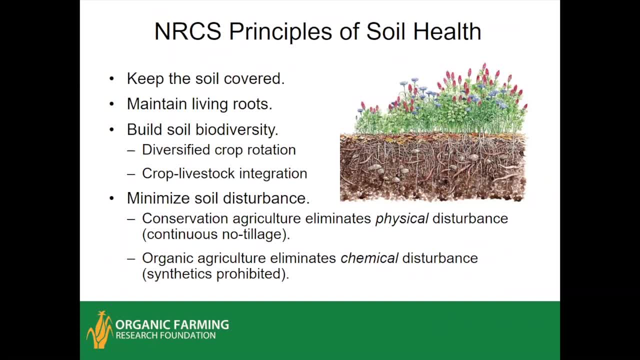 health management is an excellent place to start, And I'm going to show you some examples. Here we go. So the NRCS-4 principles of soil health. Here we go. So the NRCS-4 principles of soil health is an excellent place to start. 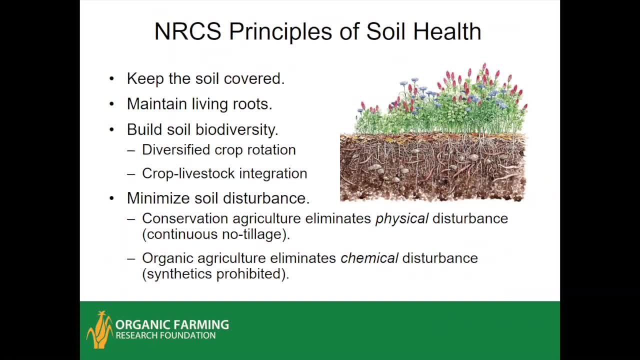 Simply keeping the soil covered by living or residue plant material. There's an excellent farmer in North Dakota. Gabe Brown has a 5000 acre ranch. He calls it keeping the soil armored. It keeps the surface covered so that the impacts of raindrops don't disrupt and seal over the 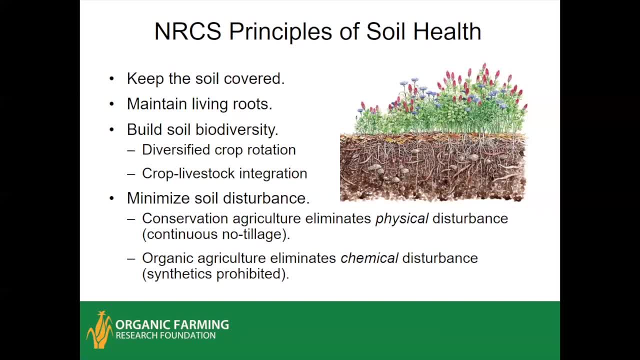 surface and cause erosion. It also keeps the soil surface from getting too hot, Maintaining living roots. That is that food pipeline. It's a pipeline to all of the soil life. The more biomass you have growing above ground, the more root exudates and root turnover you. 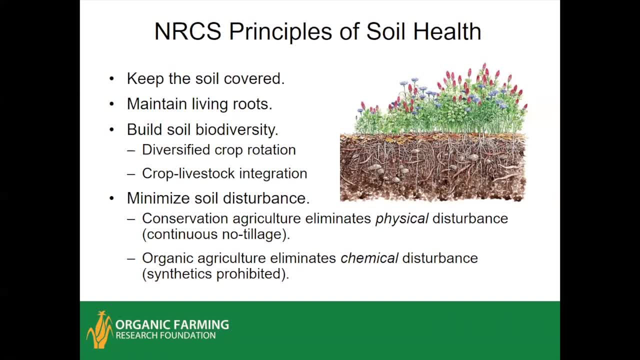 have The small roots dying and providing a continual supply of food, The more you will support an active and healthy soil food web And building soil biodiversity. This is done through diversifying what's growing above ground. Each crop has a different root architecture. 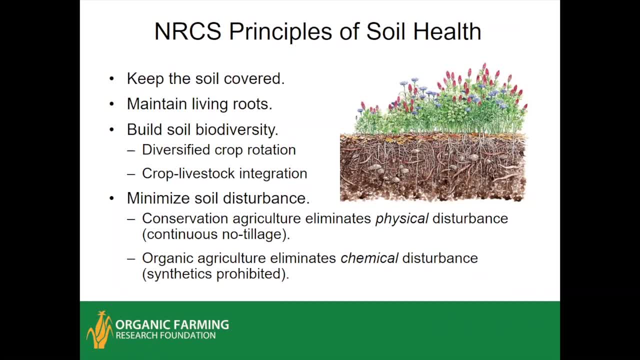 Each crop species a different set of exudates And other materials sloughed from the roots, And it will also send out a different set of specific signals that either encourage or discourage specific soil organisms to associate with growing the root zone And, of course, minimizing soil disturbance. 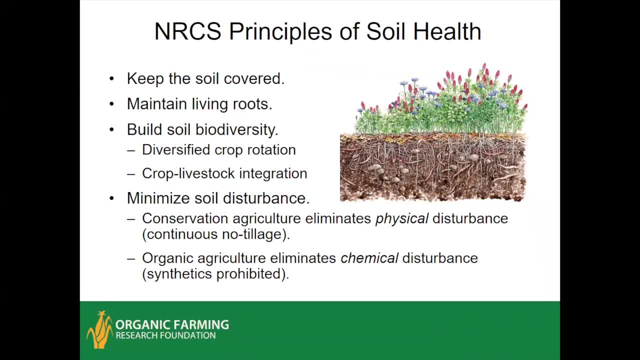 And this includes both physical disturbance- tillage over grazing which compacts the surface, traffic etc. And also chemical disturbance, And it provides a baseline disturbance: the use of synthetic chemicals. high levels of soluble fertilizers definitely disrupt the soil, soil life and, of course, anytime you 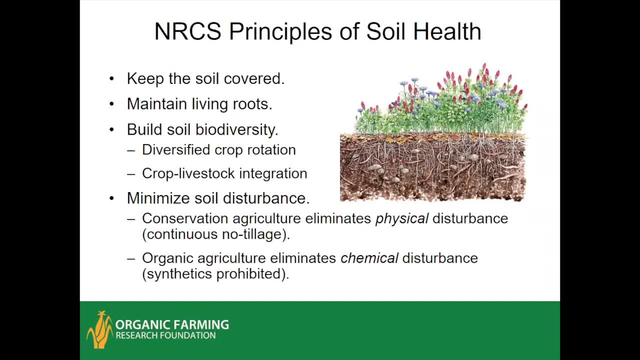 spray, a crop protection chemical intended to kill a certain pest organism or disease organism, it will have some effect on the soil life. So two parallel, complementary approaches to minimizing disturbance. conservation agriculture basically eliminates physical disturbance going by calling continuous no-till, and then allows some use of the synthetic chemicals, as on an as-needed 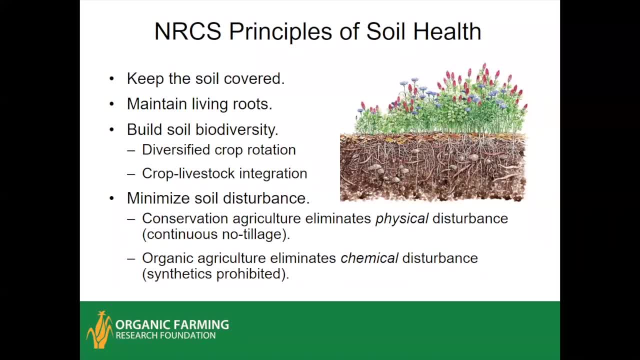 basis, although it definitely aims to reduce it, And the other organic agriculture, through the National Organic Program, rules, standards, eliminates chemical disturbance by preserving the soil life. So that's one of the things that we're trying to do here. So that's one of the things that we're trying to do here. 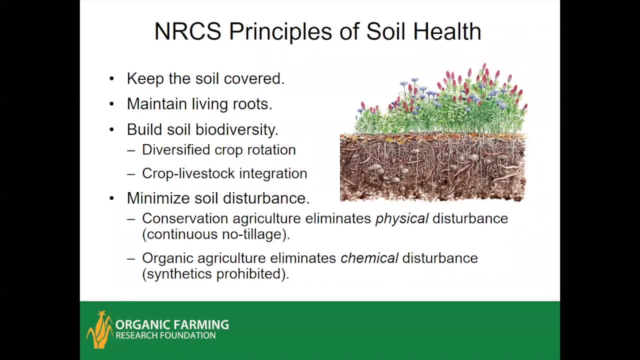 One is prohibiting synthetics and, as noted earlier, allows for judicious tillage, so there's some physical disturbance in that situation. Another way to build soil biodiversity is crop livestock integration, and related to that is management intensive rotational grazing systems, which have shown a lot of benefits in building soil health. So let's put no-till into perspective. 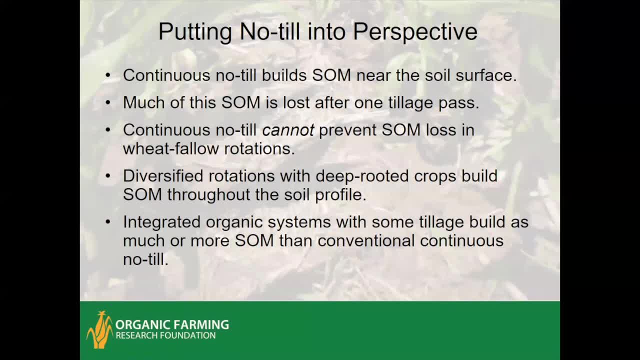 and, for example, in the United States. there are many challenges in the And there are some soil scientists, conservationists, who say you cannot conserve soil without going continuous no-till. And this really puts the organic farmer in a bind because you know, once in a while you've got perennial weed. you've got to get out there with some form of tillage implement if you're going to make a living. 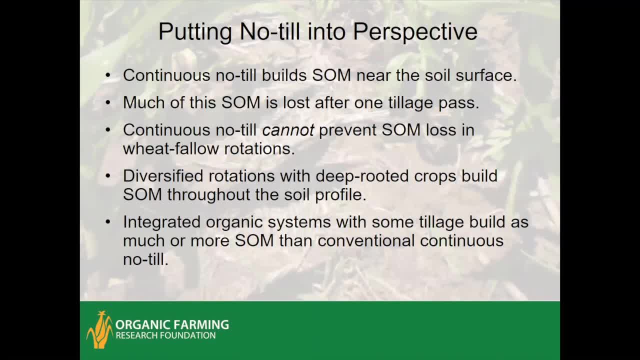 And I'd rather see an organic field get tilled up than have the farmer go out of business and it sprout condominiums or worse. So there have been a number of other research studies on no-till by itself and no-till integrated with other practices that pertain to those four principles of soil health. 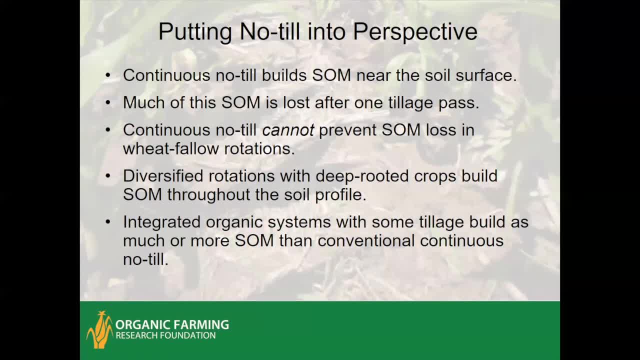 Continuous no-till. in and of itself, particularly within the context of a conventional rotation such as corn, soy wheat, with no cover crops, some bare soil periods in there, that builds some soil organic matter near the soil And that's a really good example of how soil organic matter is lost on the surface in comparison to conventional, the same rotation and inputs with tillage. 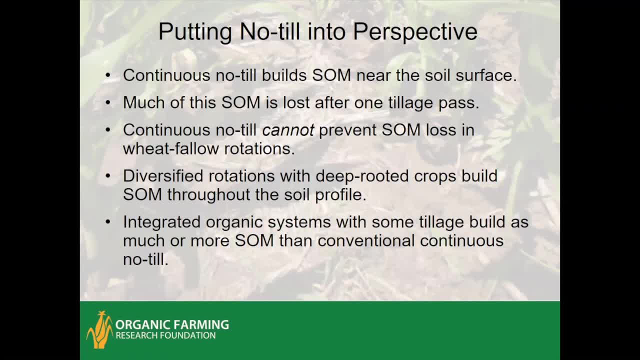 However, a lot of this soil organic matter is lost after one tillage pass because it's protected physically in aggregates, large aggregates. So even one light tillage pass will tend to break some of those aggregates and you'll have a lot of that accrual reversed. 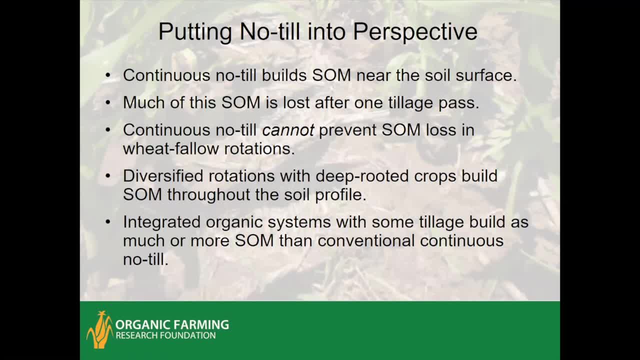 And one of the things that a number of studies in the semi-arid interior, north, central and northwestern regions wheat fields have shown is that the soil organic matter is lost in fallow rotations, which are often the traditional farming system: a year of winter wheat planted in the late summer, harvested in the early summer of the next year, followed by 12 to 14 months of fallow. 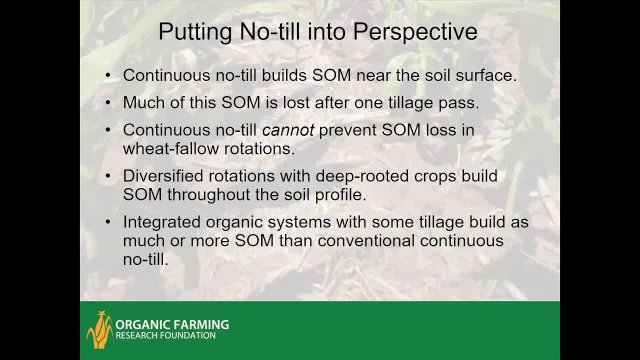 with the intent of saving up a year's worth of moisture so that you use two years of moisture to grow your wheat crop. Unfortunately, even with continuous no-till, this cannot prevent the loss of organic matter. Soil is degraded In wheat fallow rotations even without tillage. 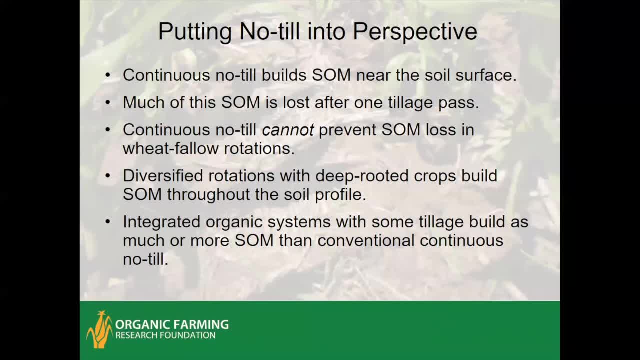 However, if you diversify the rotation and you make sure there is some crop growing each year, perhaps a shallow rooted one that serves saves moisture, you can build gradually, build soil organic matter in those dry land soils, As a number of studies, with diversified rotations that have deep rooted crops and a high diversity of crops, that building the organic matter throughout the soil profile. 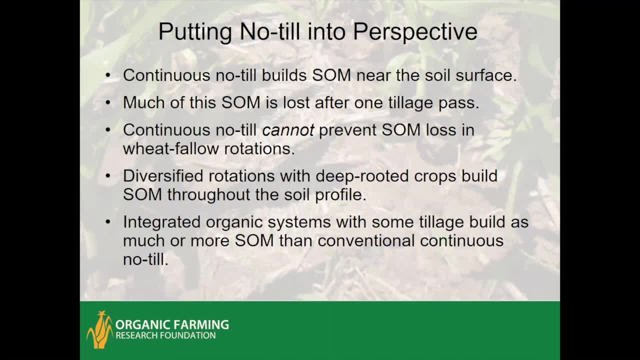 can be a good way to reduce the loss of organic matter, So that if you have to come in until three or four inches deep to deal with weeds, you are not going to be destroying all that organic matter. A lot of the organic matter that's formed through maximizing living root and maximizing plant cover and diversity is of a more stable sort than that. that's simply a crude near the surface, through no till. 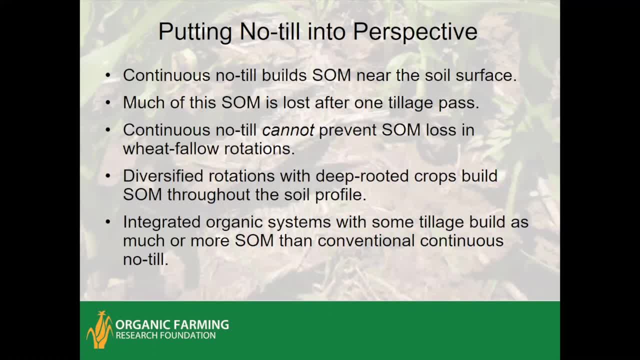 And they have been an under a number of studies, with integrated organic systems that include some tillage and build as much or more soil organic matter than the conventional continuous no-till. There's one study out in Beltsville, Maryland. I know it's not in the western region but it does have. 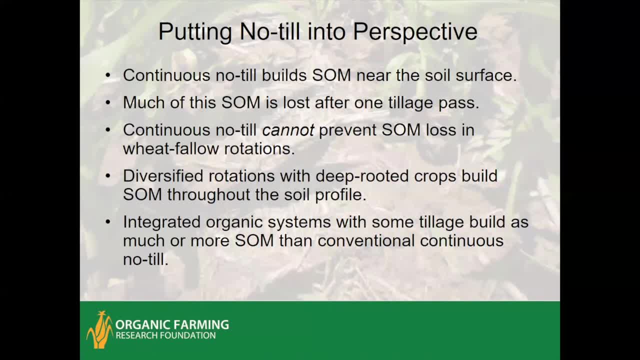 some relevance to the whole country. But the organic system that included some tillage every year. one pass every year accrued about twice as much soil organic matter over 13 years as the continuous no-till system. And I want to point out there's a farm in Montana, Doug and Anna. 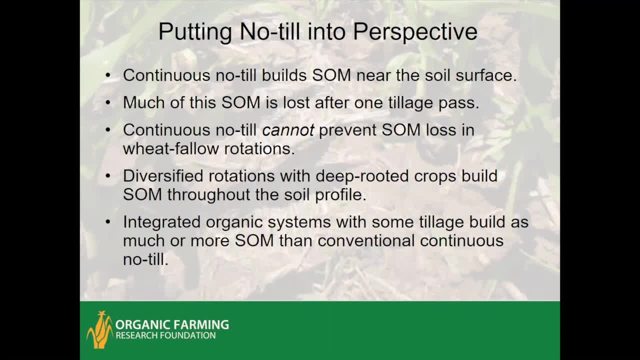 Crabtree manage 7,000 acres of dry land, grains and pulses in a highly diversified rotation. They do not fallow, They use. this is Villicus Farms in Hill County of Montana. We'll talk a bit more about some of their work, but they have built soil organic matter substantially over. 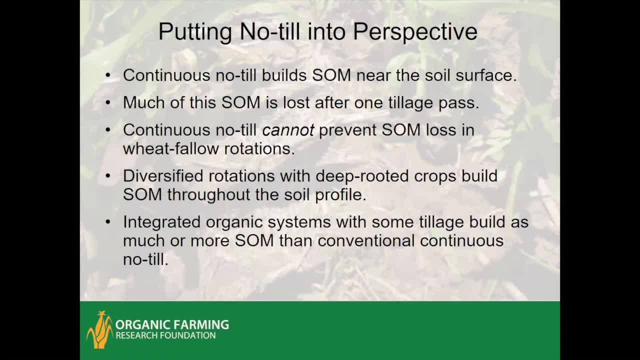 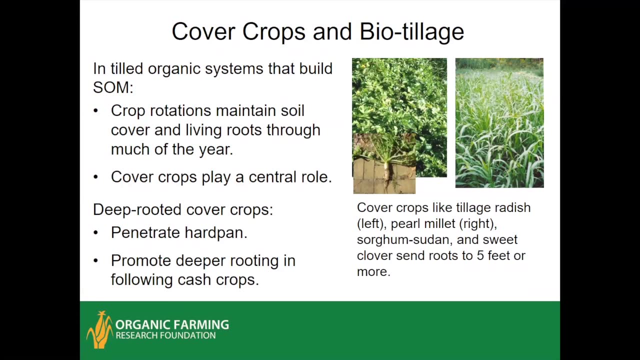 a number of years and improved the soil moisture holding capacity as well. And they do till some. Of course they take great care to minimize soil damage. So cover crops, Tilled organic systems that build soil organic matter have two main characteristics, key characteristics to note. One is they maintain soil cover and living roots as much of the year. 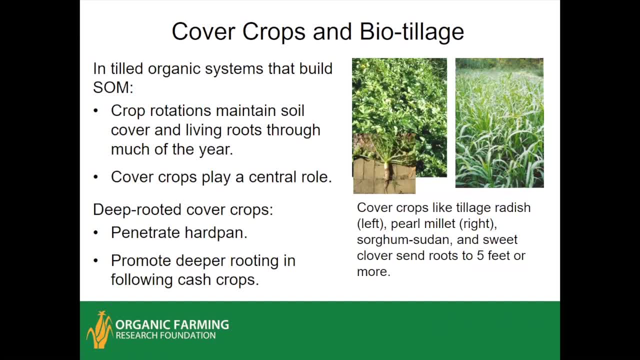 as possible. You do not see a lot of bare soil. in that, rotation And cover crops play a major role. They maintain soil cover and living roots as much of the year as possible. You do not see a lot of bare soil. in that, rotation And cover crops play a major role- Some cover crops actually. 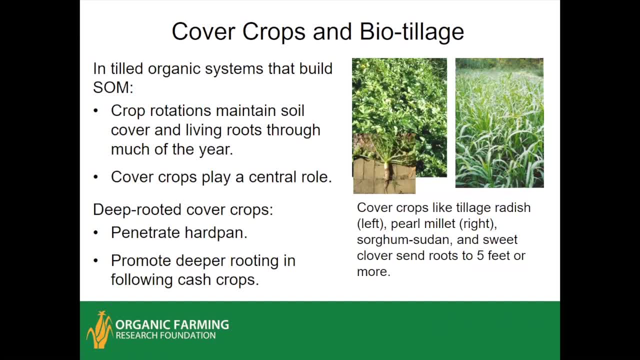 provide what might be thought of as biological tillage, because they send deep roots down as far as five feet and open up the soil profile. They can actively penetrate hard pans. that will deter a lot of production crop roots and severely restrict their ability to obtain deep moisture. 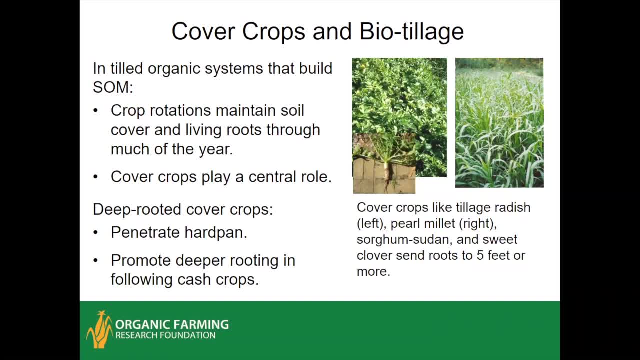 and nutrients. For instance, tillage radish is an excellent example. It'll just break right through a hard pan and it'll just break right through a hard pan and it'll just break right through a hard pan And the following crop is shown to send its roots much deeper And it benefits the yields of those. 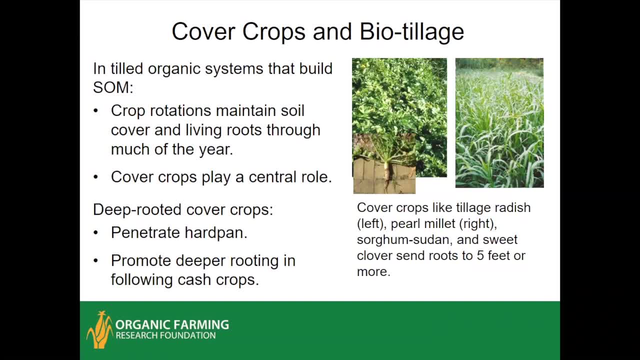 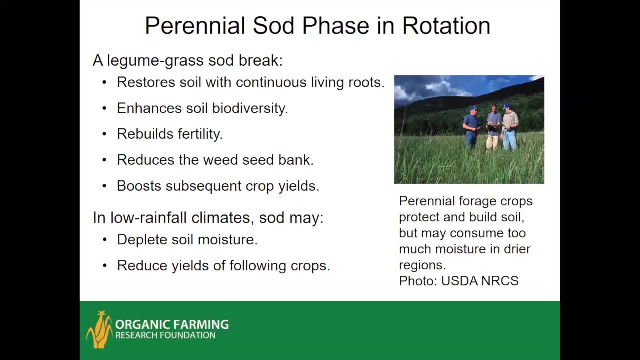 crops, partly through conserving and recycling nutrients, but partly through improving the rooting depth and the moisture capacity access. Perennial sod phase is an excellent practice in general for restoring soil because it provides continuous living roots in a protracted period of no till, Even one year, but especially your two or three years, you'll see an enhancement of 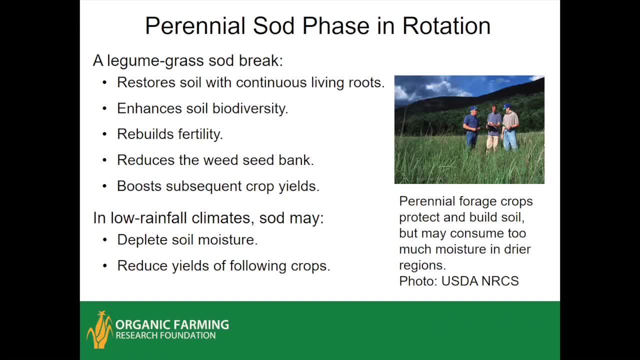 overall fertility, soil health. The annual weed seed bank tends to run down. between the fact that those weeds are not able to complete their life cycle and weed seed consumers that live in the continuous sod will draw the existing weed seed bank down. Very often you see an improvement in 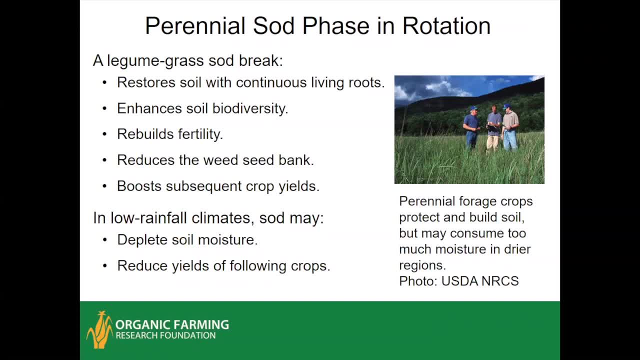 yields after that sod break. Big caveat is that in areas of low rainfall the sod may deplete soil moisture and a deep-rooted sod sometimes has been observed to deplete soil moisture so badly that the next two or three years of production crops suffer a yield. 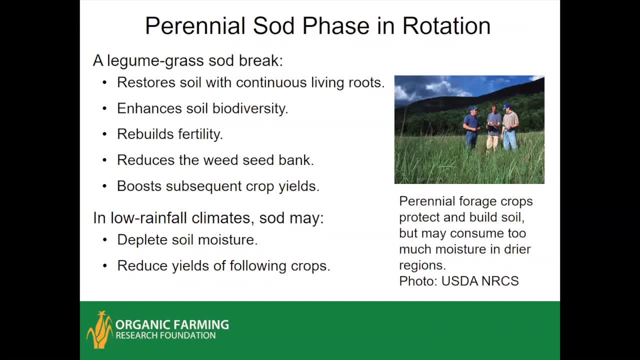 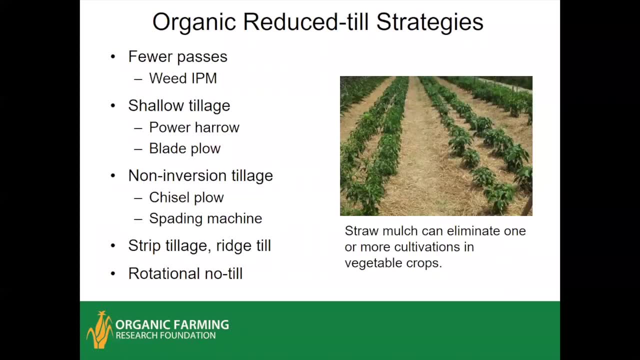 reduction as a result of that limitation. So with that one caveat, in appropriate situations this is an excellent practice. Here's a few strategies for reducing tillage. One is just reduce the number of passes. Every time you take a tillage implement into the field, you're creating some disturbance. 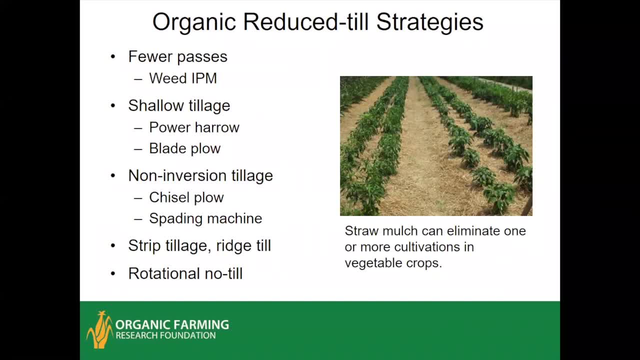 You're going to lose some organic matter, lose some soil life. So if you can simply reduce the number of passes, Another is to till more shallowly. A couple of implements that allow shallow tillage is something called a power harrow. It's really good for creating a seed bed where the residues 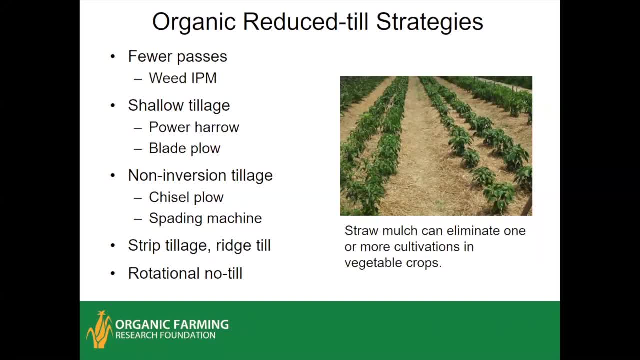 are not too heavy And the blade plow or sweet plow, undercutter. I've not actually seen one of these in person, being from the East Coast, but the more I've seen them, the more I've seen them. So if I read about Western region agricultural challenges and solutions, the more I learn how. 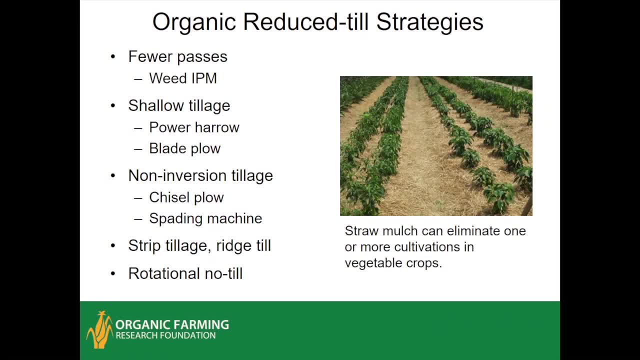 important a tool is is it basically undercuts the existing vegetation a very short distance below the surface. It takes out the root crowns, leaves most of the residue on the surface and leaves most of the soil profile undisturbed. Non-inversion tillage is another way to approach. 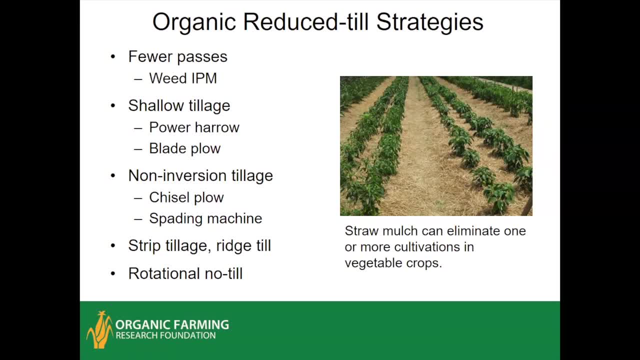 this Chisel plow spading machine. we'll talk about the spading machine in a little bit. Also tilling, not the whole fields, doing a strip or ridge till, And that's a very interesting strategy because it concentrates the benefits of tillage, which include nutrient release and 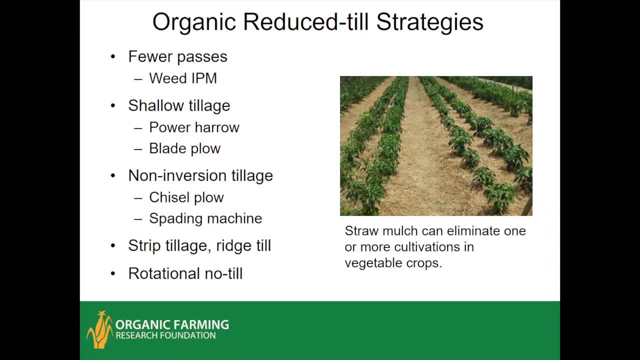 more complete weed control right in the crop row where it's most critical, And it reduces the adverse effects by not disturbing the between row spaces. And then there's rotational no-till. We do not have any means to do continuous no-till in an organic system at this time in an annual crop rotation. However, some major primary 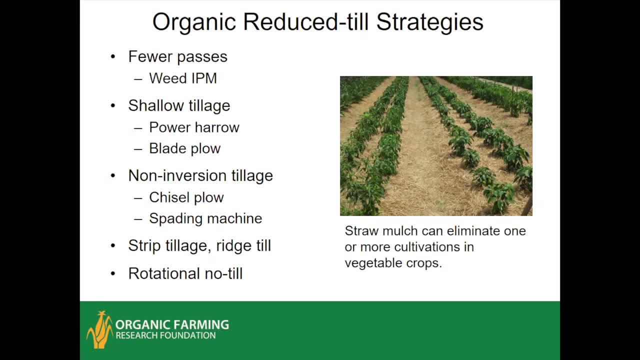 tillage events can be eliminated by roll crimping the cover crop and planting the cash crop. no-till through that. But let's go back to fewer passes of classic example right here: just using straw, If this farmer had not put it down a good straw mulch on the tomato and pepper crop here. 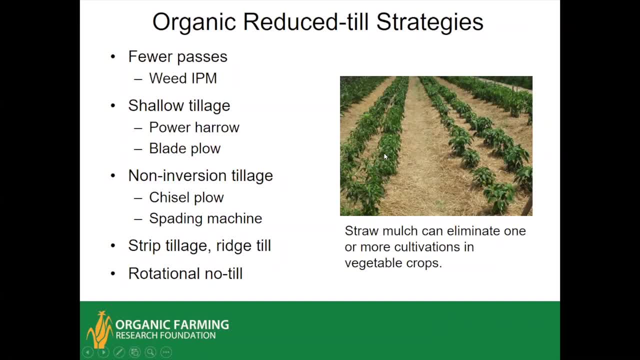 he would have been out there holding the crop And he would have been out there growing or cultivating at least a couple more times to keep the weeds down. So right there, any kind of integrated weed management that uses multiple tactics and reduces the number of times you have to get out there and cultivate, that is reducing tillage. 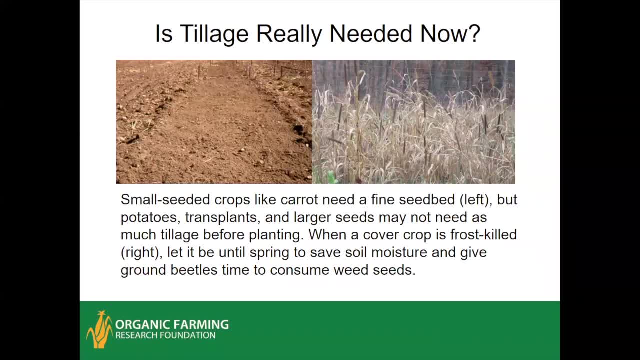 One thing to remember is you always want to ask yourself: do you really need to till right now And if so, what is your purpose in doing the tillage? Because, for instance, that very fine seeding the seed bed on the left, that may be important for something like planting carrots. 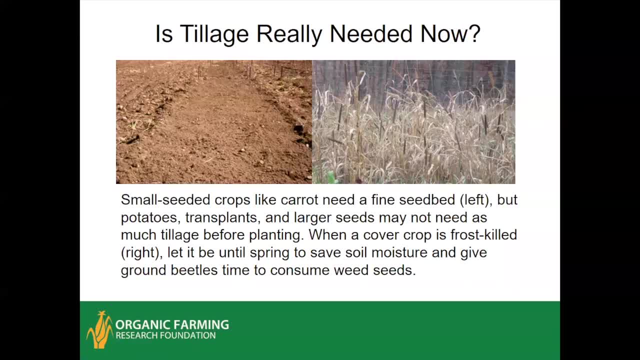 But having worked the soil that fine is even more vulnerable to both wind and water erosion and simply compaction and surface crusting if you get a heavy shower on that. So if you're planting something with larger seeds, like beans, you're putting garlic cloves or potato. 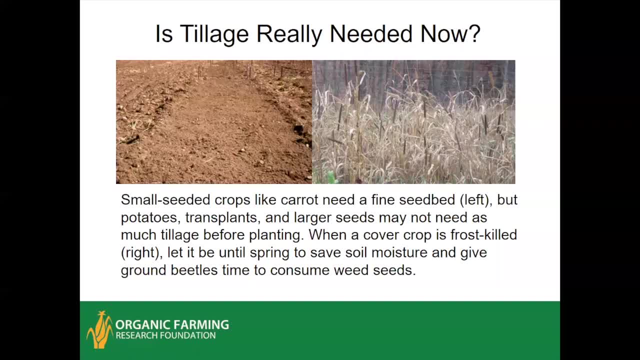 seed potatoes, and you could certainly go with the more coarser seed bed that you see on either side of this fine tilled pass, And maybe you don't even need that much tillage. Another thing: if you've had a summer cover crop growing like this pearl millet over here, 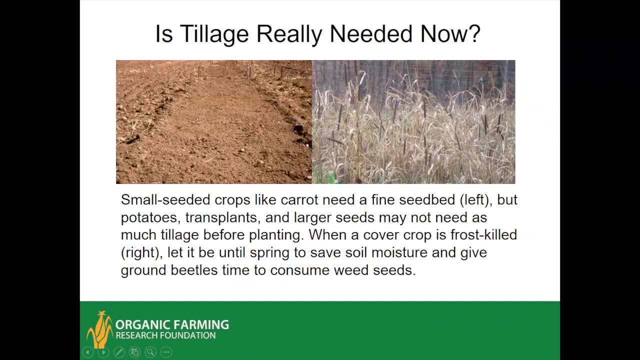 and you get a heavy frost in October and it's killed. definitely don't be in a hurry to till that under, In fact leaving it standing or maybe rolling it so that it's easier to manage in the spring, But you don't want to disturb the soil and the root mass in the fall if you can avoid it. 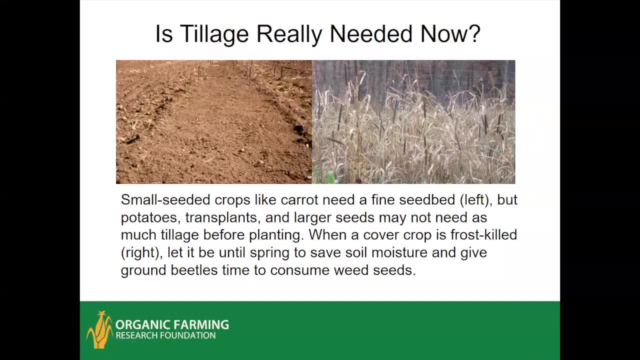 There may be some circumstances where you might want to do that. There may be some circumstances where leaving residues over winter will create excessively wet conditions for getting an early crop in, and then perhaps you need to make some kind of compromise. Another thing that happens, though, if you leave those residues in place, is you're leaving the soil surface habitat undisturbed. 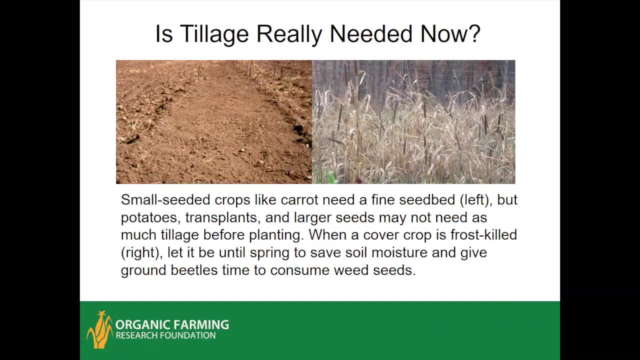 So the ground beetles and the other weed seed consumers will clean up any weeds that have grown and set seed during the course of the year. And of course, if that cover crop was really thick it probably wouldn't have any weeds, But you definitely want that clean up. 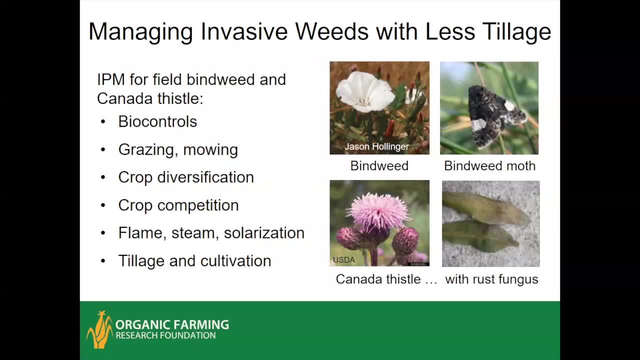 Clean up crew to be able to do its job. So just addressing a couple of very invasive weeds. We have Canadian Canada thistle here in Virginia. It's been a pretty serious weed for us as well. I know it's very serious out in large part sections of the northwest. 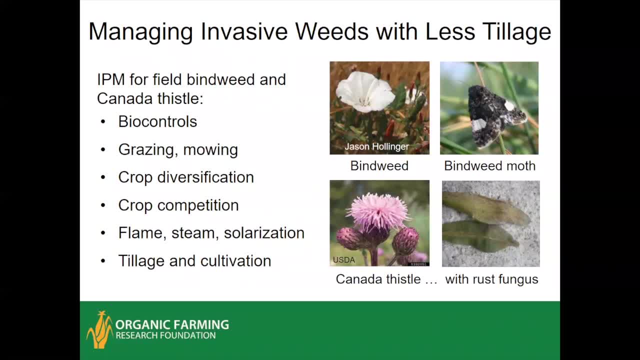 I'm less familiar with field bindweed. We have its kid brother, hedge bindweed, and it's bad enough. But these pose a real challenge. You really can't stop either of these. We have a lot of weeds with a roll crib cover crop or with very, very low level of tillage. 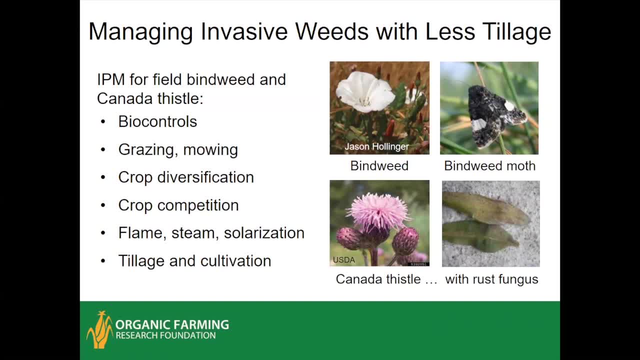 So we need to find ways to hit them with as many different weed IPM strategies as possible. There are some recently awarded organic research and extension initiative grants that are looking into biological control. The bindweed: there is something called a bindweed moth that's been found to be a very good biocontrol. 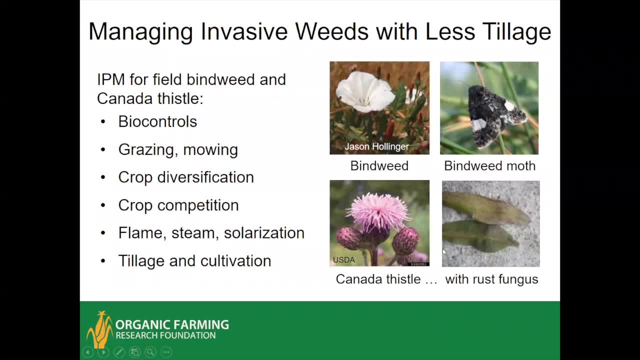 Eats them down quite a bit. And Canada thistle is subject to a rust fungus which fortunately does not attack most of our crops. Fairly specific for thistles, So integrating these with grazing and mowing, crop diversification, direct competition from crops. 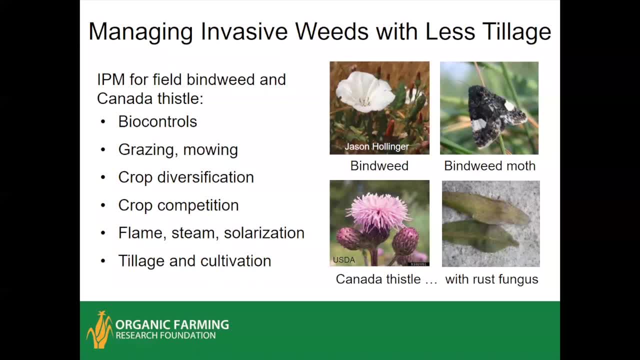 There's been some progress of using steam like a steam weeding treatment at a certain temperature and tractor speed has been found to significantly reduce the vigor of the bindweed. Now, as I said, this is an alternative. You can do this with a little bit of cultivation, but with all these other tactics you won't need as much. 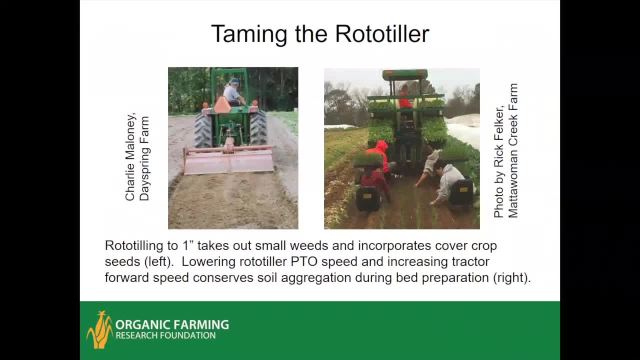 And you won't be sacrificing your soil quality to get these stubborn weeds under control. Research is in progress on that. Okay, here's another thing. You don't necessarily have to go out and buy a fancy tillage, a new tool to go from beating the soil to a pulverized erosion prone state, to being gentler on it. 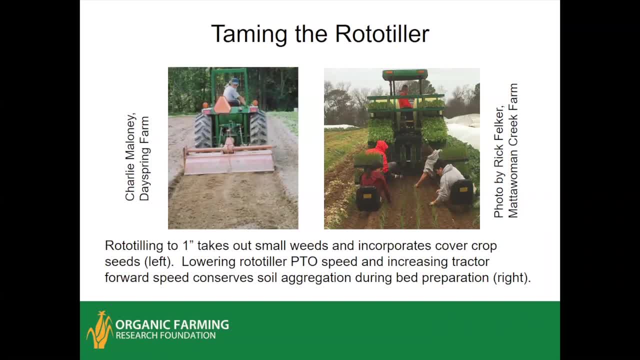 A couple of farmers have shown me ways that you can take this and use this for your crop. So if you want to go ahead and buy a new tool, this is a good way to do that. Okay, that you can tame the rototiller, as I call it. On the left is a farmer in east, in coastal region of 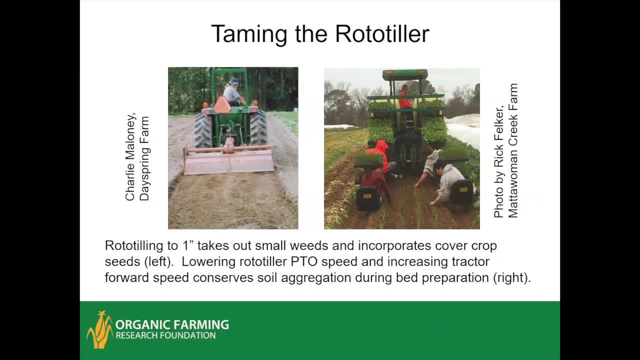 Virginia. He's rigged that rototiller to work only one inch deep and so in one pass he's taking out germinating weeds and planting the cover crop. that is just broadcast On the right hand, Rick Felker, on the eastern shore of Virginia. That is a loamy sand soil and you can see it has considerable. 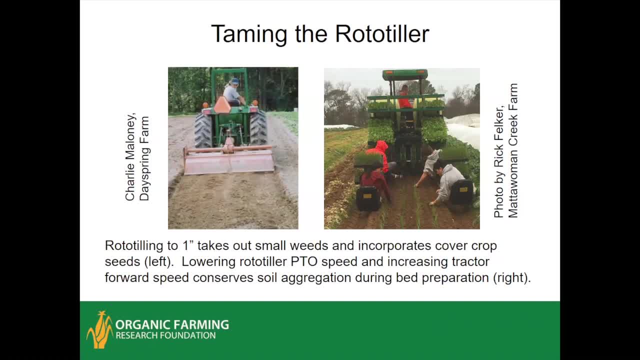 organic matter and it has some soil structure. The way he manages this is his tillage regime- is a bed shaper which rebuilds the bed every year- and that is a fairly gentle way to build the beds- and then runs the rototiller with a higher. 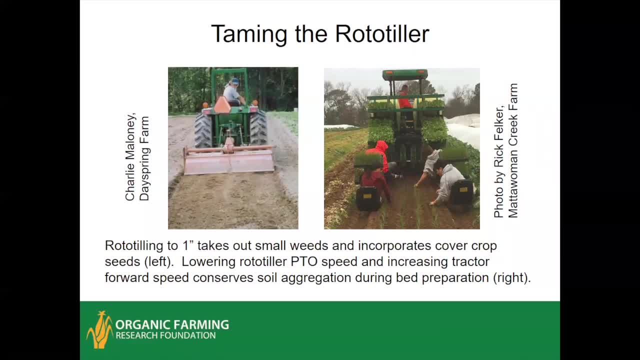 tractor speed and a lower PTO speed so that instead of beating the soil really severely it's more gently going through almost like a harrow to create a seed bed. and he has found he's been able to build organic matter on a loamy sand soil. in those circumstances, 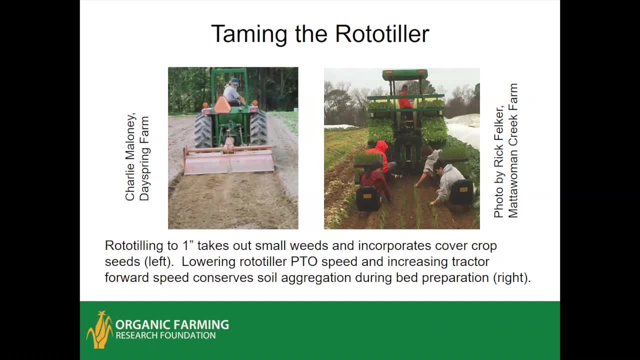 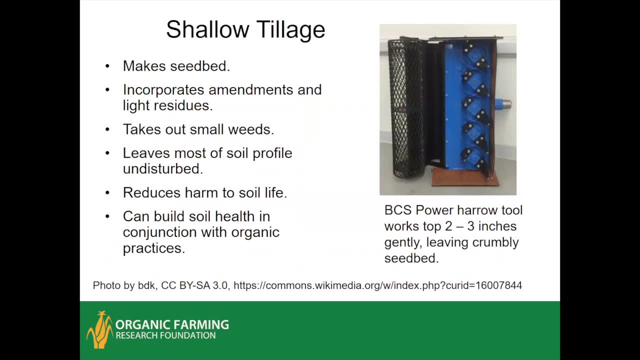 These are techniques that can be applied anywhere. as far as I know- and I'd be interested in hearing others experiences- that Here's a newer implement. the power harrow creates a similar seed bed to what you saw with the rototiller at the low rotary speed. It's a 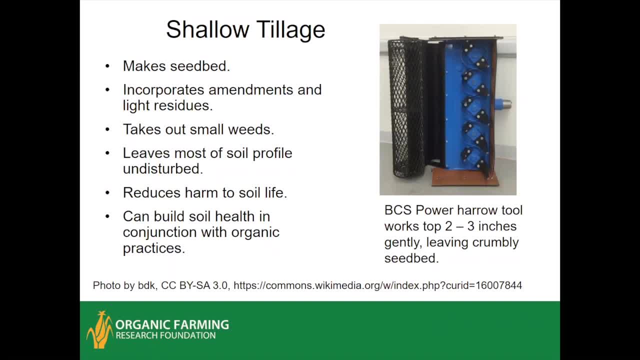 good for making a seed bed, incorporating amendments taking out small weeds, These, most of the rest of the soil profile undisturbed, and there have been a number of meta analyses, which are research studies that look at experiments that have been conducted in all different parts, all different bio agricultural regions around the world, and then compiling, getting a, an average. 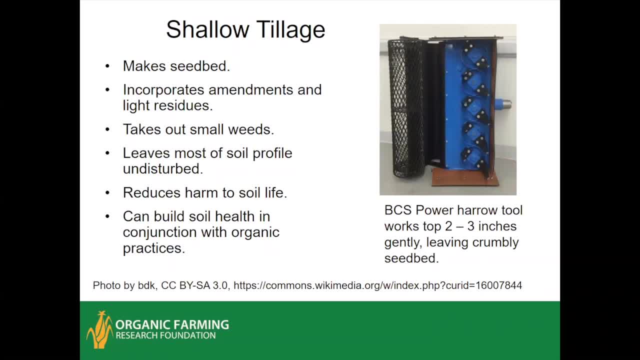 getting a sense of what the overall benefit is, And these studies have found that doing shallow tillage versus doing a standard plow disc really does allow more soil life to continue. there's less adverse impacts on soil life with this method, and the same can be said for chisel plowing as opposed to moldboard plowing. 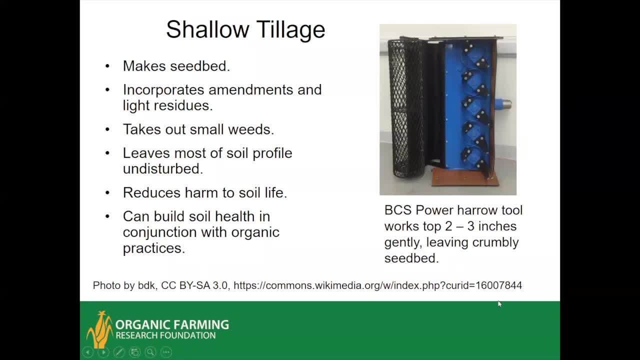 And that was and that is reflected in the NRCS. they have a system for estimating how severity the soil is being tilled, called the soil tillage intensity rating, and they add up all of the field passes during the course of the year. if it's less than 20, it's considered no-till. um, it could be some, you know, like a planter would. 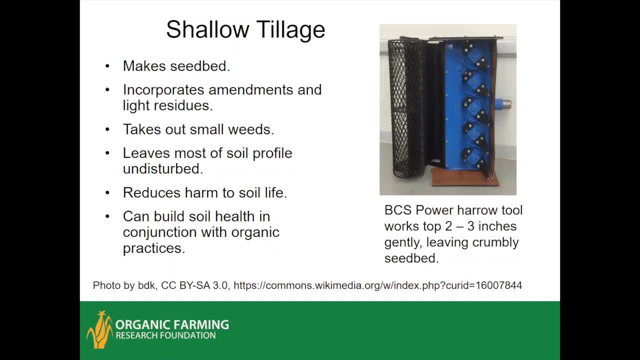 just open the soil slot and have just be a few points. um, i believe up to 80 is considered reduced till. a single pass of the moldboard plow would be 100, whereas a chisel plow would be only 45 and a shallow till implement like this or like a light disc would be more like 20. 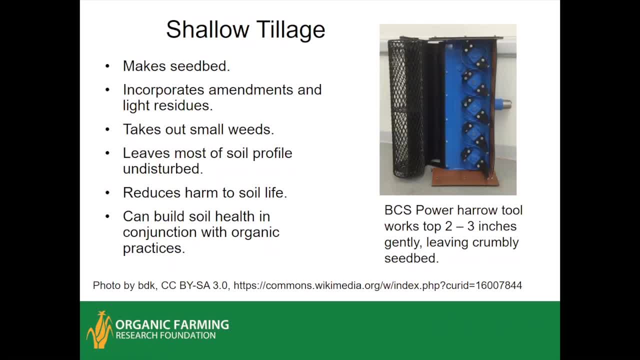 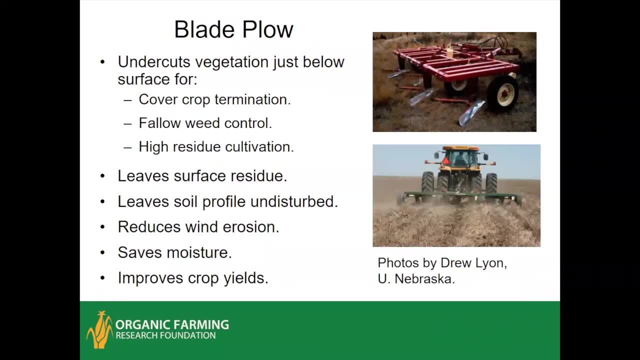 so we can see not all tillage is alike and there are definitely benefits um to taking steps towards less disruptive tillage. this is the blade plow. i got some pictures from university of nebraska. they did some studies in the western part of the state. if you terminate a cover crop with, 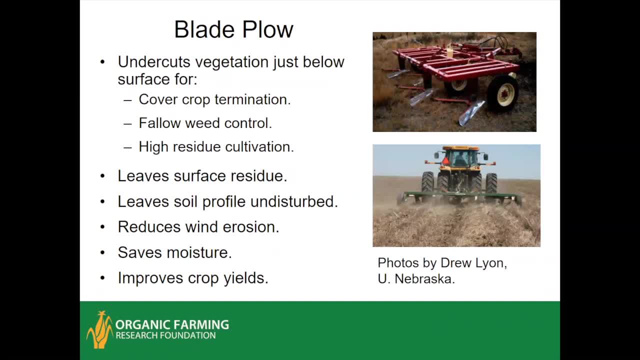 this, implement and grow corn and soybean afterwards. you have yield improvements from the cover crop plus undercut tillage, whereas if the cover crop is simply disc'd in just in the standard and then you have a cover crop plus undercut tillage, then you have a cover crop. 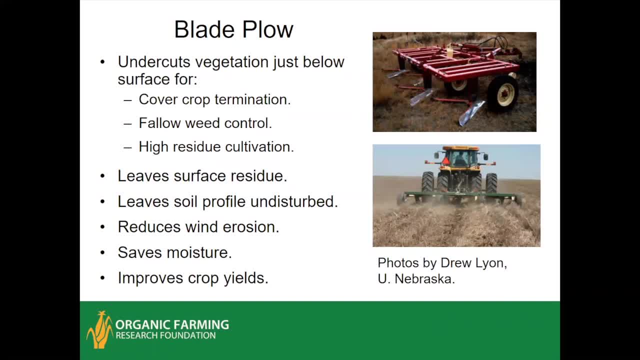 and then you have a cover crop plus undercut tillage, and then you have a cover crop plus undercut tillage, a couple passes with a disc. the soybeans showed a yield loss because there was more moisture lost. With this implement. you see that the residue is left on the surface, conserving moisture. 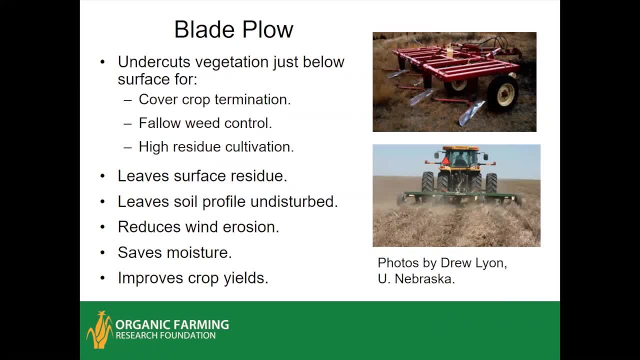 and the fact that it undercuts fairly shallowly allows most of the soil to remain undisturbed. It's been used for terminating cover crops, for weed control during the fallow period of a rotation and also high-residue cultivation. There are other implements of a similar design that run between the rows and up close to. 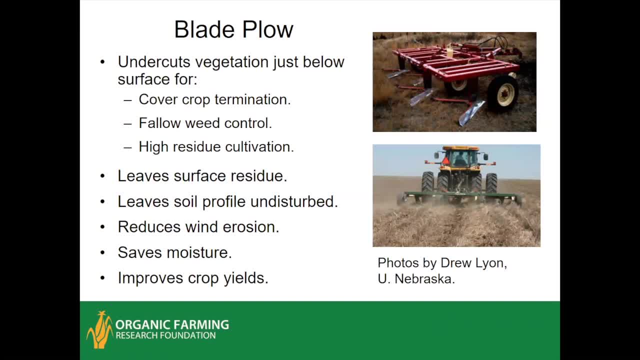 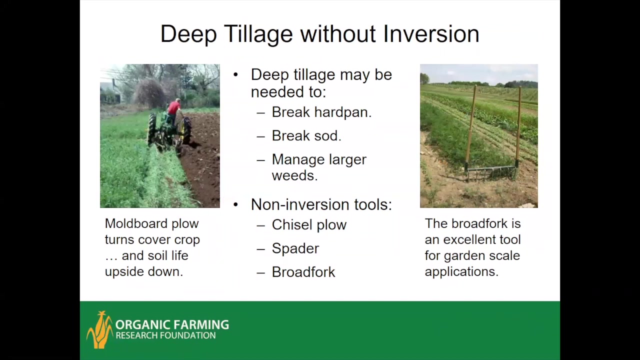 but not into the row and undercut most of the weeds in a high-residue system. Studies in the interior Pacific Northwest have confirmed that using this tool in lieu of the disc will save moisture and reduce wind erosion. And then I mentioned deep tillage without inversion, that moldboard plow on the left. 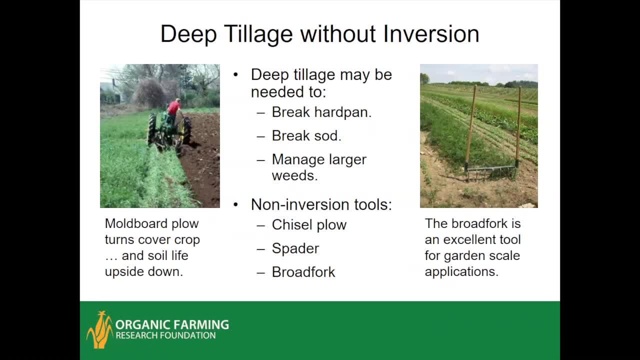 that was many years ago. I took that picture and, yeah, it's turning the whole soil upside down. These are great seedbeds but definitely quite disruptive Garden scale. the broadfork is a really fine tool. A lot of gardeners consider themselves no-till and they will broadfork once a year. 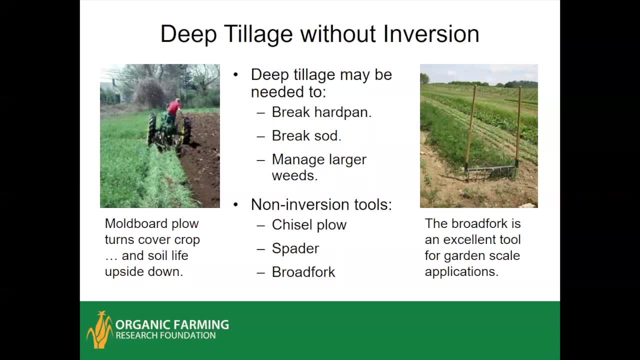 And you're really gently fracturing the soil, breaking up hard-panned loosening weeds. you can then pull them out. Here it's being used to dig carrots. Carrots are also another relatively good way to use it. Chisel plow at the farm scale is an example of a non-inversion deep tillage tool. 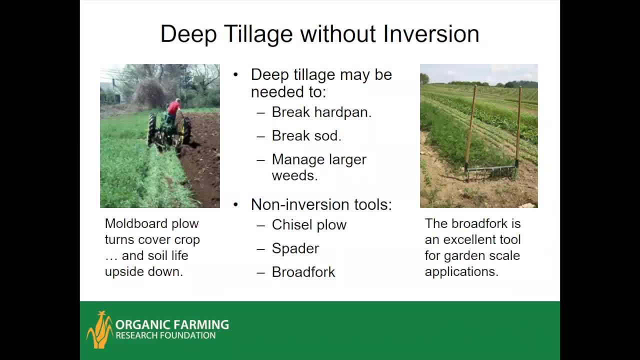 And it can be used to break through hard pan, even to break sod, And these are the situations where you're going to actually need to do- maybe do some deep tillage. If you're doing an organic farm, you have a hard pan you've got to break through. 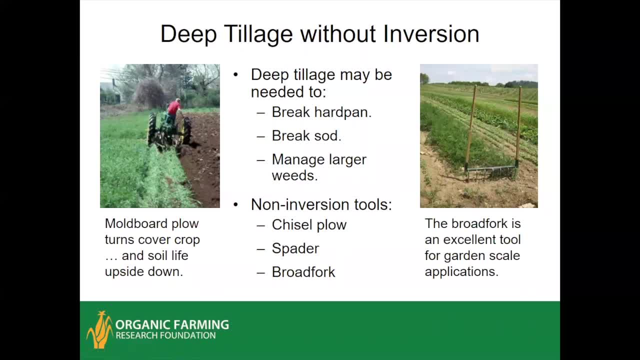 A lot of times cover crops will do that work. On some occasions It may be the best bet to do it first with a tool and then follow with a cover crop. Breaking sod is very hard to do unless you're going to have a small enough scale that you can do it with tarps. 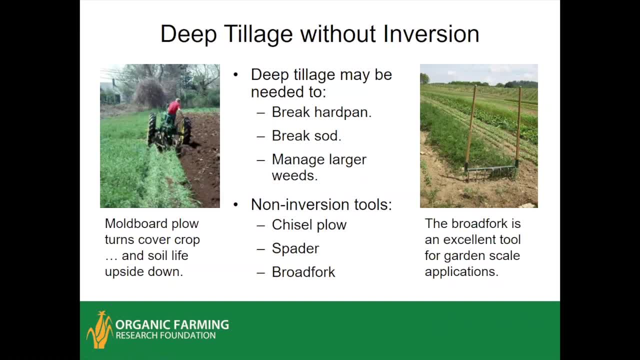 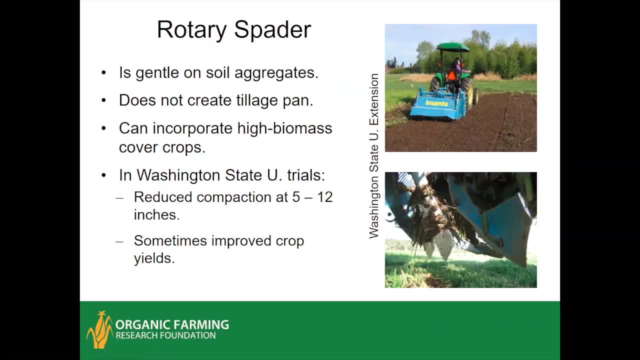 and just kill it. no-till that way with opaque tarps. Larger weeds sometimes require the deeper tillage Rotary spade or spading machine. This is probably one of the best inventions for small-scale vegetable growers. It's a fairly slow process. 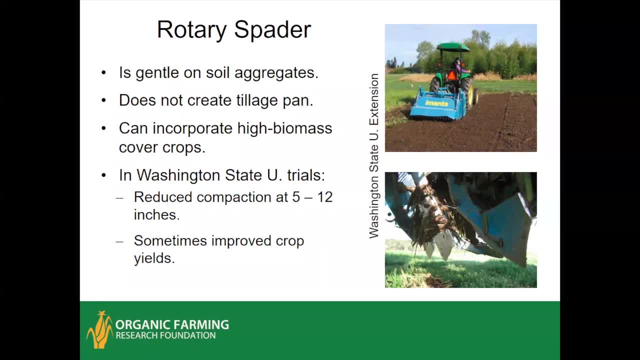 You have to drive through the field gradually, but this can actually break sod and make at least a coarse seed bed, Something that's suitable for planting potatoes, for instance, in one pass into sod, or a very heavy cover crop with less residue. One pass will leave you a seed bed that you can plant just about anything in. 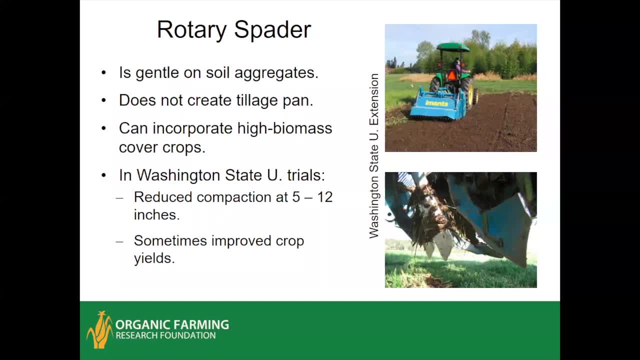 It's a lot gentler on soil aggregates than rototilling or heavy disking. It does not create a tillage hard pan. In fact it relieves hard pan. In Washington State University multi-year there were farming system trials where they looked at the rotary spader versus plowing and disking. 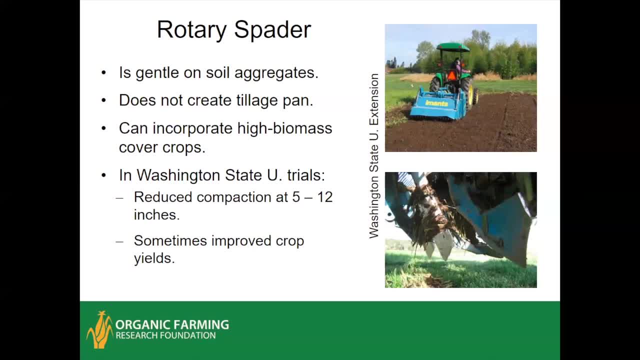 This implemented causes substantial reduction in compaction between 5 and 12 inches below the surface And in about a third of the about 25% of the site years they actually saw an improvement in crop yields. So this became their standard full tillage implement tool when they did further studies on minimum till and strict tillage. 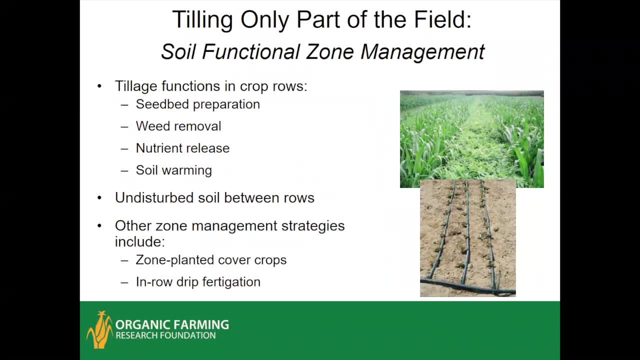 So this became their standard full tillage implement tool when they did further studies on minimum till and strict tillage. So this became their standard full tillage implement tool when they did further studies on minimum till and strict tillage. So here's another strategy to only part of the fields- the strict tillage I've mentioned. 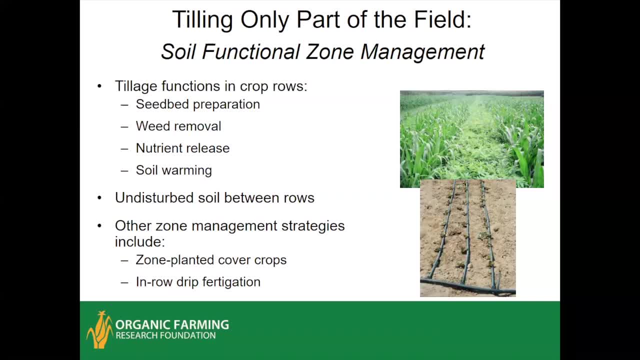 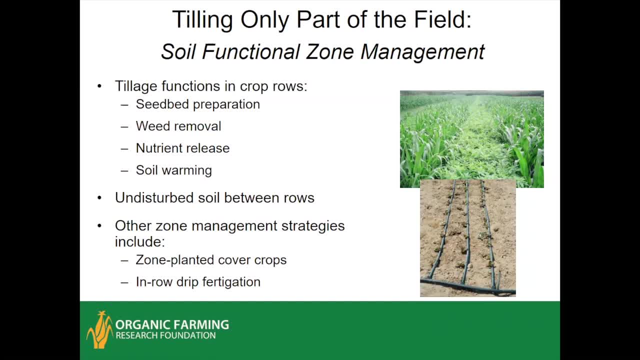 crop going, but we don't have to till out the whole field to do that. if you got a wide space- you know you got tomatoes planted in rows five feet apart or corn planted in rows three feet apart- you can say, okay, well, let's do like work up a six or eight or ten inch wide strip, right. 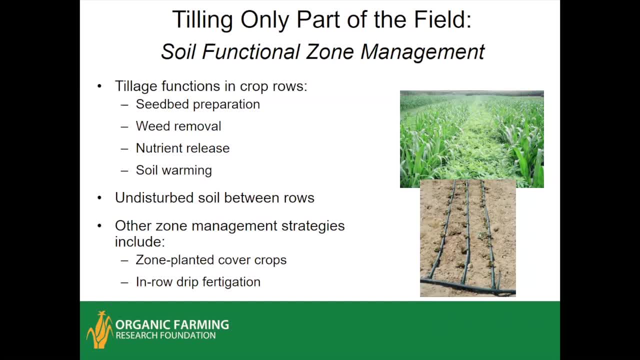 where the crop is, encourage the bacteria to multiply. you know, maybe sacrifice some fungi, but you're encouraging that nutrient release. you've taken out the weeds, you've created a seed bed, you're accelerating the warming, but then you leave 60 to 75 percent of the field. 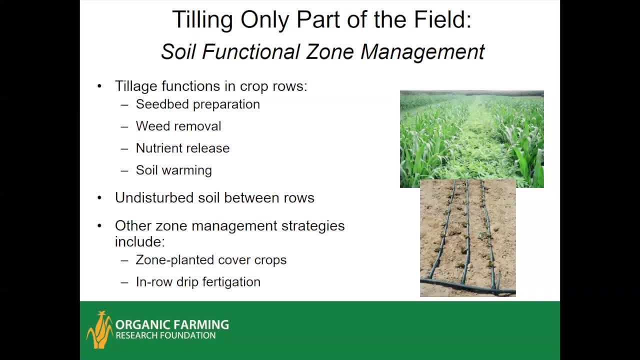 undisturbed between the tilled rows and there are other zone, what I call zone management strategies. you want to get the nutrients to where the crops are and you don't want to be feeding the weeds. so in this picture right here you see the bed tops. this is a organic vegetable. 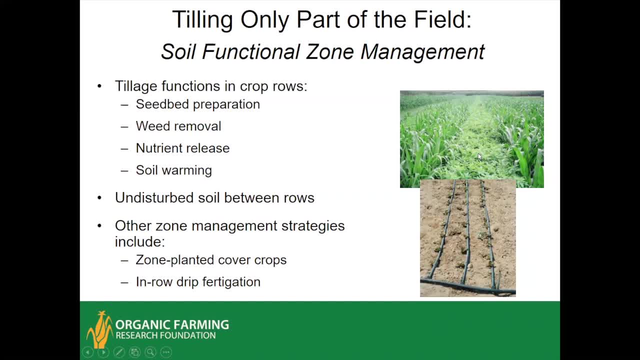 production, actually field trial at a research station here in Virginia. there is a legume cover crop, in this case sun hemp, planted in the crop row which is going to be the top of the bed where they're going to be a double row of broccoli in the fall, And between the rows that's sorghum sudan which is going. 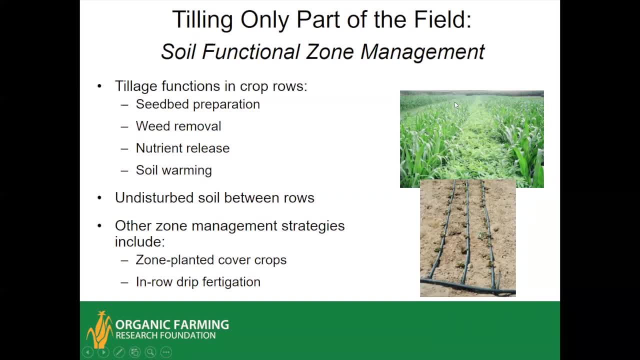 to create lots of biomass, lots of roots, suppress weeds and tie up nitrogen. So there's not going to be much nitrogen available to feed the weeds in the rows, but there's going to be more nitrogen in the crop row all right, on what's called the grow zone, the bed top. 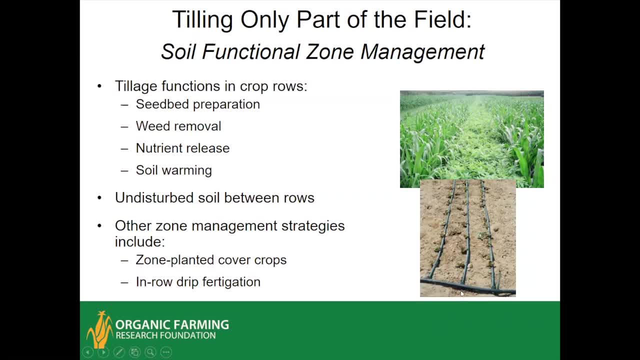 Down below we have drip irrigated lettuce and this can often be used to drip fertigate. There are some formulations of organic fish seaweed-based fertilizers that can be used in drip systems, although I've heard there's still some problems to iron out. 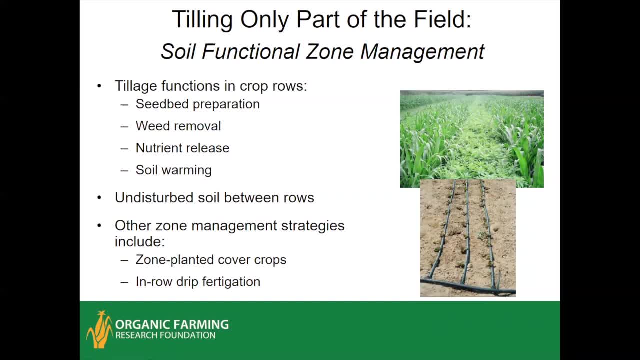 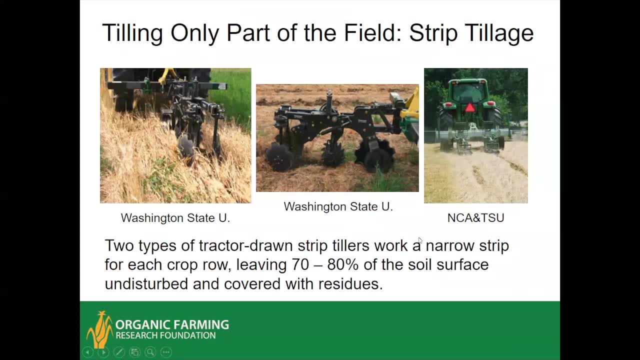 But if you drip fertigate, you're then feeding the crop and not the weed. So here we go: Strip tillage. a couple of things to note here, A couple of examples at Washington State University, and this is one here at North. 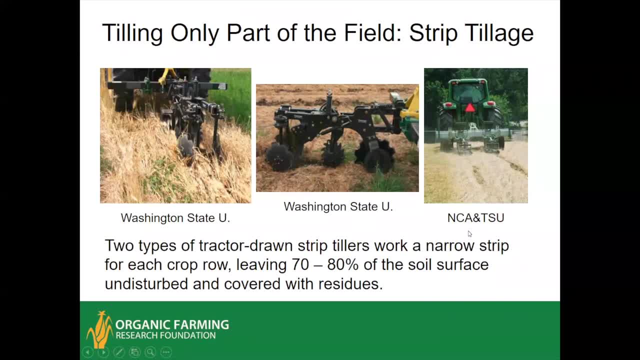 Carolina Agriculture and Technology State University in Greensboro. This implement has an opening coulter and then a shank, and then a narrow rolling basket and some closing coulters. Basically, it leaves a narrow strip that has been worked up and ready. 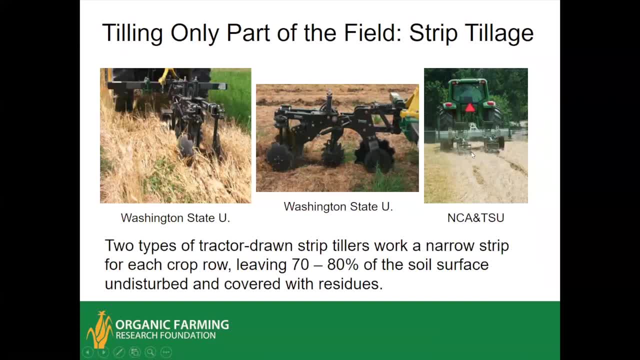 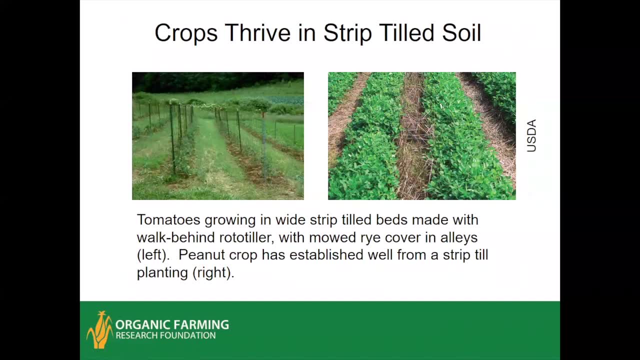 to receive a crop. This one has a slightly different rig, but it's again leaving these narrow strips And here's some cross-planted and strip till situations. Those are tomatoes and five-foot centers. In this case, it was simply a small walk behind. 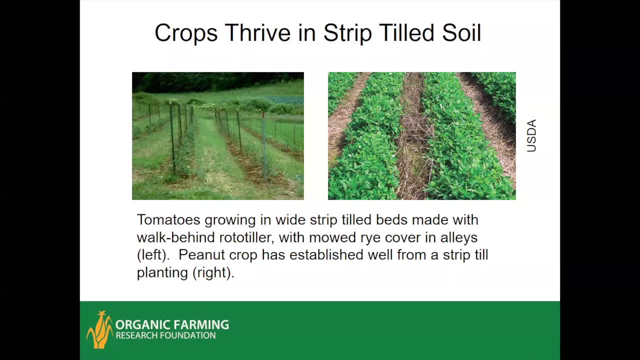 rototiller. So instead of tilling the whole field, the farmer worked up the rows just for the tomatoes and let the rye crop grow and just mowed it periodically, so that it provided a weed-free and also a mud-free alley to walk on between the tomato rows. 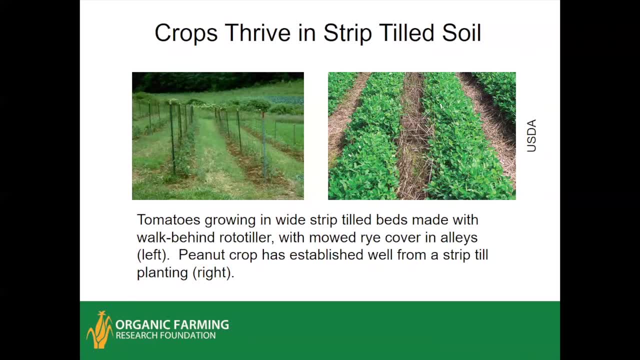 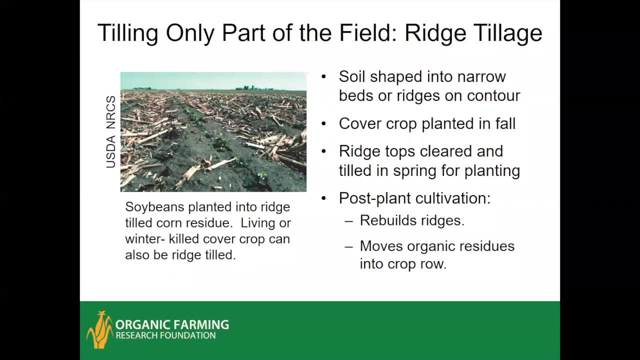 These are peanuts that were planted into a strip-tilled field, also doing quite well. So this is ridge tillage, often practiced in the Midwest. The soil is shaped into ridges and a cover crop is planted, or simply, in this case, the residue of the cash crop is left on. 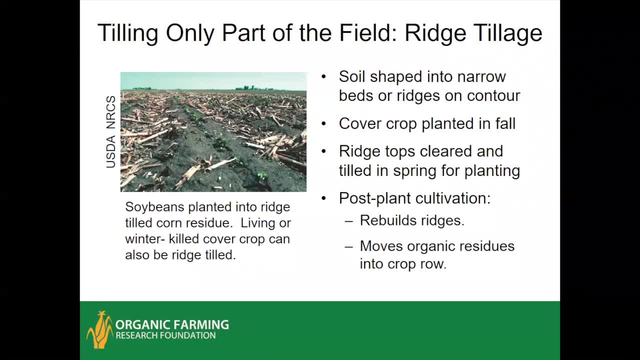 the surface And then in the spring the top of the ridge is basically cleared off. There's a shallow tillage operation to move the residues off the top and leave a seedbed. There's soybeans coming up in that seedbed. Later in the year, when there are a few weeds coming up, they go. 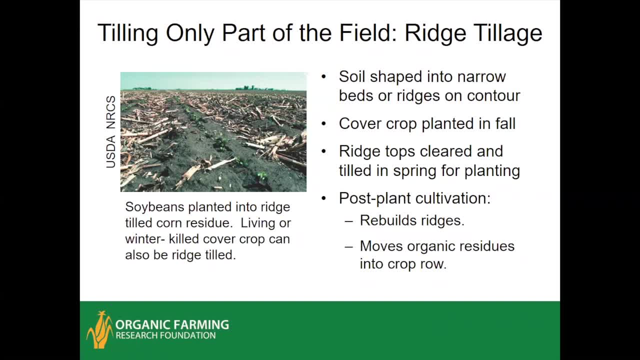 through some kind of a high-resilient tillage And then in the spring they're going to be put into a residue cultivator, which could be a sweep type of implement, And that takes weeds out and it also moves some of those residues into the rows. So you're moving organic nutrients. 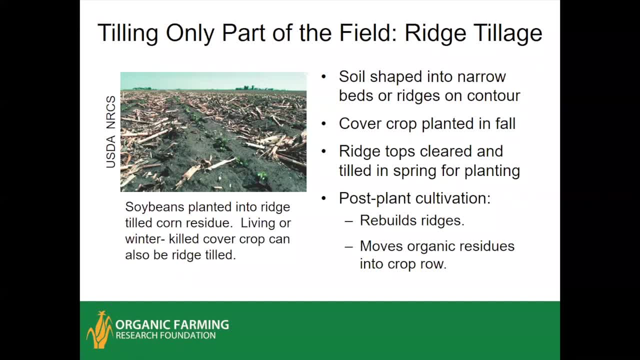 basically back into the crop row And the studies by this, Williams and others. it was published in Agriculture Ecosystems and the Environment. They'll be listed in the supplemental notes. They looked at the several parameters. They looked at the soil biological activity and verified that you increased the important function. 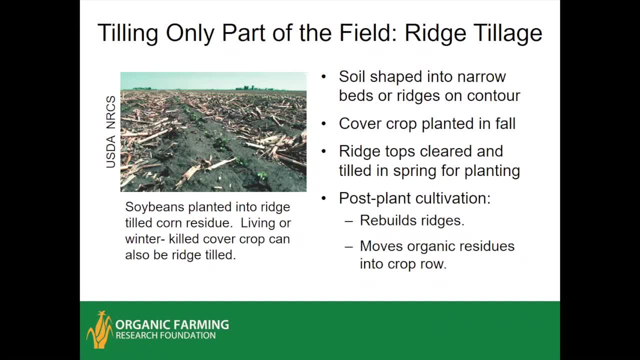 of nutrient release in the row and the equally important functions of carbon sequestration and stabilization, and also basically conserving the soil, leaving the soil mostly undisturbed between the rows. Okay, So rotational no-till. many of you may be familiar with this procedure, so I'll go. 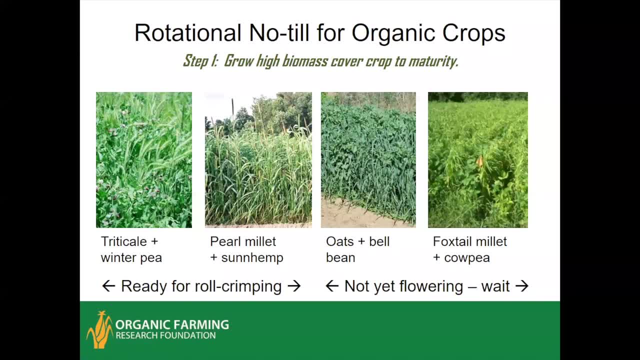 through this fairly quickly. Basically, the first step is you got to grow a really high biomass cover crop and you need to grow it to maturity. All of these crops that you see are high biomass in that they have three tons or more of dry weight biomass per acre above ground and probably half again as much below ground. 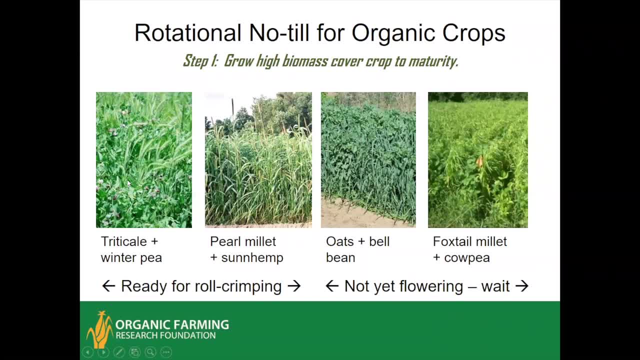 These two on the left are actually up around five tons per acre and they are also in full bloom- full to late bloom. You want the rye to be shedding pollen- In this case it's triticale- but The cereal grain should be either in the process or finished shedding pollen. 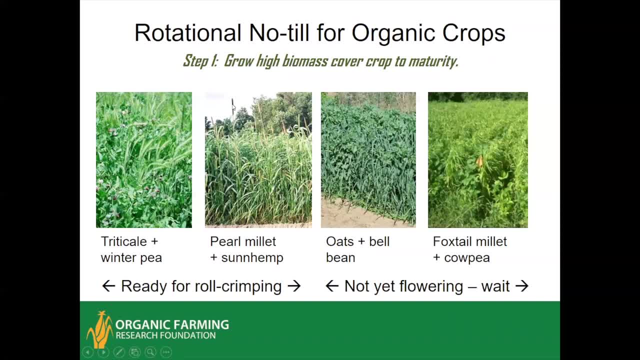 Here's pearl millet, also in that stage of full to late bloom. You can see the heads there. There is some sun hemp there. It's also blooming Over here. they're not quite flowering yet. The oats and the bell beans are still in the vegetative state. 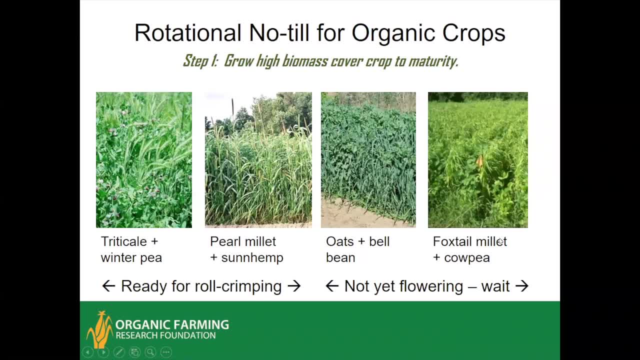 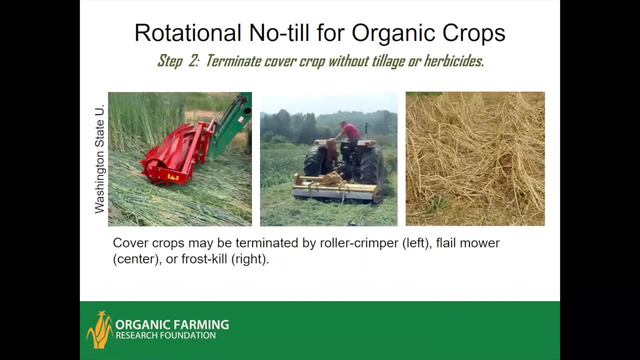 and the same with the foxtail millet and the cowpea. So they need another couple of weeks there before they're ready to be terminated with a roller crimper or a mower. So the second step in this rotational no-till system is: a lot of people are now. 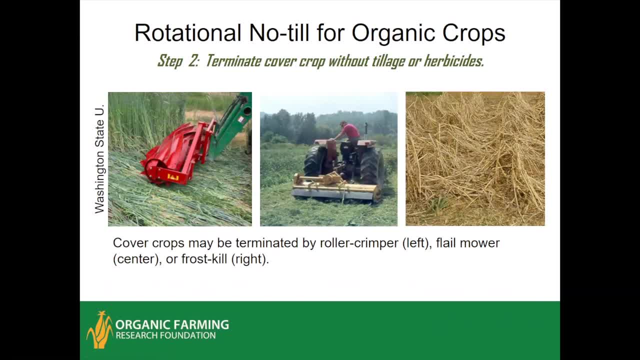 by now familiar with the roller crimper. Another way is to go through with a flail mower, which needs a fairly evenly distributed residue. There are both advantages and disadvantages to the flail mower approach, in that the weeds will grow a little faster through that than through a roll crimp. 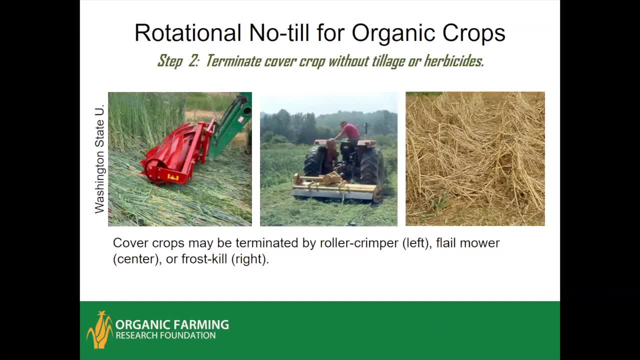 because the residue breaks down a little faster. However, if you do have weeds come up, it's easier to get in with a high-residue cultivator in the more finely divided residue than to go through that roll crimp field. Another way is to grow a cover crop that's going to winter kill. 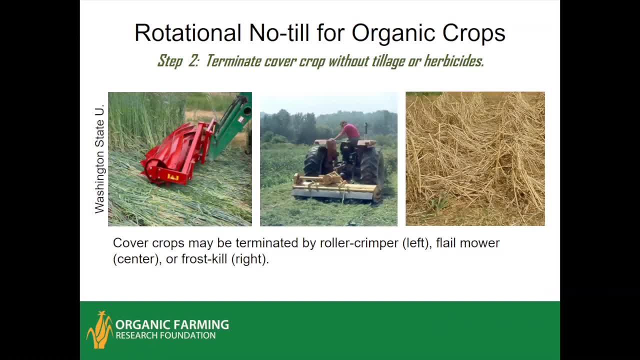 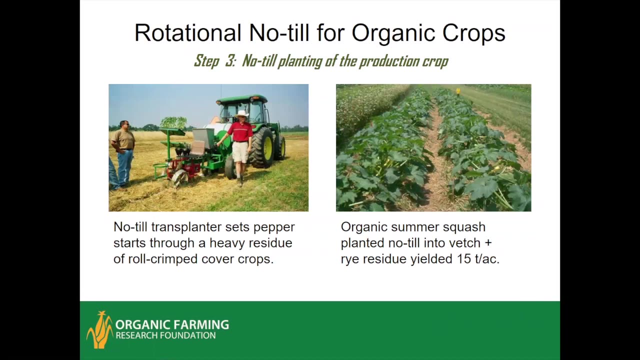 in preparation for an early spring planting. This is pearl millet that has winter killed. It dies out at about 28, 30 degrees Fahrenheit. Third step is no-till planting of the production crop on a really small scale. You can do it by hand or you can go through with something called a no-till planting aid. 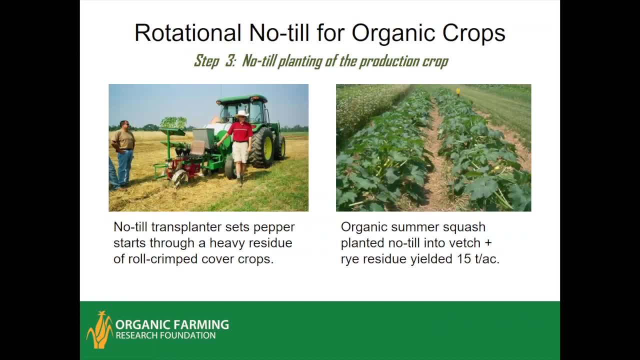 that just buries. It basically works up a very narrow strip parts, the residues, works up the soil with a shank and then a finishing implement. But over here is a no-till transplant that was developed at Virginia Tech and is now being used in various places around the country. 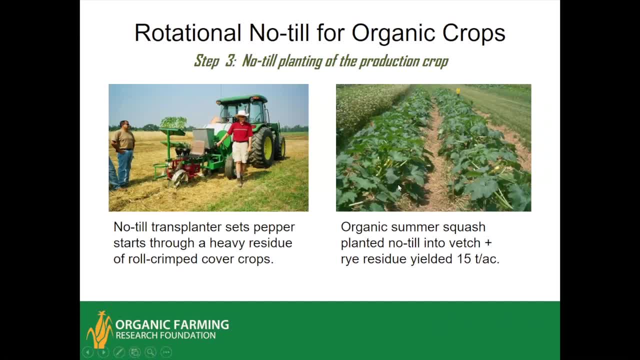 Here's some organic summer squash. that was planted no-till into vetch and rye. that was roll crimped and it's doing very well. You can see a few perennial weeds but way behind the crop It's a little bit of a no-till. 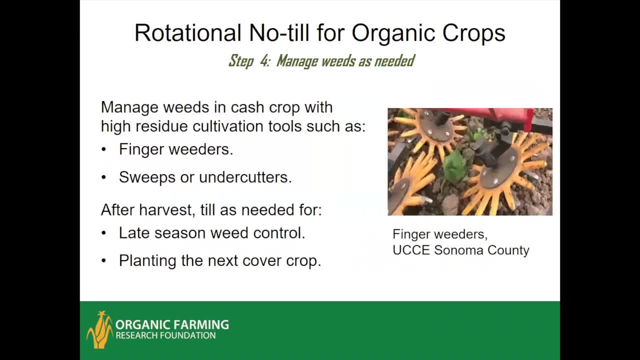 It yielded 15 tons per acre. Fourth step: you do have to manage weeds as needed. The finger weeders are pretty good in high residue. They're much better than the very lightweight torsion weeders and tine weeders. They just tend to get tangled up in those residues. 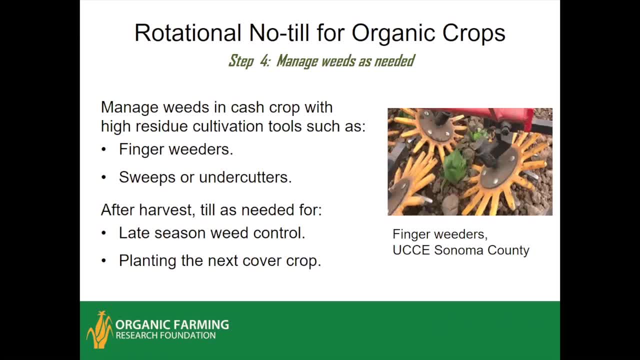 I also mentioned that there are undercutter tools as well that can take out weeds And then, after you're done with the production crop, very often you need some late season weed control. You can also do some tillage to plant the next cover crop. 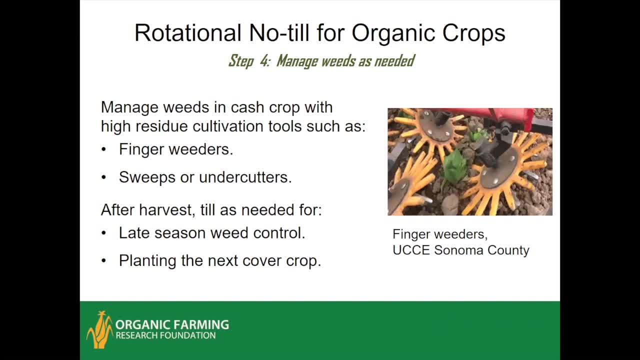 This is why this is rotational no-till. You don't really anticipate eliminating all tillage. In the best case scenario, you probably could get away with a fairly light tillage, a shallow tillage or something, and get the next cover crop planted. 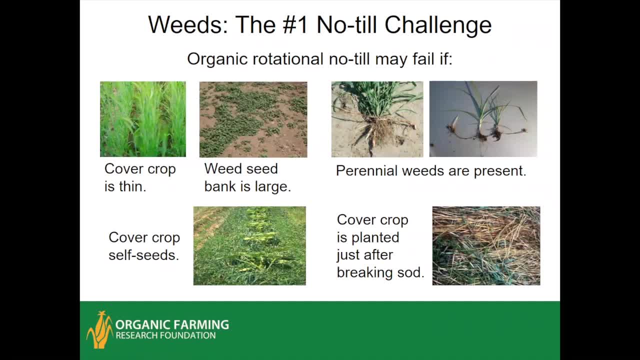 Weeds are the number one challenge in all these rotational organic no-till systems. If your cover crop is even a little bit thin, I mean that's pretty decent. but you could see it at the Triticale Here was planted in a rose and because of lower soil fertility. 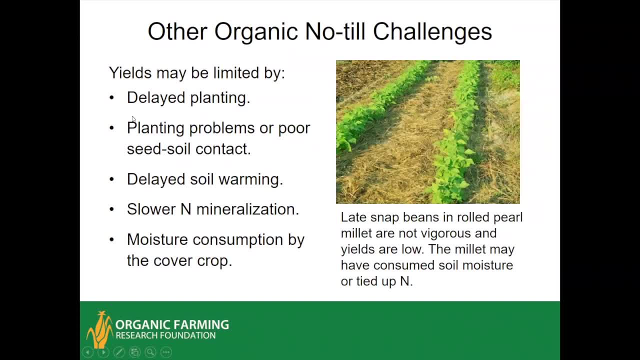 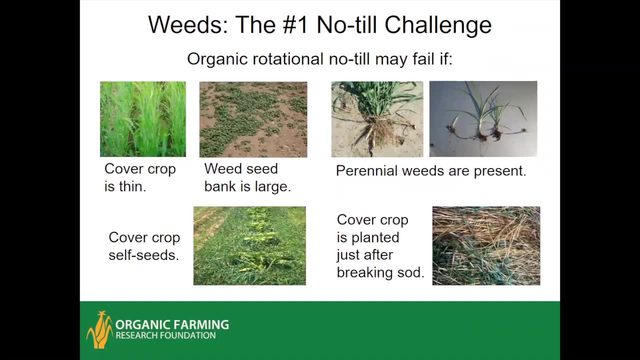 you have about two tons of biomass and you can see the ground between the rows. Oops, I think I accidentally advanced. Let's see if I can go back. Thank you, So the weeds are going to start growing there and when you roll crimp they'll be ready to take off. 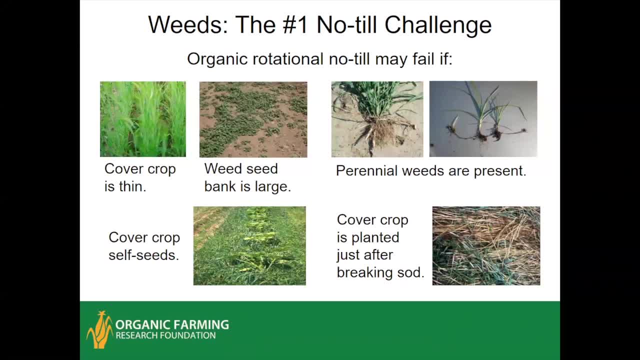 Another thing: if you have annual weeds, you've got lots of them, You've got a really big weed seed bank, Like if you till up a little piece of ground and it looks like that a week later you will have too much weed pressure usually for it to be successful with this system. 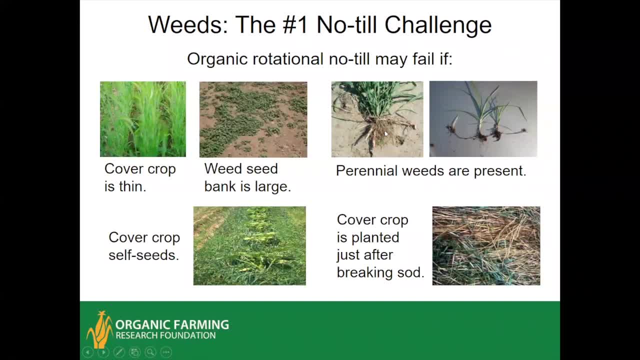 And if perennial weeds are present to any significant degree- Johnson grass. this is yellow nut sedge. other examples are the bindweed and the Canada thistle we saw earlier. they will make this system pretty impractical. Another thing that can happen is if your cover crop is over mature and it sets seed. 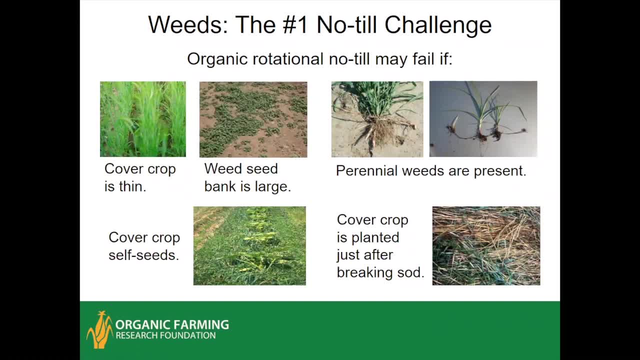 it'll come up and compete with the crop itself seeds. This was actually the same experiment, as you saw earlier, with that very successful summer squash cover crop. In this case it was barley and crimson clover, both of which bloom and set seed about three weeks earlier than the rye and the hairy vetch. 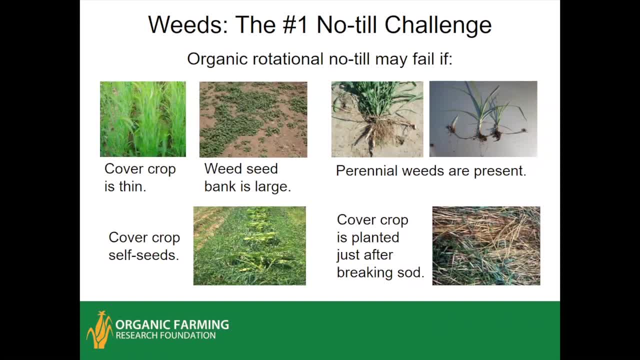 They were rolled in the same day and they self seeded like crazy and the squash having a very hard time. Another thing that can happen is if you plant the cover crop right after breaking sod, after coming out of a sod phase in the rotation, and that is one challenge. 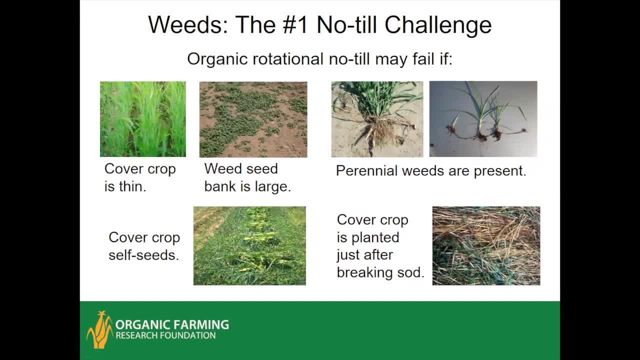 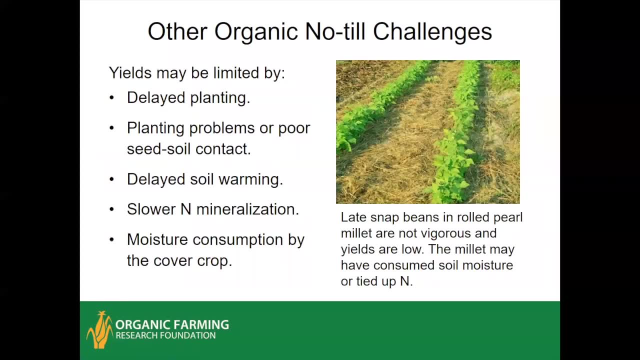 which, with that system, if you then roll cut that very next cover crop, very often there is enough of the sod left to come up and create a problem. Few other challenges when you're doing organic rotational- you're doing any kind of rotative no-till with a high residue. 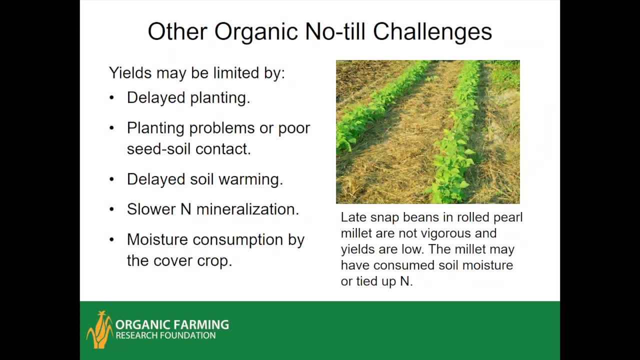 you may have delayed planting. the soil is cooler and wetter takes longer to get ready. You're going to have planting problems, poor seed, soil contact. that's a matter of um having longer planting cycles, and then you know. 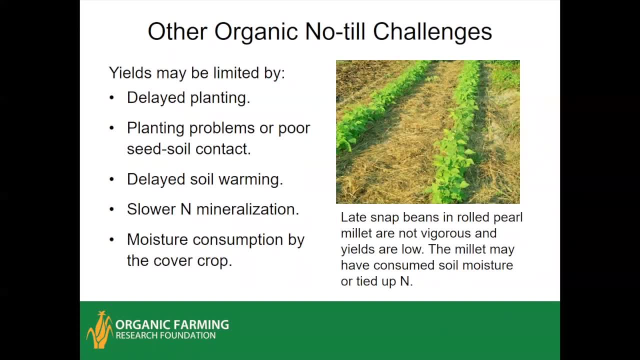 the right tools for planting through thick residue and ensuring good seed soil contact. If soil warming is delayed, this can be a problem, especially in northern regions. It'll slow down the establishment of the crop. It also slows nitrogen mineralization because you haven't 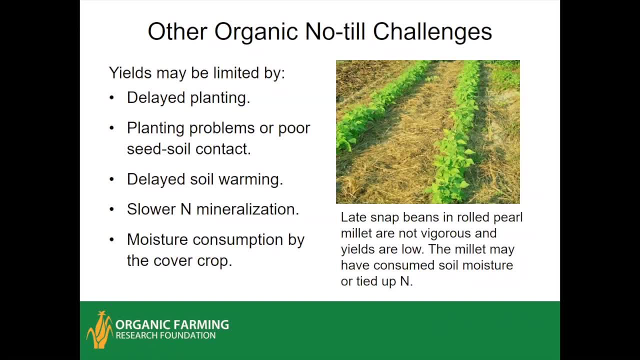 stirred up the soil, You've left it completely undisturbed, And if your soil health is excellent and your temperatures are warm enough, it could work out quite well. But one thing that's happened is, in the north central region, these organic rotational no-till systems. they'll look great. 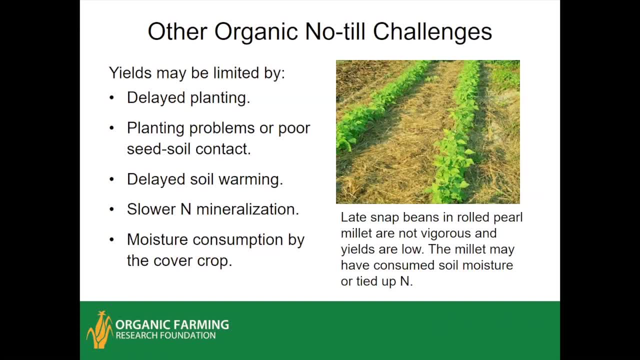 in terms of soil health. And yet the moisture, excuse me, the slow warming and the slow nitrogen mineralization can cut soybean yields even by a third and corn yields are often cut by two-thirds. Another issue in lower rainfall regions is moisture concentration. So if you have a lot of moisture in your soil, you're going to have a lot of. 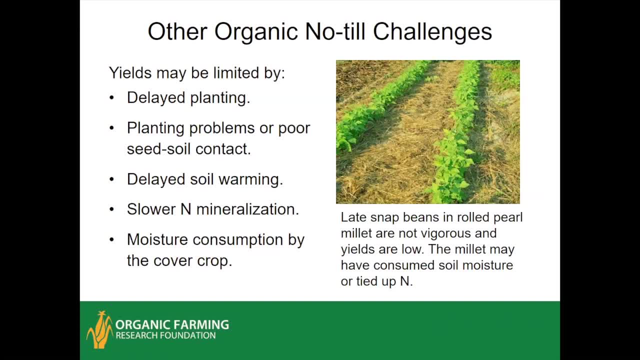 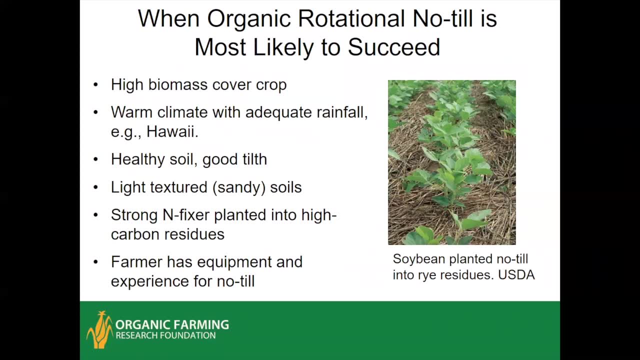 moisture in your soil. So if you have a lot of moisture in your soil you're going to have a lot of consumption by the cover crop prior to the cash crop planting. So there are situations where organic rotational no-till is likely to succeed. 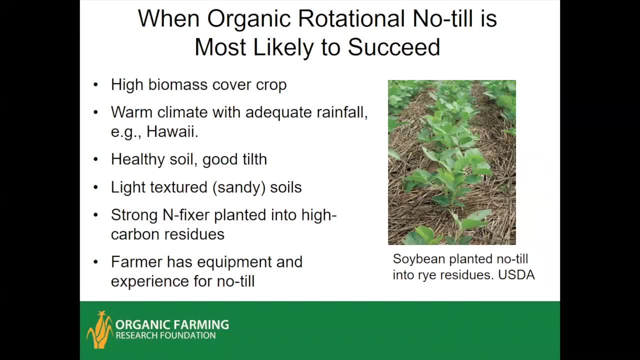 As I mentioned before, you need that high biomass cover crop that really evenly covers the ground Warmer climates. the southern United States, from California all the way over to Florida and the Carolinas and Virginia, parts of Virginia, our growing season is long enough and our climate is. 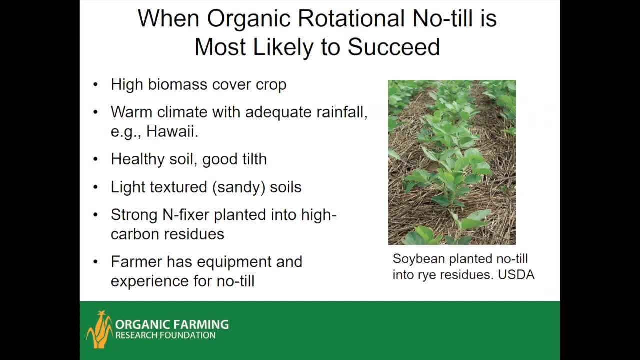 warm enough that there is time to grow a fully mature cover crop and to establish the cash crop and the soil cooling may not be as much of a problem. can't even be an advantage. There's one example of a study that was done: some studies in Maryland, some in Iowa and some 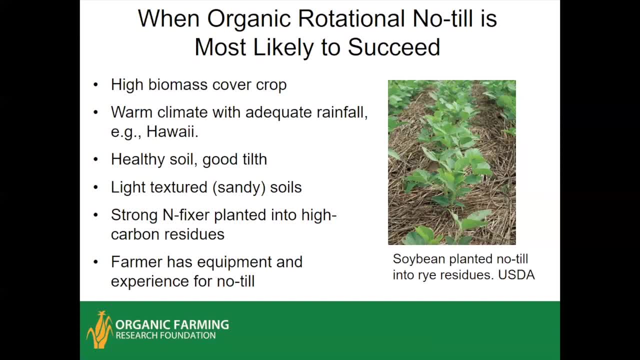 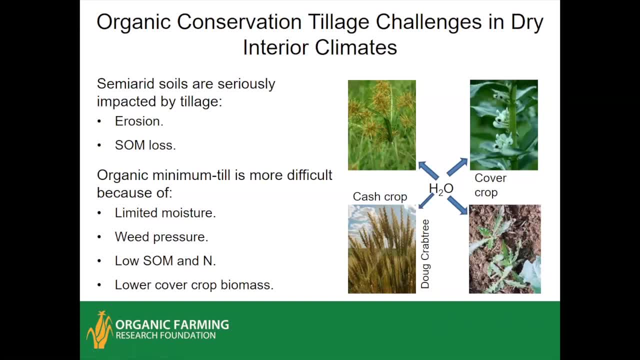 So when you have good soil health, it's in good tilth. that generally supports the no-till system. So when you have good soil health, it's in good tilth. that generally supports the no-till system. matter is not that high to begin with and the impacts of the soil organic matter loss. 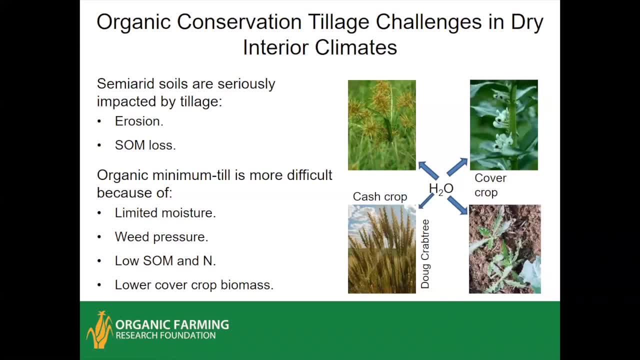 after tillage is especially severe And because of this limited moisture, organic minimum till organic no-till systems are more difficult to implement successfully, and the weed pressure itself is one of the major concerns. Also, it's harder to get enough cover crop biomass. 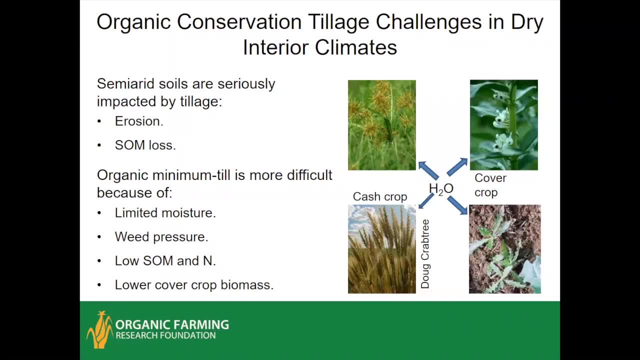 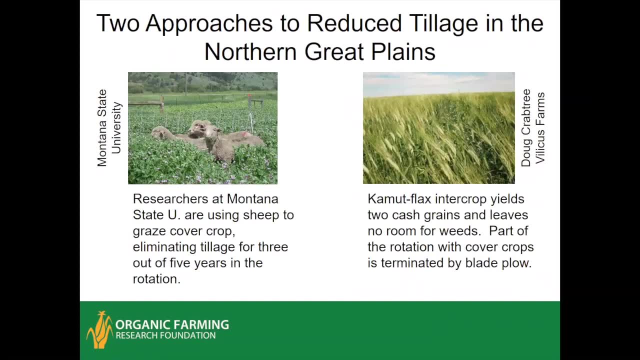 to achieve the kind of surface mulch you need for a minimum till system to work. So two approaches to these challenges. in dryland production. Researchers at Montana State have been looking at a five-year crop rotation and they diversified the rotation so that there's 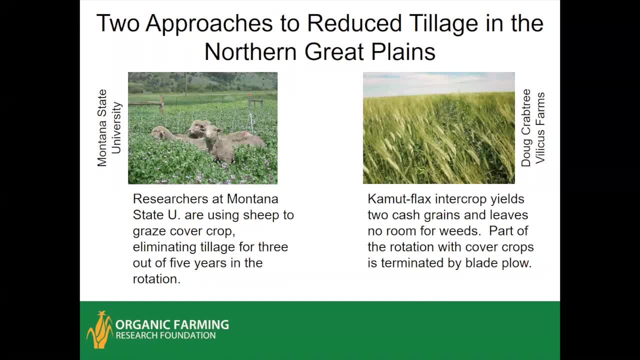 sweet clover lentils, a couple of different kinds of cereal grains, rather than just doing the wheat fallow. And then they thought: well, what if we use sheet grazing rather than tillage to terminate the sweet clover ahead of the next cereal grain? They're working on fine-tuning that system. They had some. 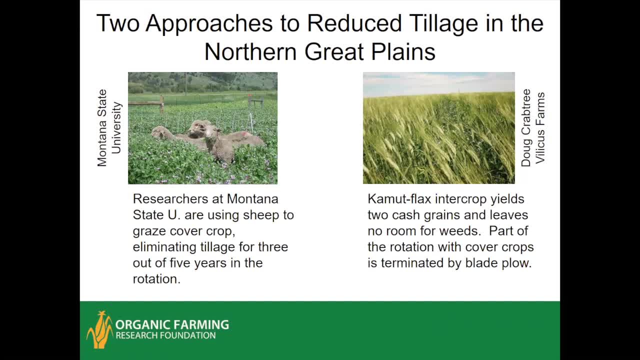 mixed results with it, some yield sacrifices. But I also want to again mention Villicus Farms, Doug and Anna Crabtree. This is an actual biculture cash crop. They're growing a mixture of kamut or corazon wheat and flax, both of which are marketable grains, And they are able to thresh those together. 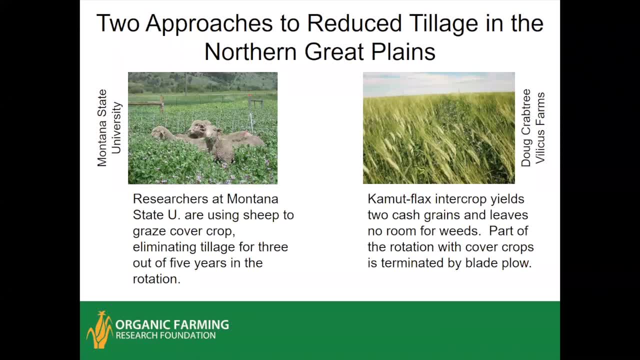 and they separate very easily. It's a relatively easy process. They separate on the farm and sell them as two cash crops And you can see there's really no room for the weeds with those two crops growing together And they have developed rotations of five to seven years in length. 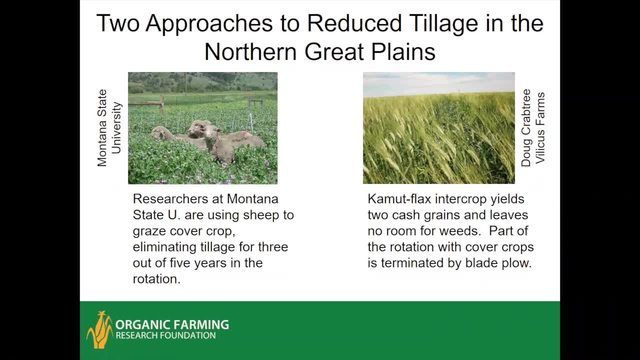 using a total of 10 different species of cover crop and 15 different species of kamut, And they're able to thresh those together. and they're able to thresh those together and they're able to thresh those together and they're able to separate from. 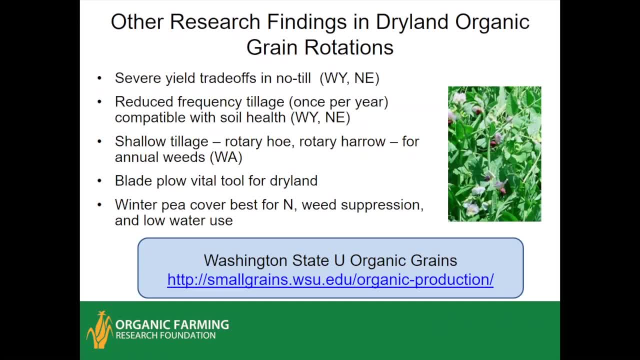 the sleep on them. There's an observation on画 of lentil trade-offs because of the dryness And, for instance, in Wyoming Nebraska. also, it's a short growing season, relatively cool weather. However, systems where they reduce the frequency 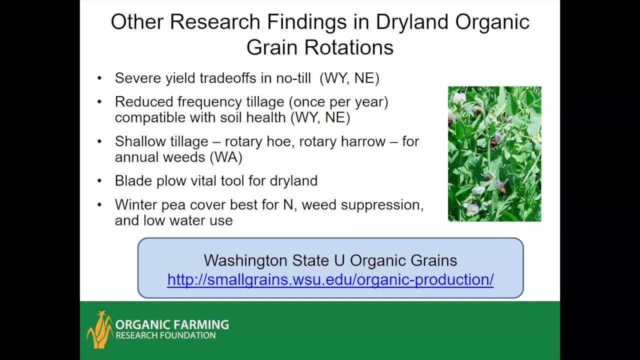 of tillage. just get it down to once per year and then use some of these tools that reduce the impacts of tillage, such as the rotary hoe, rotary harrow or the blade plow. All of those strategies significantly improve soil health and minimize the adverse effects of the tillage. 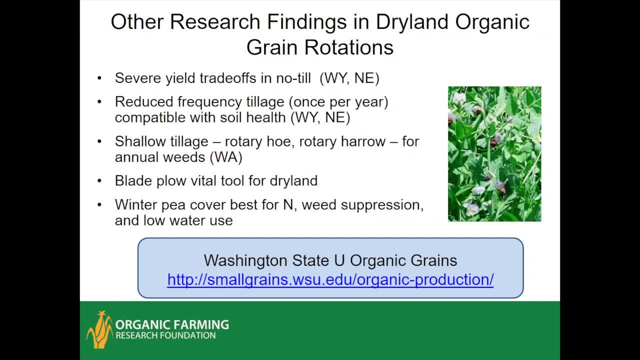 operations on the soil. One thing that several studies that OREI, the USDA organic program, funded organic research programs, have funded is that the winter pea- here's Austrian winter pea, grown during the winter as a green manure, has been working best in terms of providing some 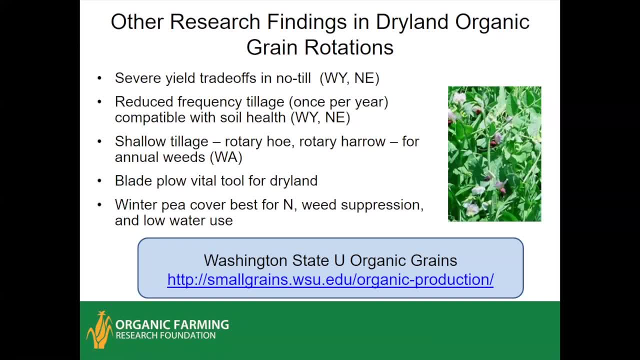 nitrogen For the next cash crop, suppressing weeds and doing so with relatively low water use. And that's another thing. some cover crops utilize a lot more moisture than others. Pearl, millet and barley are light users of moisture, even though they're very drought. 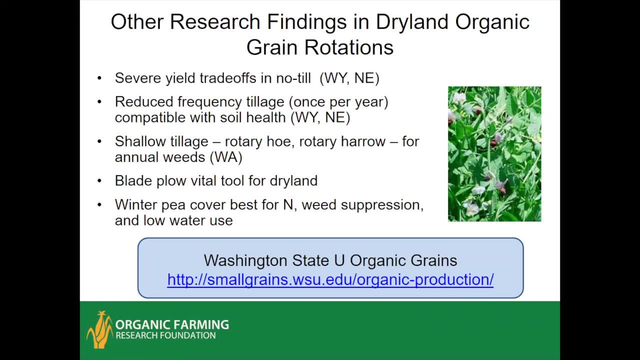 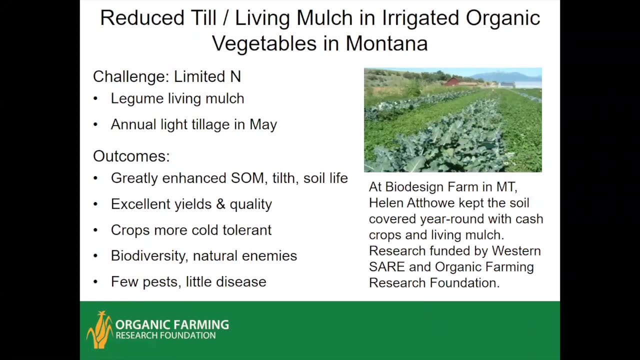 tolerant, whereas some other drought tolerant species, such as alfalfa, are very heavy moisture users and can really leave the soil profile depleted. So that's another thing to consider in developing a rotation for a reduced till system. So just very, very quickly touch on an example of vegetables that are grown with irrigation in a dry region. 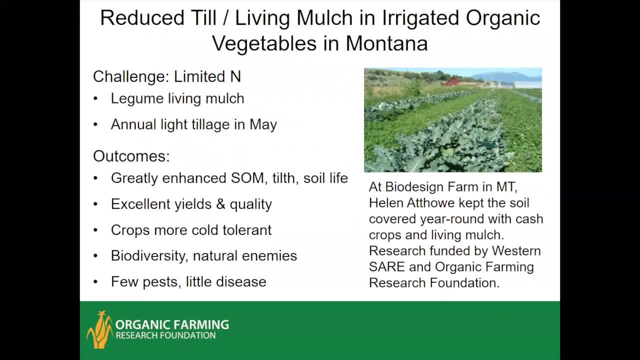 This is in Montana. Helen Athow has been developing and evolving these systems for several decades. She's worked as a consultant and as a farmer and as a conservationist for many years. The challenge that she found for growing here's broccoli- again a very heavy nitrogen feeder. 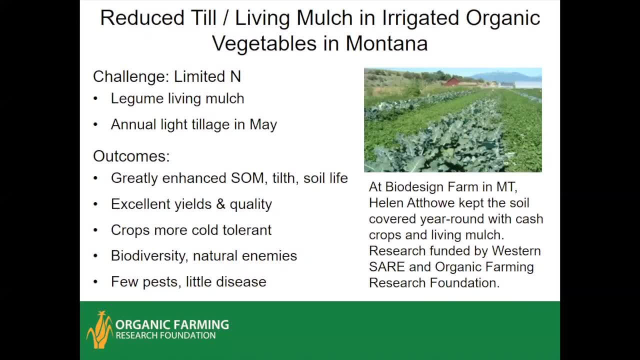 the challenge was limiting limited nitrogen, So she developed systems that were based on a legume living mulch that was tilled once a year, relatively shallow and light in May, just enough to set it back and get her cash crop planted, And then, by either self-seeding or by reseeding the alley, she gets to cover the living mulch. 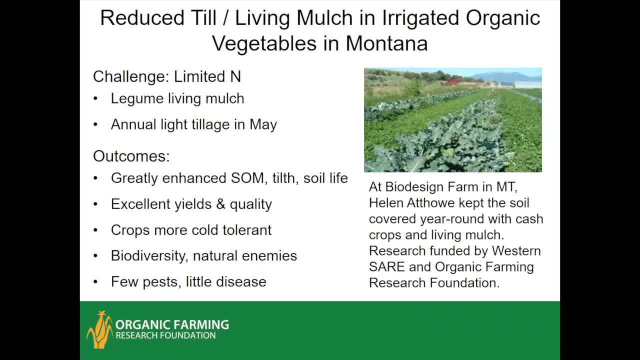 reestablished And some of the outcomes she had is that this system really built up soil life and and soil organic matter and overall tilth, overall soil health. She had excellent yields and quality found. the crops were more cold, tolerant, had fewer pests and less disease. 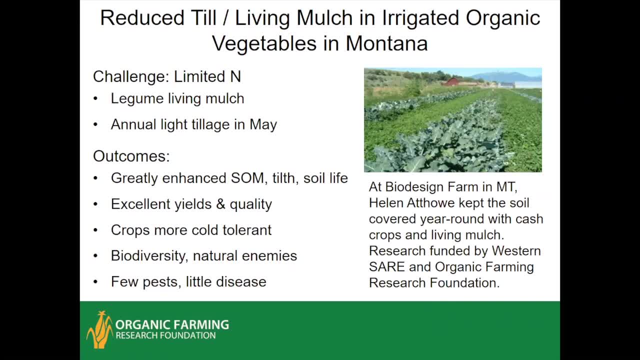 A lot because this kind of system- you're keeping the ground covered and in multiple different kinds of crops, builds a biodiversity and supports natural enemies. She wanted me to emphasize that her research was funded by the Western SARE program and also by the Organic 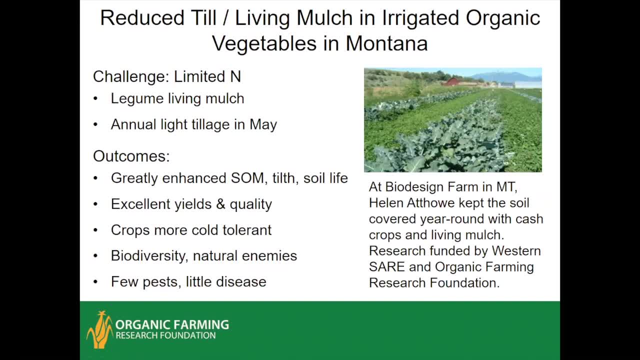 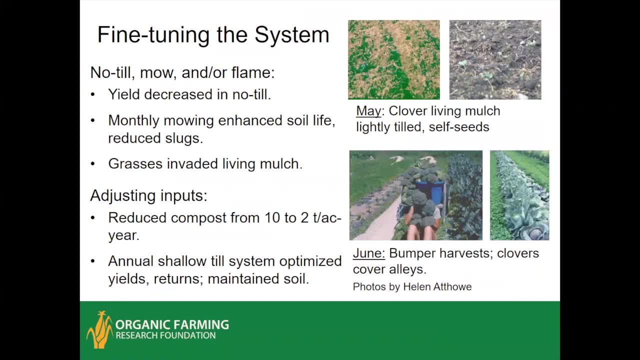 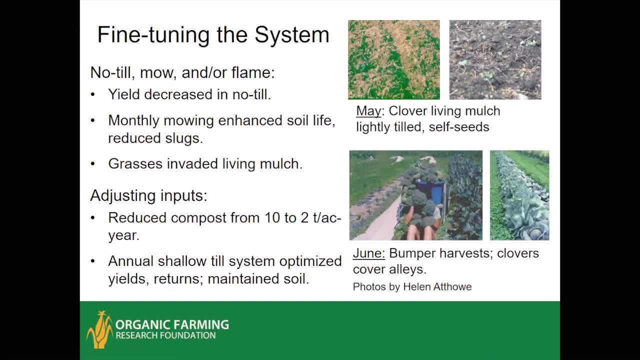 Somehow, when you mow that grass and then let it regrow, there's even more root exudates and root deposition into the soil profile. It's somewhat analogous to management-intensive rotational grazing. She also found that because the soil is so healthy, she could reduce the amount of compost from 10 tons per acre down to two tons per acre annually, To big cost savings. it also avoids building up excess phosphorus. You can see the kind of bumper crop she's getting out of that. It was the cabbage on the right, broccoli on the left. 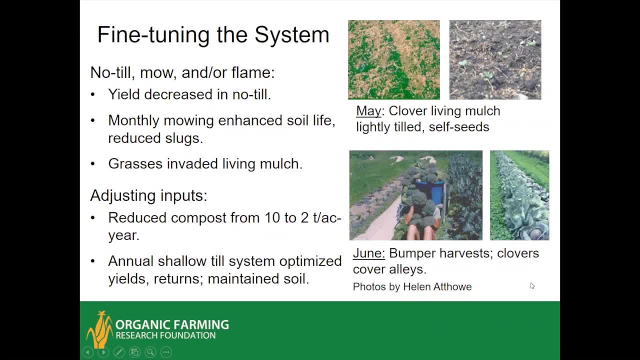 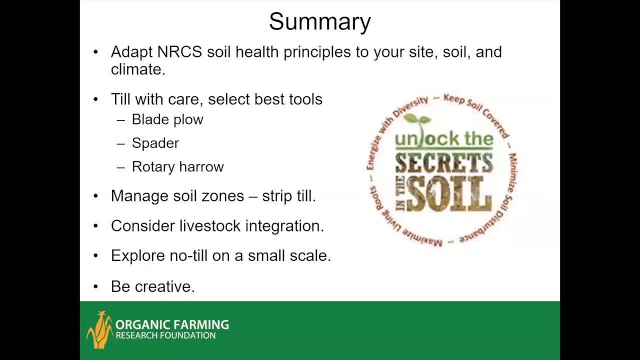 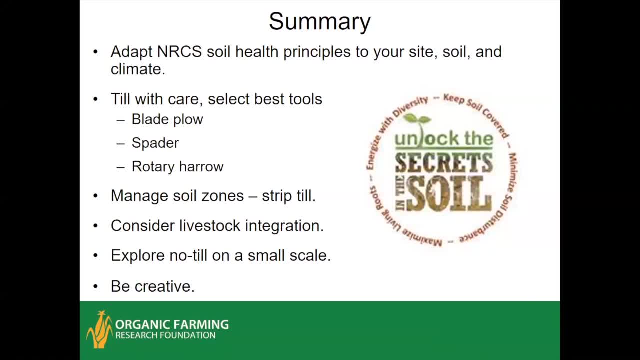 important one. It's a very important one. It's a very important one, It's a very important one. And a fifth one, offered by Gabe Brown of North Dakota, which is to integrate livestock into the system when you can. You want to use those as a starting point and then adapt them to your 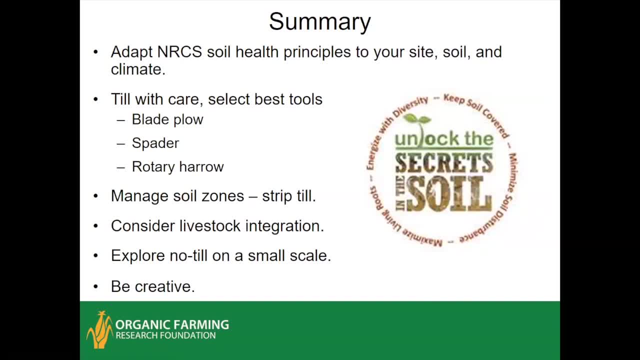 particular climate, soil and site and production system. Till with care, just like the best tools. There's a few examples there that we've talked about. Consider the soil zone management, the strip-till system. Consider livestock integration when it's appropriate to your enterprise mix. 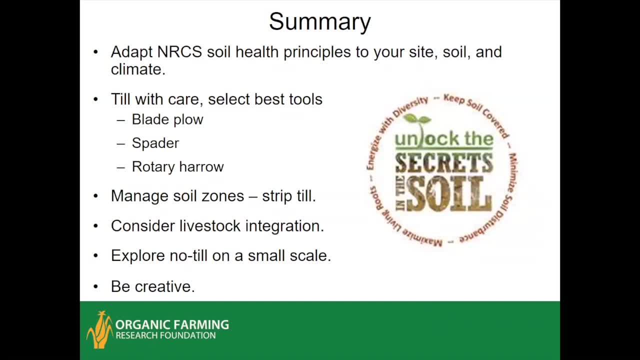 Now I would say: explore no-till on a small scale to begin with And, as always, be creative. You know, it's like I will not be able to tell you how to do a minimum-till organic farming, especially when it's not in my region. 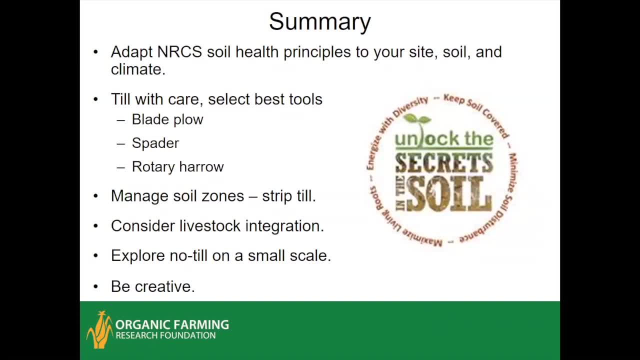 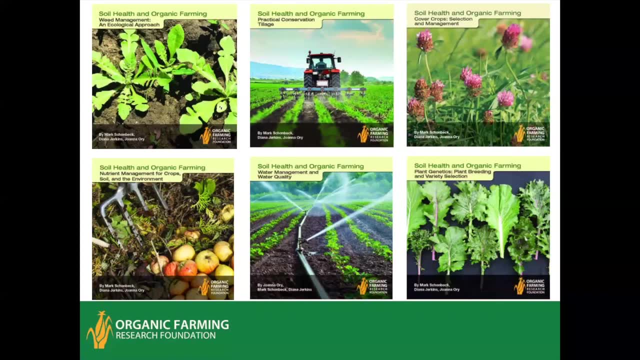 So I'm now open to questions, Thank you. Okay, Thank you, Mark. These are the other soil health guides that are offered through Organic Farming Research Foundation. They're newer ones on climate and on risk management through improving soil health, So watch for those. 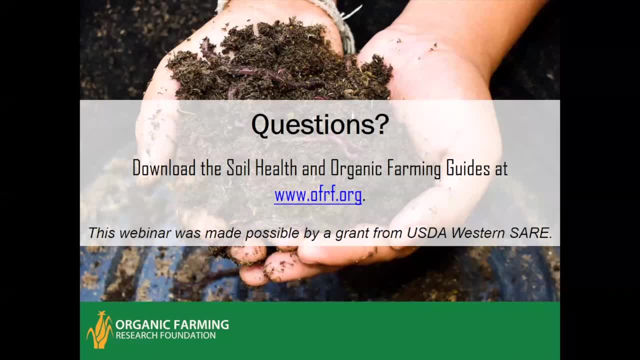 And we're now ready for questions. Okay, Thanks, Mark. We're going to start our question and answer period And we see some questions coming in already, But if you have another question, this is a great opportunity to ask Mark, And you can just type it into the Q&A box on your screen. 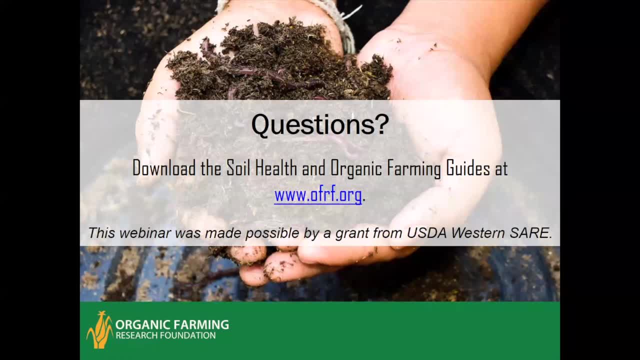 And we'll be reading the questions out loud for the next 30 minutes Until we run out of time. So if you don't see the Q&A box, there should be a bar with some controls at the bottom of your screen. If you click on the Q&A one, that will pull it up. 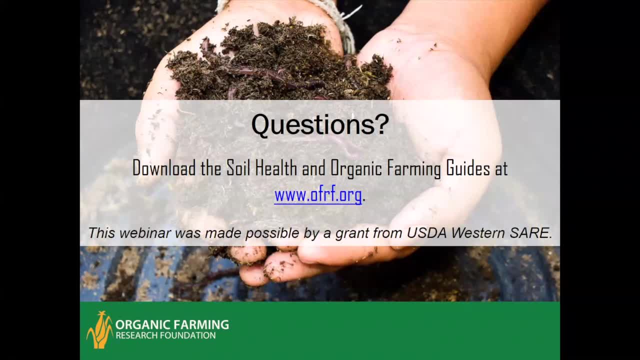 So I also just want to mention, before we start the Q&A, that this presentation is being recorded And you'll be able to find the recording in about a week or two on the eOrganic YouTube channel, along with all the other webinars in the series. 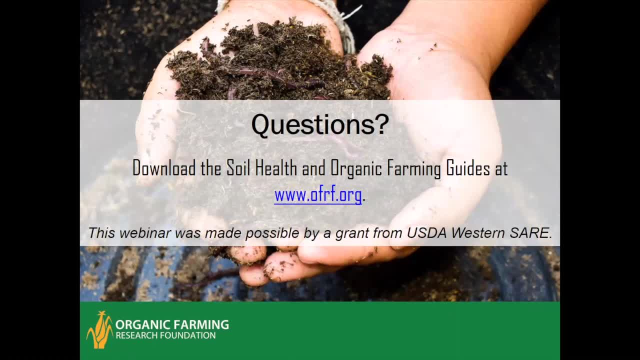 And I'll be putting up a couple more links on your screen which have a link to where you can find all those recordings, And then the presentation notes which Mark prepared, which has a lot more information than he was able to have time to give on this webinar. 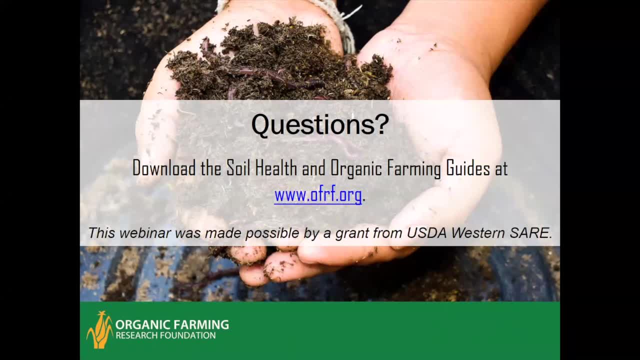 And the slides are there as well, So I'll just pull that up in a second after we get started with the questions. So we had one person who wanted to know whether you have any tips for soil health practices for tree fruit orchards and berry plantings. 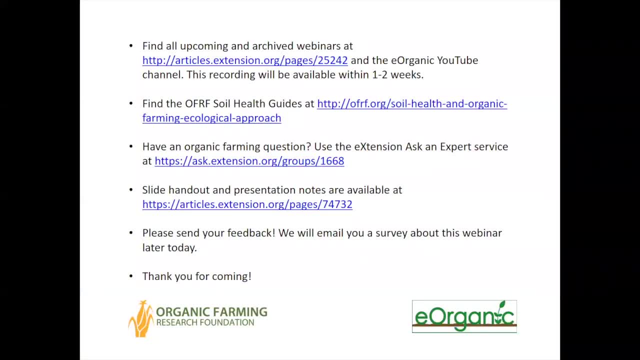 Ah, yeah, Yeah, good question. It's pretty clear that keeping the orchard floor covered as much as practical makes a huge difference to soil health. We actually did a couple of I go into that more in the water management webinar which will be presented for the Western Region later this year. 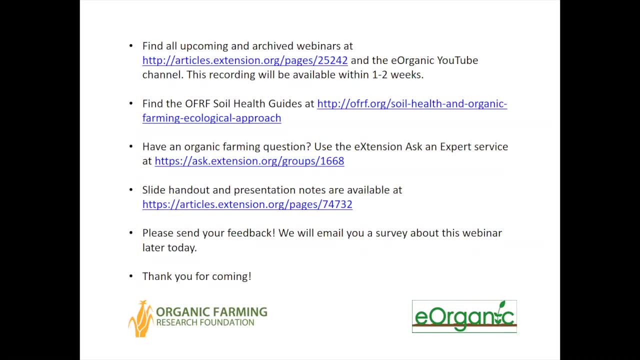 I did one for the Heller webinar series. that was just general, not specific to region. But there have been a couple of reports comparing soil organic matter levels and water use by the crop in either tilled or herbicide fallow versus keeping the soil, the alleys and the orchard floor covered in perennial vegetation. 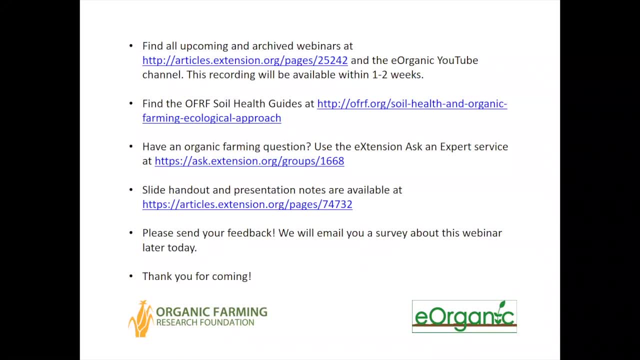 And organic matter levels were basically cut by half by doing the bare fallow, whether by chemical or by technology. So I think that the What we can do is we can get those ones to the back of the orchard with a lot more water. 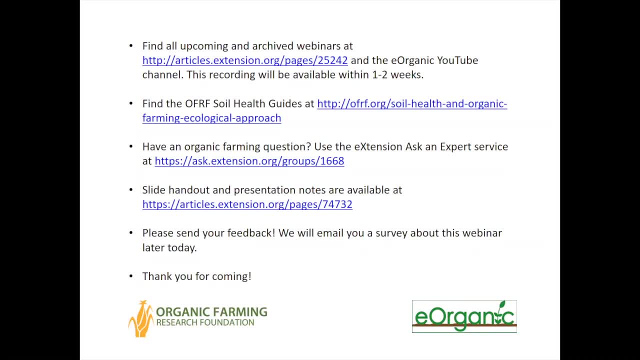 And in Utah, which is very dry region, water consumption by the Living mulch system in the orchard floor was about the same as with the bear soil, but tree health during tree establishment was much better because you had — they were using nitrogen fixing legumes and bird's foot tree foil in the alleys and then using a shallow rooted, self-seeding annual alyssum right under the trees. 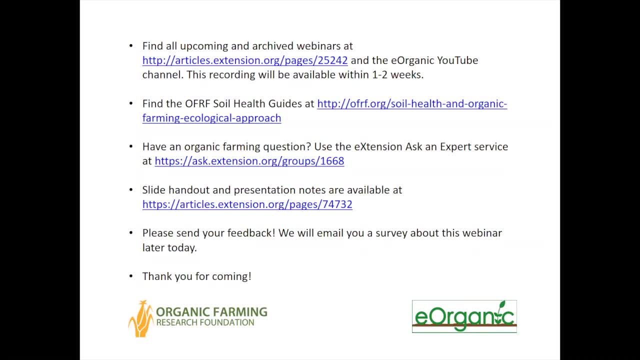 and then using a shallow rooted self-seeding annual alyssum right under the trees, and then using a shallow rooted self-seeding annual alyssum right under the trees trees so they wouldn't compete too much for moisture. that system sustained much better soil. 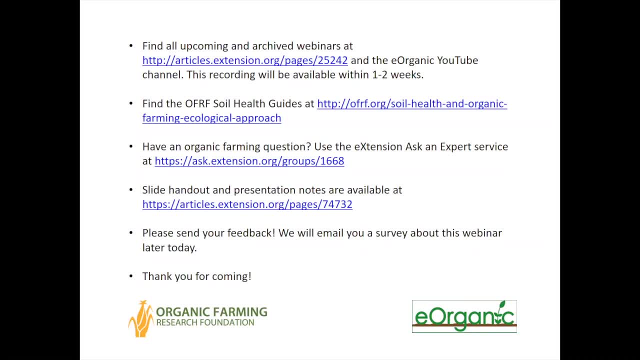 and tree health. uh. so i would say: when you're doing a perennial crop, get away from tillage as fast as you can. and another thing is during the crop establishment. one way to control weeds right in the crop row is to use weed mat or landscape fabric. it's not as kind to the soil. 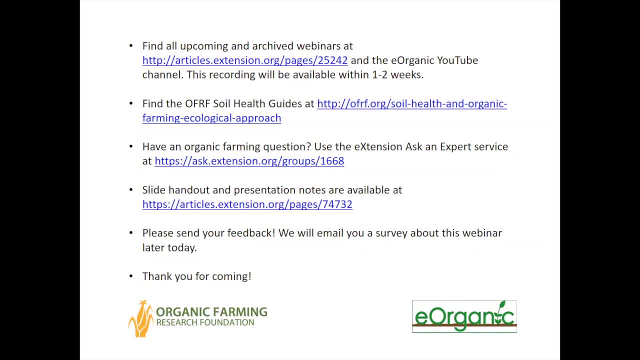 quite as an organic mulch or a living mulch. however, it will really keep the weeds down and it will prevent competition with the young establishing crop. once your crop is well established, probably you could just go with a continuous cover. okay, let's see this. listener is west of the cascades in western washington and farmers here claim that they must. 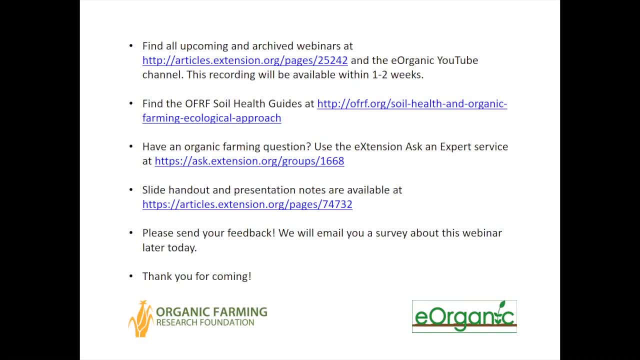 till to dry up their weeds out wet soils for timely planting, and most of them are seed crop farmers who grow spinach, beet and potatoes. What reduced tillage methods might work for these farmers on our floodplain silt loam soils? Really good question, especially since I'm 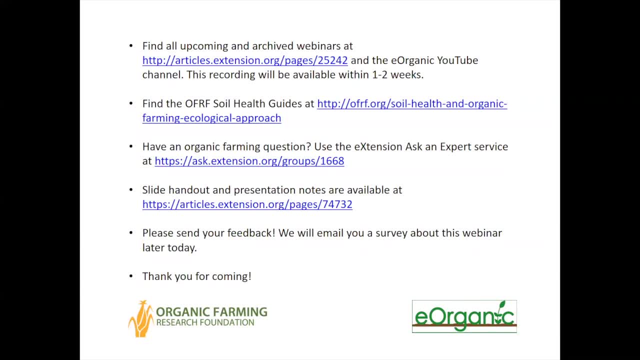 quite well aware of the soil type effect on the results of that trial in that same region. with the squash, I would go with a spader because it's relatively gentle on soil aggregates. It goes deep but does not compact. It breaks compaction Depending upon the crop you're. 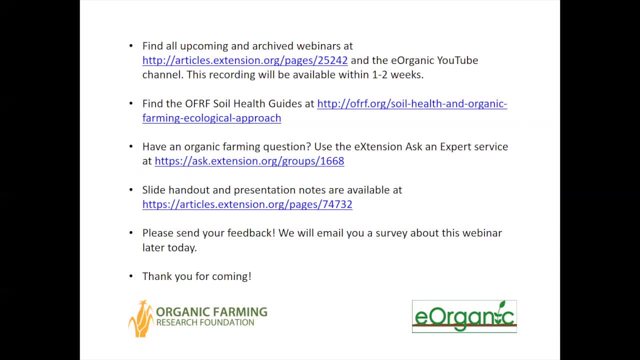 growing. you might be able to use winter cover crops to draw out excess moisture If you're planting potatoes. I don't know for sure, but I would think that in that part of the world the summer would not be too bad, Too hot for potatoes. You could plant a winter cover crop that will draw some of that moisture out. 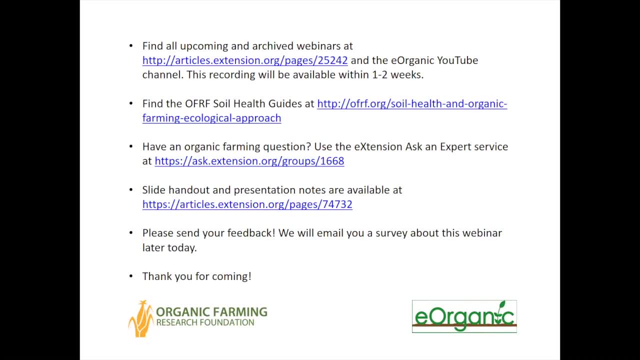 and then terminate it and perhaps use the spader or maybe look into strip till if conditions are warm enough For really early crops like spinach. I know there's an early spring crop. you got to get the soil warmed up for that. I think that is one of the most challenging aspects. 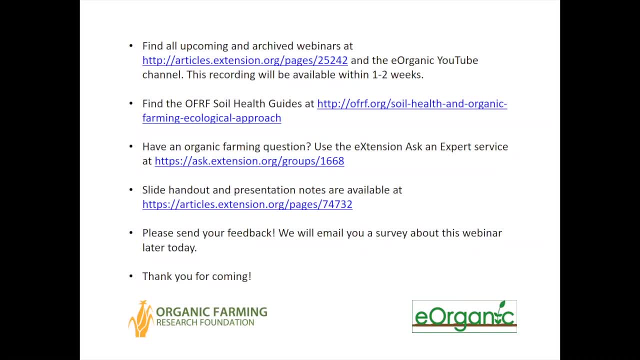 but again, keep an eye on the evolving, emerging tillage technologies. There are new tools coming out all the time that ease up on the soil damage. If you've got a rototiller and that's all you've got, I would say look into increasing tractor speed and gearing down the PTO so that you're. 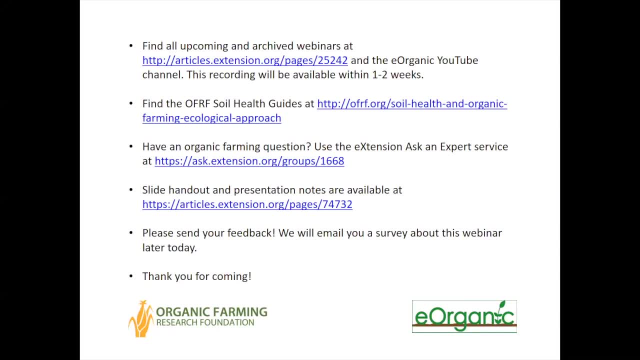 gently turning the soil and not beating the heck out of it? Is there a benefit of roll crimping a cover crop versus cutting the soil? I think that's a good question. I think that's a good question. Yeah, the roll crimping, it orients the residues so it's easier to run some of the no-till planters. 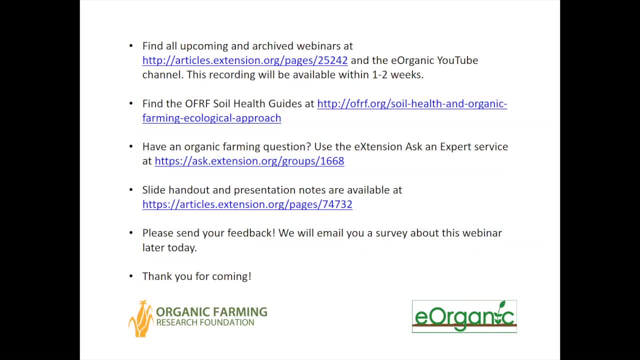 and transplanters through that oriented road. You'd have to drive in the same direction that you roll crimped. It also gives a longer period of weed suppression. On the other hand, if you have enough weed pressure that you know you're going to have to do some weeding operations, you might 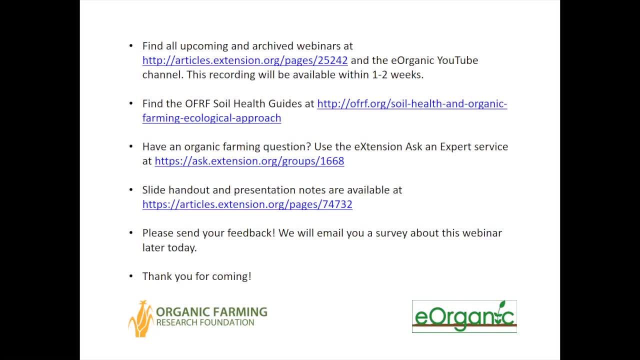 instead need to go ahead and mow flail mow so you got finely chopped and evenly distributed residues and then use a high residue cultivator- Okay. The same person asked: we've been experimenting with no-till and we've had some. 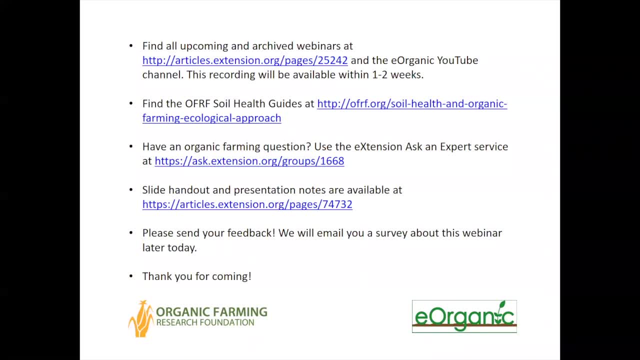 serious wire worm issues? Have there been studies of increased soil pests with no-till? I do remember some of the studies that have been done Every spring. the first thing that we examine is our soil quality. They have. we have no last year, So we have no last year. But again, if you have, 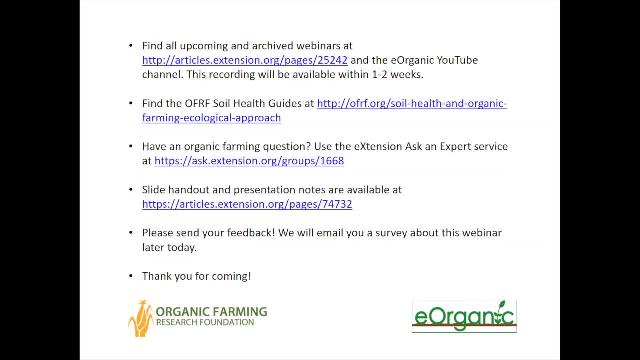 I do remember slugs being a big issue on Cape Cod. when I did my very first organic no-till experiments back in the late 1980s, I had not heard of wireworm. I am aware that that tends to increase with high residue, so I'm wondering if it would be any less if you spaded in the residue. 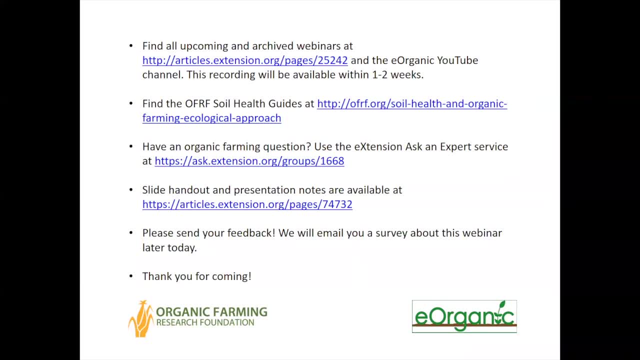 Maybe a trick would be to grow a cover crop that winter kills, or to grow a lower residue crop right in your row so that you could do some kind of a strip or ridge till or something or a row cleaner that cleans the residue out from right around where your crop is. 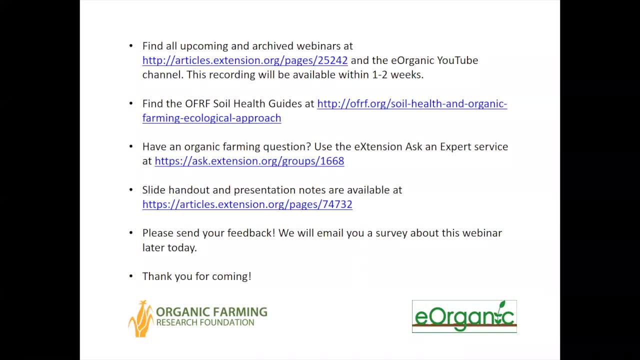 If this is wireworm on potato, that's an issue of the wireworm coming in. It's a good question about soil food. I'm not really that familiar with wireworm. I'll have to make a note of it. There may well be studies that show that, but I know that slugs are an issue. 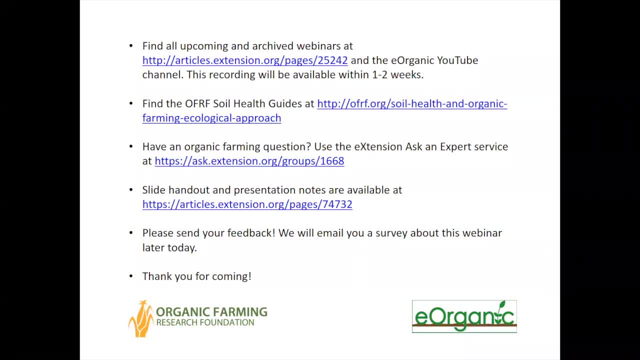 What are some solutions to slow nitrogen mineralization in no-till vegetable production, Especially with strip tillage? That's a good question. One general finding is that the more your soil health has been enhanced, the greater the nitrogen mineralization potential will be, even under a grass legume cover crop mix. 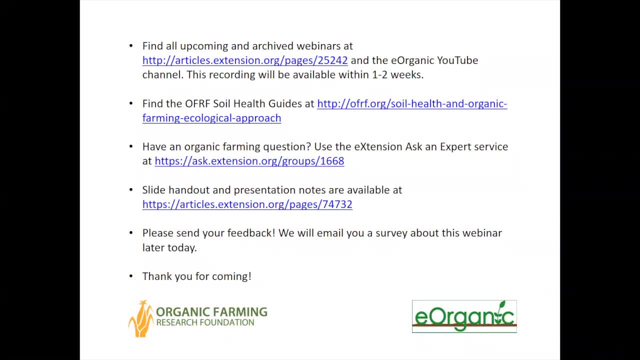 If your nitrogen mineralization is slow and you're strip tilled, you might do zone planting of cover crops, like planting a legume or a crucifer, like tillage radish in your crop row. and of course, if you're growing, if you're growing brassica vegetables, you'll want to use the legume. You don't want to use a crucifer. you know a radish. 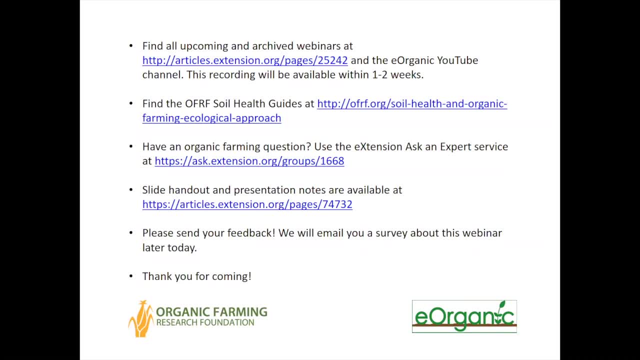 So probably you're going to want to grow, you know, the high legume cover crop and then in the alleys maybe a grass cover crop that will tend to keep the nitrogen down. in between, If you're really having trouble with nitrogen limitation, you could do in-row strip fertilization, fertigation or, you know, just side dress a little bit of feather meal. 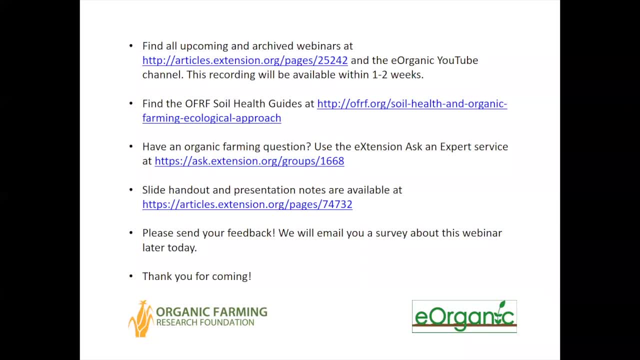 A number of strategies for just providing more nitrogen. but in the long term, the more you can build up the soil food web and soil health, the more that nitrogen is going to be in your crop, So that nitrogen mineralization should improve. Okay, here's a comment. One significant problem we've seen with weed mats in orchard production systems is the creation of a hospitable environment for rodents such as gophers and bulls. 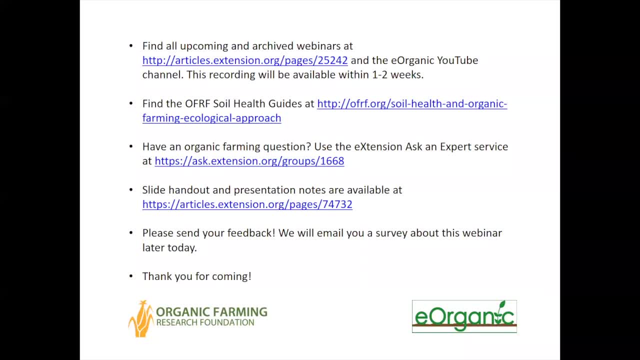 Bulls have been seen in the central San Joaquin Valley to destroy an organic orchard almost before any detection. Please bear this in mind when using weed mats, especially in young orchards. So thank you for that comment. Okay, And then another comment on the wire worms that it came and ate broccoli roots. 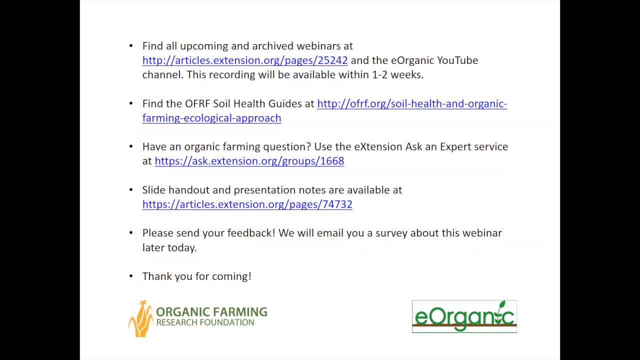 Wire worm ate broccoli roots. Wow, Okay. so next question: Do you have any tips for using these methods in a flood irrigated organic raisin vineyard which is in a dry region of California? Uh huh, I don't have not right off the top of my head, but I want to make a note of it. 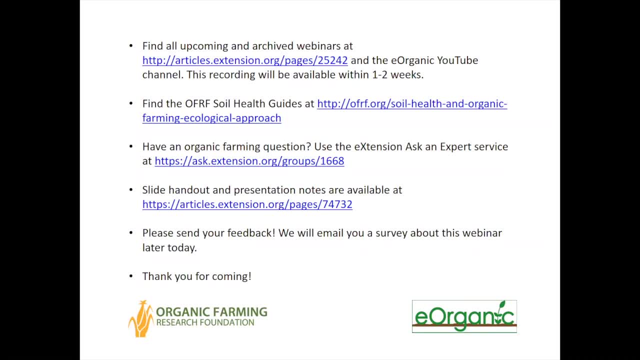 Flood irrigated raisin vineyard. Again, you'll probably want to try to get the whole soil area covered. I mean, you would probably want to find some living mulch that can tolerate the higher moisture for part. you know the brief periods of flooding that that are in there. 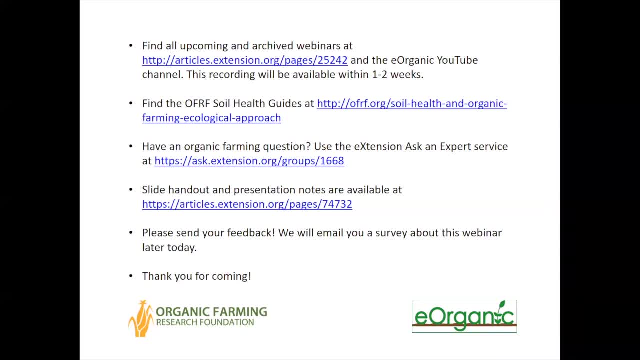 Okay, That is pretty much what we can be entailed in that irrigation approach. Okay, So do you have any recommendations for Alaska growers? Mm, That is a real challenge because she had the extremely short growing season there. I guess I would lean towards. Well, two things that have been helpful in the north central region. One is overseeding the cover crop into 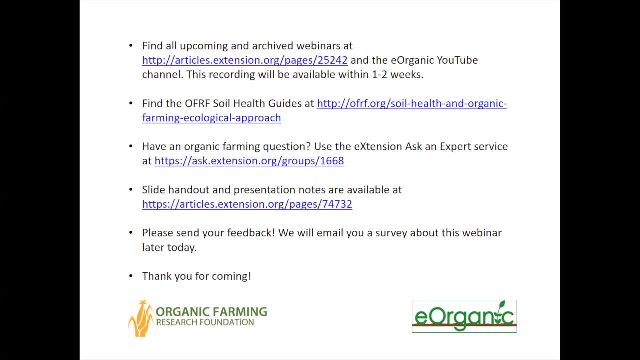 standing cash crop and if you're going to have to get in really quick in the spring, think in terms of growing a cover crop that has winter killed. I have to admit, I have very little experience of applying these to it in Alaska. Okay, what resources might you suggest for cover? 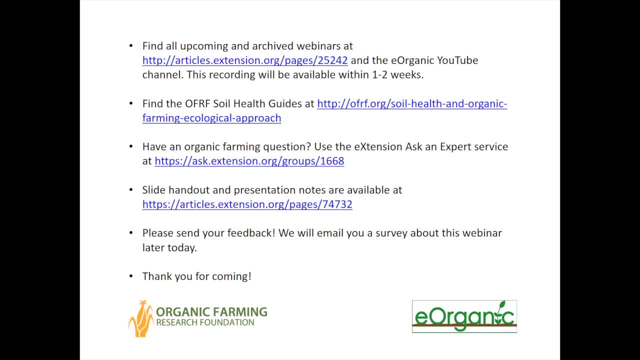 crop mixes, especially mixes with- let's see, more than does, I think, the- I'm just trying to read this- more than eight types. I would go to NRCS If this person is from Montana or even a neighborhood or North Dakota. I mean, Gabe Brown has worked. 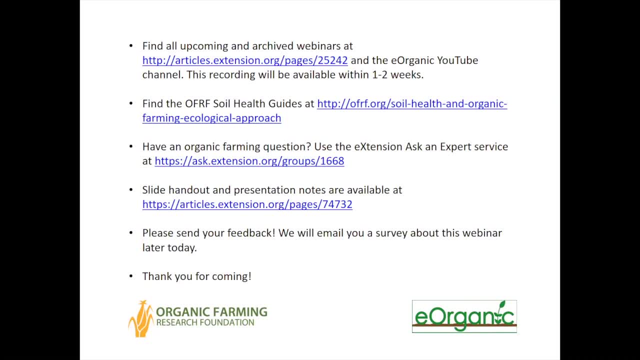 with them. Now he's not an organic grower but he uses very minimal amounts of water. Just reading his book Dirt to Soil, there's a lot for all of us to learn from that. He did take the conservation ag approach of first eliminate tillage and then phase down and phase out as much as practical the synthetic inputs, and he's come a long way. doesn't use any synthetic fertilizers anymore. He uses these very highly diverse multi-species cover crop mixes and has been quite successful with them. 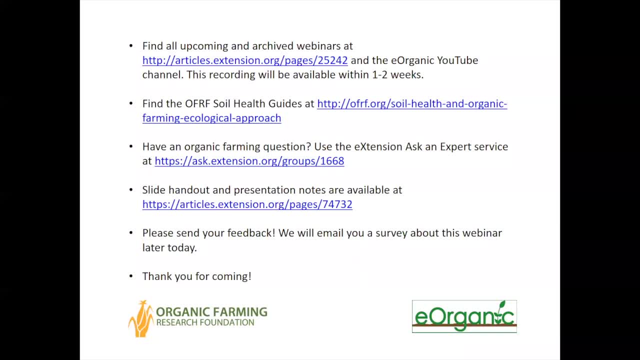 There have been more mixed results with the University of Pennsylvania, but on the other hand, I know there are growers in the eastern and central United States who have also been very successful. But I would say in my experience it's been Natural Resources Conservation Service that have really been most enthusiastic about these very high diversity mixes. 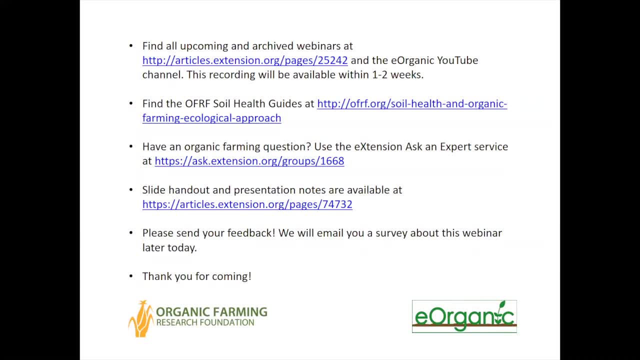 And they may be able to give you region-specific recommendations. Okay, Someone typed a comment about Gabe Brown being a good source of information and said that he has several YouTube videos. Oh great, So you might want to check those out, Okay. 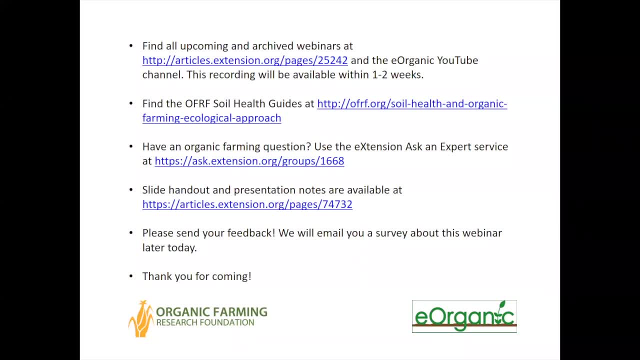 Let's see. Do you have any other recommendations on how to help manage slug populations? Well, I know there is a relatively well, it's actually not that new. it's been around for more than 10 years. It's a very low toxicity slug bait allowed in organic systems called sluggo. 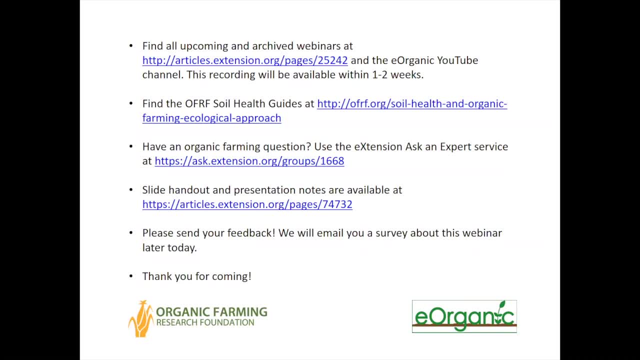 And it's basically iron phosphate in a formulation that takes your slug populations way down And it doesn't have the high toxicity of many of the other older slug baits that are out there. Larger scale, I'm not really sure. Is it like a small-scale vegetable production? 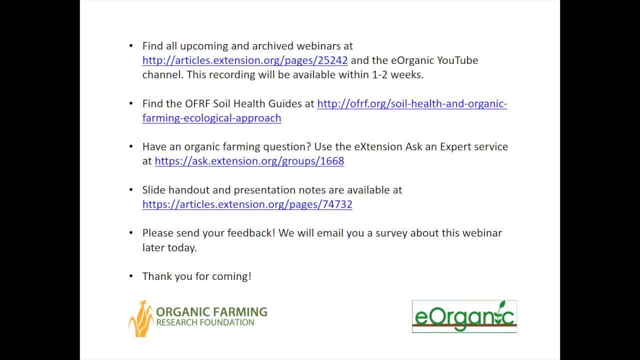 Or are we talking about slug problems in grain crops and such Okay? We aren't sure yet, But if the person has more comments on that, feel free to type that in. Yeah, But that is one product to look into if you're not working on too large a scale. 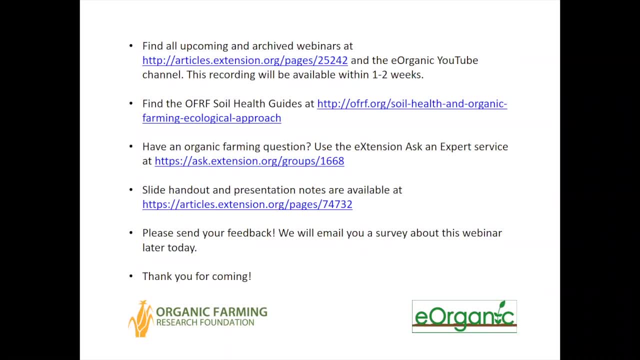 Okay, There are a couple people asking about soil testing. Do any of the soil health guides that you mentioned address soil testing? Because I know we put up some videos on our YouTube channel, on the organic YouTube channel, on some simple soil tests that you can do at home. 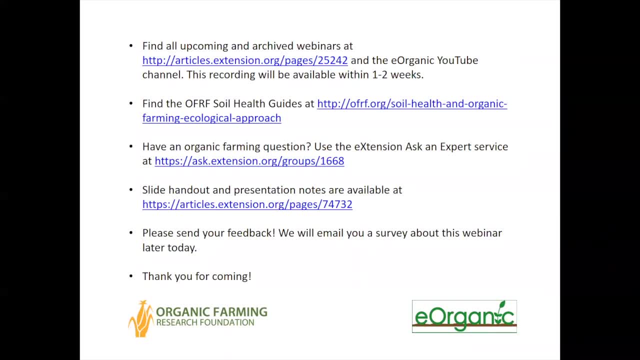 And I know we have an article on soil testing using chemical tests for organic farming, which I'll try to find right away and put in the chat. But if you have any other recommendations to learn more about soil testing, I touch on this a little bit in the nutrient management webinars. 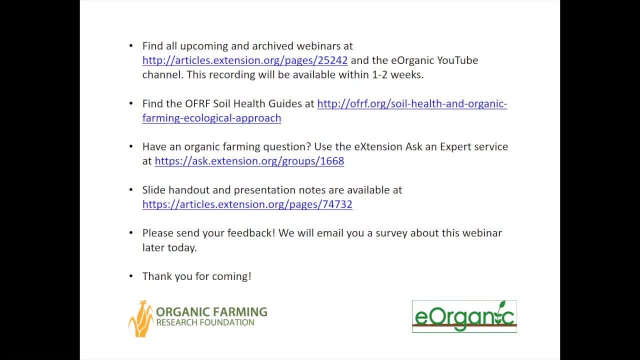 And I will also in the risk management webinar that's coming up, Because more and more they're finding that standard soil test recommendations are often recommend more than you need, That crops are not removing as much And they don't really need as much to sustain fertility. 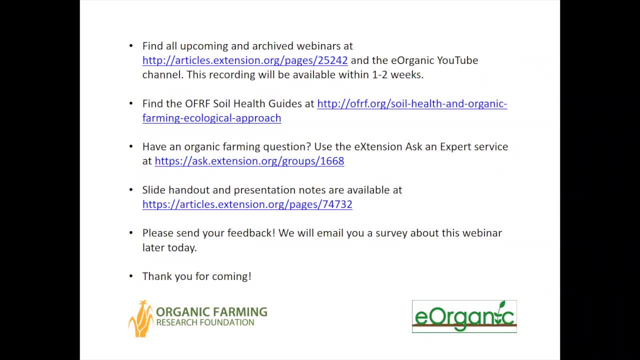 And this becomes more and more true As your soil health improves. What I keep coming back to is: you know, if you're not certain whether you're getting a return on your investment in the fertilizer? do a side-by-side trial. Say, if you're growing broccoli and you say, well, I typically put down 50 pounds of nitrogen. 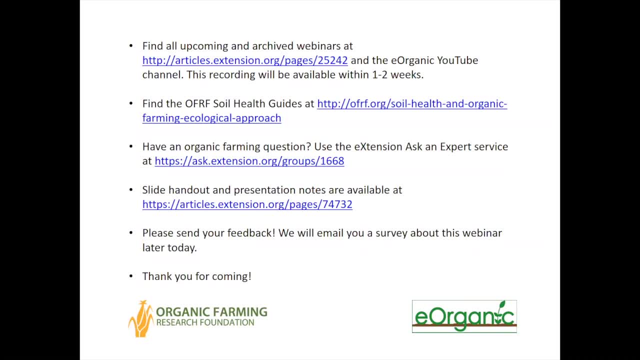 I wonder if I really need more. You could try, you know, try one row with 100 versus 50. And do that a couple years in a row, Because you may get somewhat different results year after year. And that's one approach. 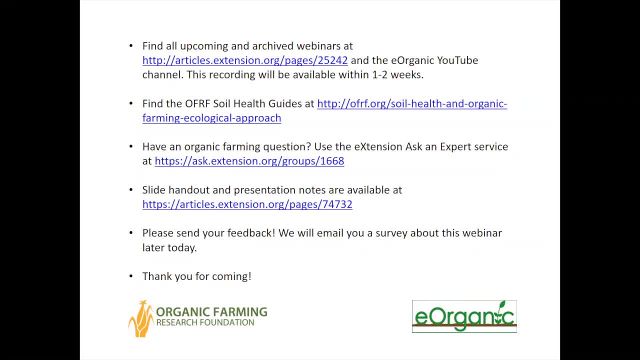 Another is to use foliar analysis, as well as soil, to make sure you're not providing nutrients you don't really need to sustain the crop. And, of course, there are more and more soil health, soil biology tests coming out In addition to total organic matter. 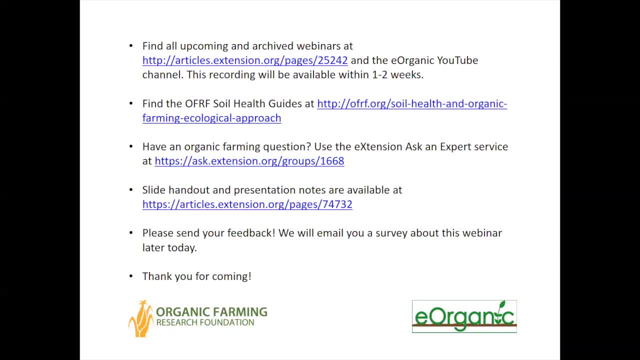 And there's active organic matter tests. There's a fairly simple soil respiration test. It does require a lab analysis, But with careful sampling and sending it to the right lab you can get that done without too much expense. This is a field that's sort of young. 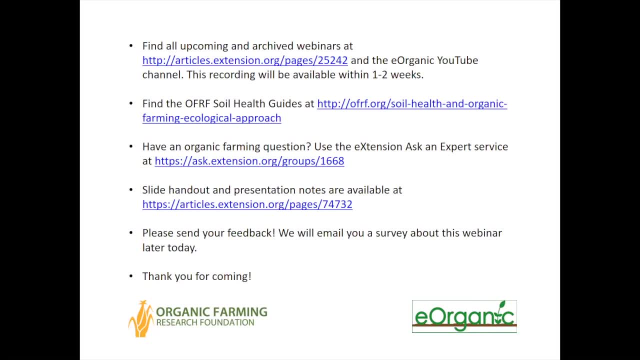 It's, you know, soil health oriented testing And in fact NRCS has just posted, Just finished a comment period the end of last year, on a draft technical note, It's like a manual describing six major measures of soil health and the laboratory procedures associated with it. 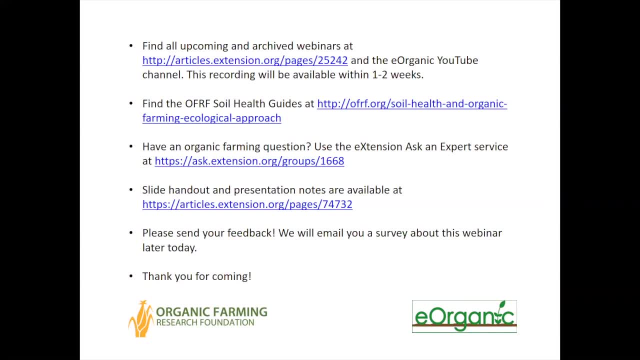 So there is the science of biological soil health testing is still young, but it is moving ahead. Okay, Let's see. Has there been research on how long it takes the soil food web to reestablish after it's been disturbed? Oh, that's a good question. 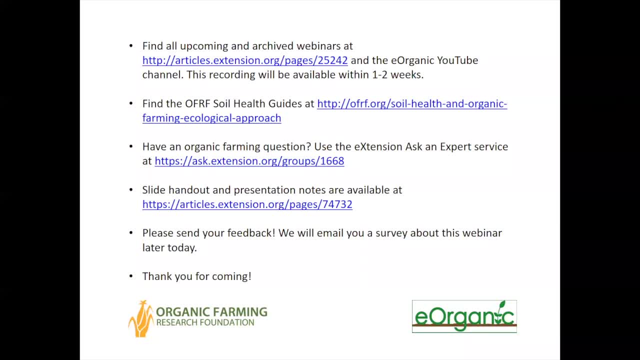 There have been some studies, I think it varies And you know again, the less frequent and less intense the disturbance, the more it will tend to bounce back pretty quickly. For instance, one type of disturbance is soil solarization. You're just creating intense heating that kills off a lot of the weeds and the pathogens. 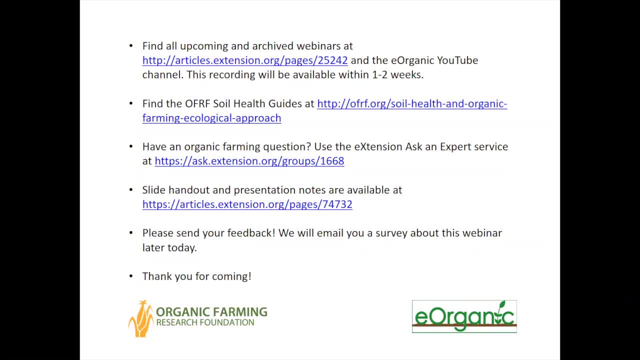 And what has been found is that in general the beneficial organisms of the soil food web will tend to go dormant. They'll just kind of take cover during that time And then they'll gradually recover over a few weeks. That is a good question. 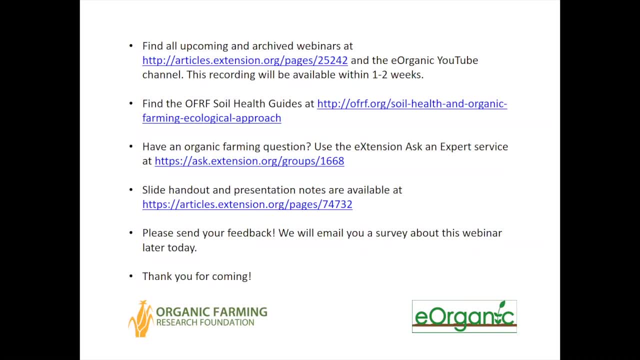 And I think it's something I need to look into. Okay, Do you have any more thoughts on involving animals with planned grazing to help manage soil health and sustainability? I think it's a very powerful tool. I am not a grazier. I've never had experience with livestock. 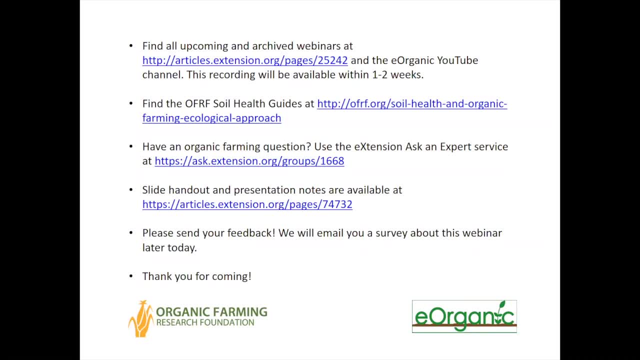 But there are plenty of success stories with management-intensive rotational grazing. I talk about this some in the new soil health guide at the Organic Farming Research Foundation website On carbon sequestration and climate mitigation. there's quite a bit of discussion there. 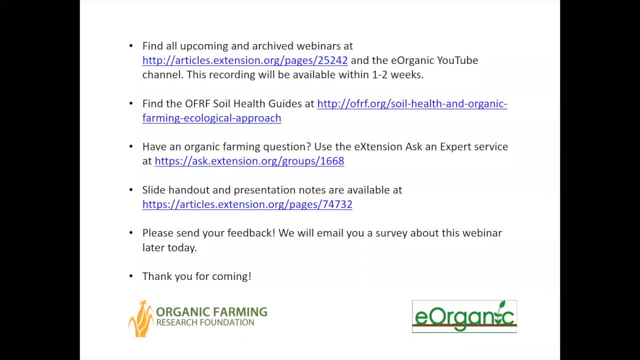 Because one of the fastest ways to build soil carbon is to put in a high-diversity perennial pasture or prairie mix and then rotational graze it. You know, really management-intensive, brief, intense grazing followed by plenty of time to recover. 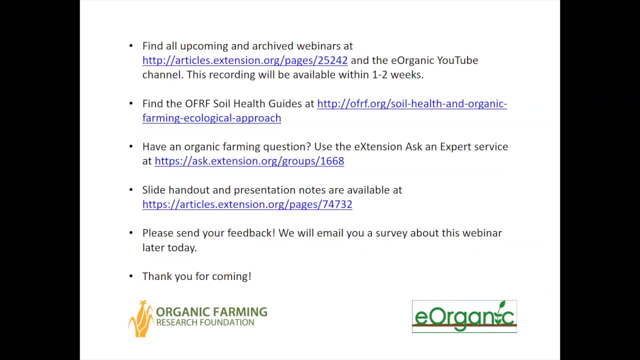 Oh yeah, Comprehensive assessment of soil health. I saw that flash up here. That is a soil health assessment tool that Cornell has developed. From what I've seen, it really is most applicable to climates fairly similar to Cornell: cold and kind of humid continental climates. 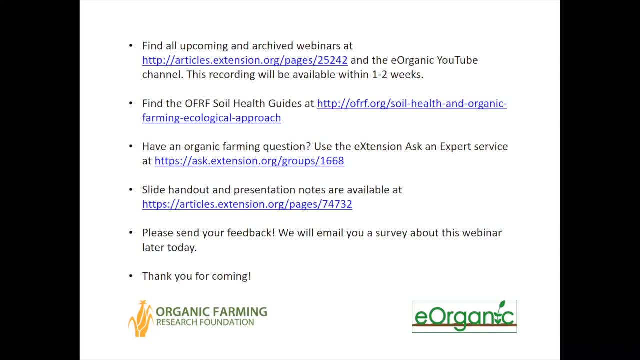 It was evaluated in the deep south. It was evaluated in the deep south. It was evaluated in the deep south. I think it was in Texas or was it North Carolina. It was found not to be that as useful in predicting soil health outcomes and soil health impacts as it is closer to its home base. 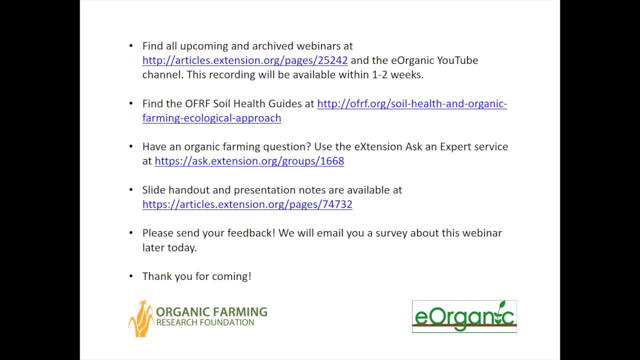 It works very well in Pennsylvania. Pennsylvania Association for Sustainable Agriculture is using it in a multi-farm project that they're evaluating improvements in soil health or levels of soil health. I think it's an excellent model And I'm wondering if perhaps, with some adaptation, a very similar approach could be taken in the Pacific Northwest and also for interior dry land regions. 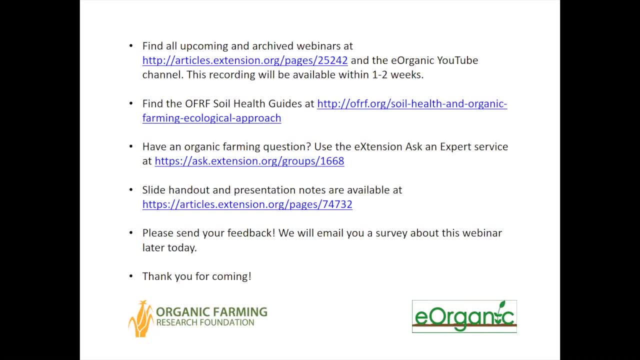 Okay, Mark mentioned that a risk management webinar which is going to be taking place soon that he's going to be presenting, And that one is coming up soon, on February 6th. So if you're interested in attending that- I think probably the evening- 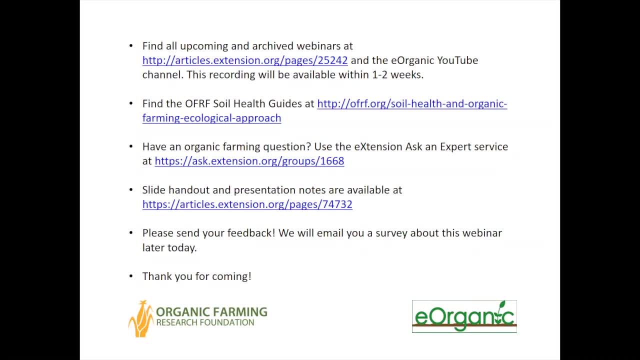 That's right. That's right. I think probably the easiest way is just to put in webinars by eOrganic into a search engine And you'll see our upcoming schedule of all the webinars that we've got planned this winter And that one is called Lower Financial Risk by Increasing Soil Health. 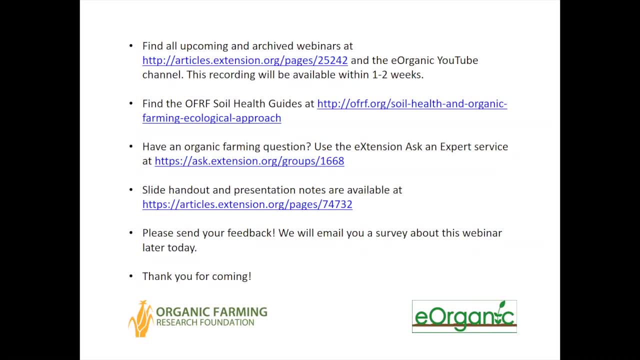 And that one takes place at the same time as this one did on February 6th, And we've got quite a few other webinars on soil health, as well as many other organic farming and research topics coming up this season, So I hope you can all join us for those. 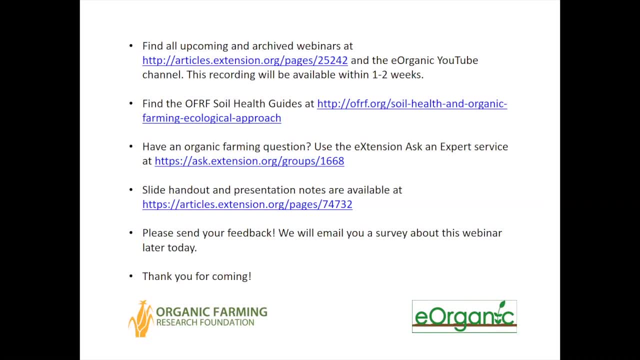 So it looks like we have pretty much covered the questions here, So I'd like to thank everyone for all their great questions. So thank you again, Mark and Dawn, who's been online, for joining us, And we hope you can all join us for the many other webinars this coming season. 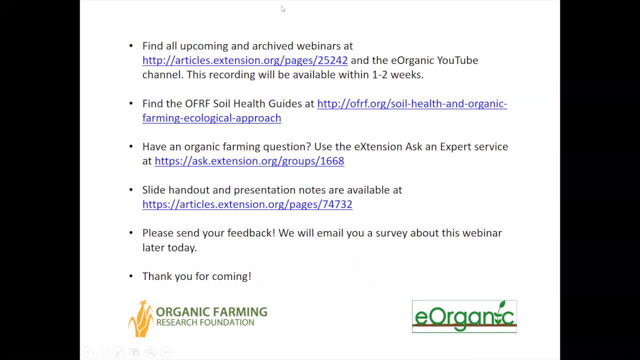 So thanks everyone. Okay, Thank you.